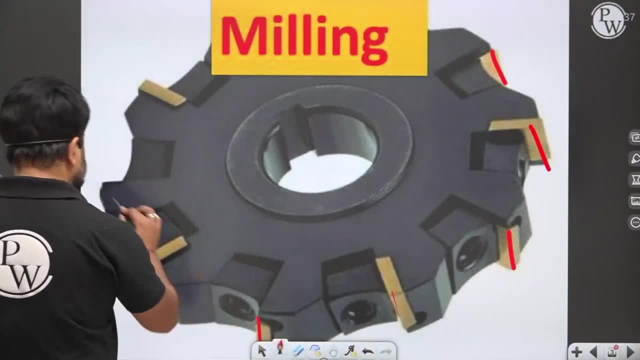 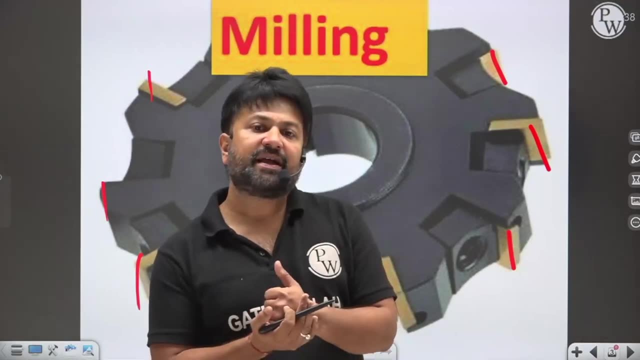 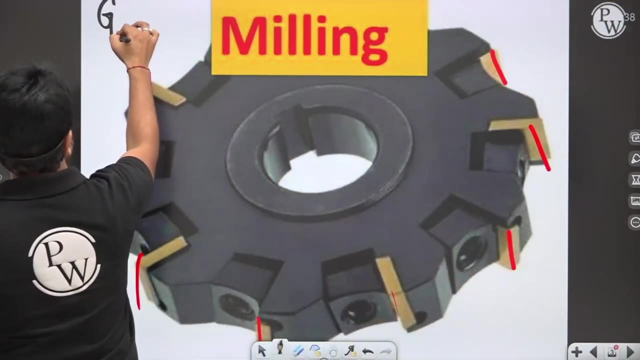 is a multi-point cutting tool. See here: this is a multi-point cutting tool, My dear. I am going to discuss the silent feature of the milling cutter. Basically, milling cutter is going to produce grooves and flutes. Milling cutter is going to produce grooves and flutes. 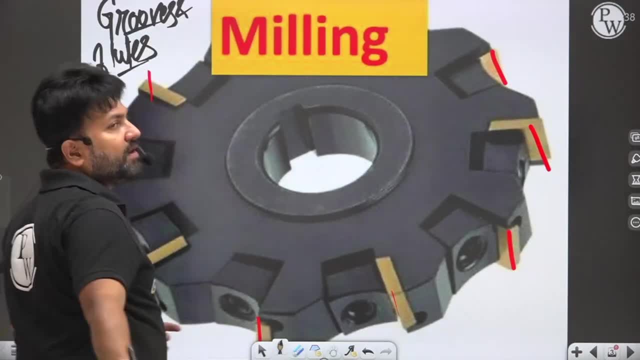 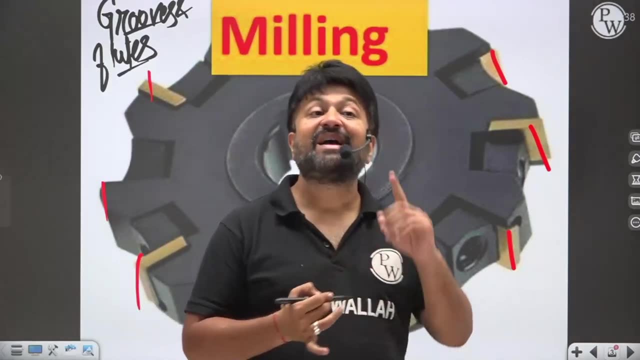 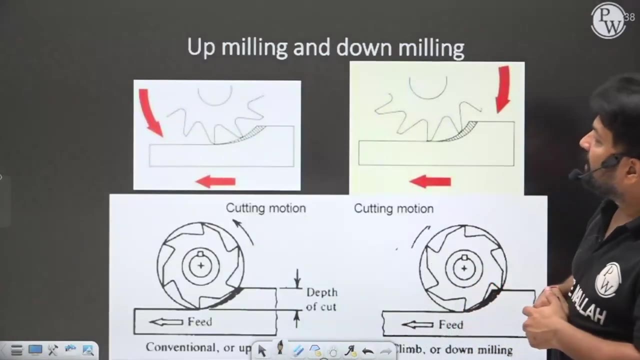 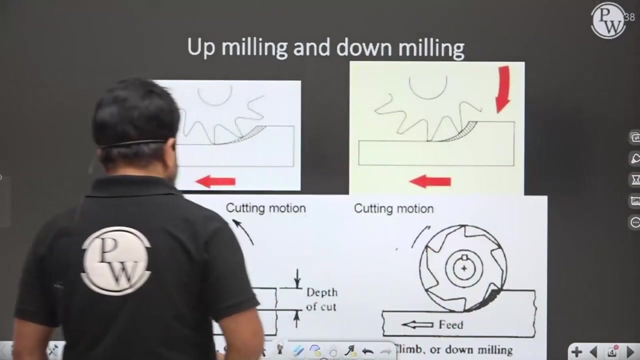 grooves and flutes in various tools like drill tapes, reamers, hops and gear shaping cutter Right and gear shaping cutter Milling are basically are of two type. That is, that is the one, is that is your conventional milling. This is what This is: conventional milling. I will show. 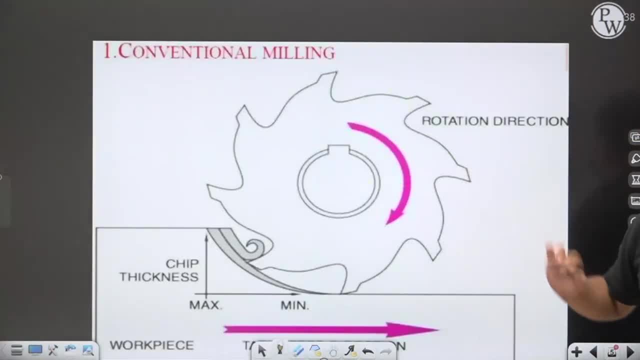 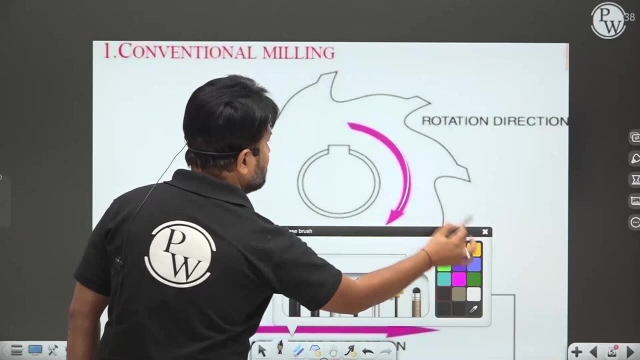 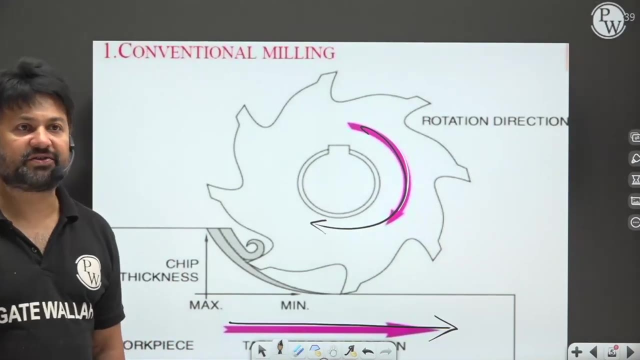 you. I will show you in the another figure. See, this is the conventional milling. In a conventional milling, the direction of your milling cutter, the direction of your milling cutter and the direction of your table are in what Are in opposite direction. Okay, are in opposite direction And in: 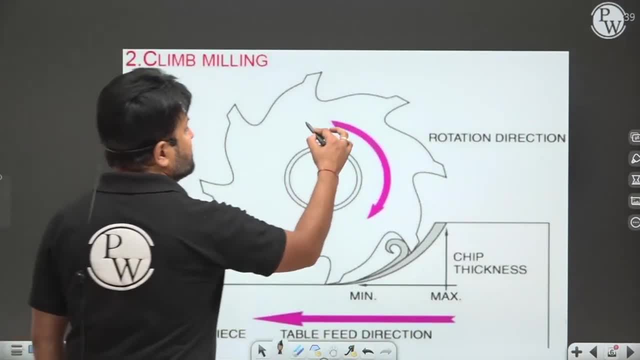 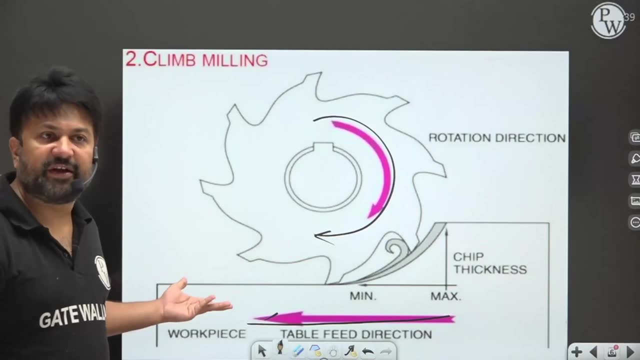 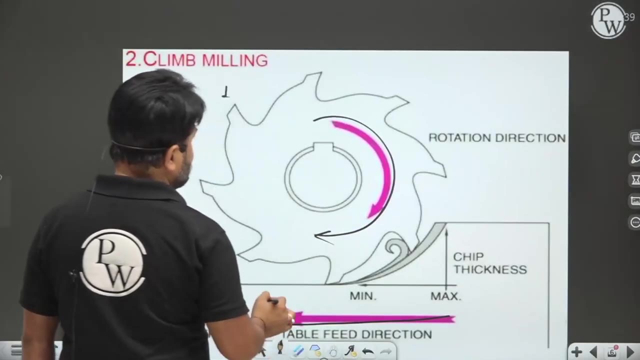 the peri in the climb. milling the direction of the milling cutter? okay, and the table speed or the workpiece speed or workpiece feed direction is the same. My dear, this is the milling cutter Right, This is what. This is the milling cutter, This is the milling cutter. teeth One, two, three. 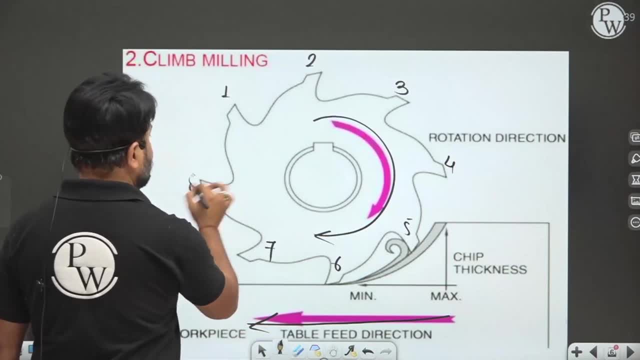 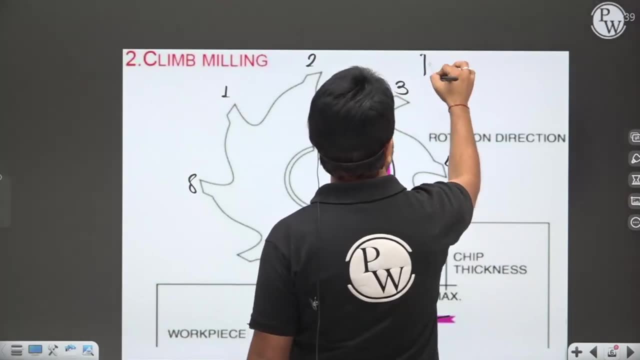 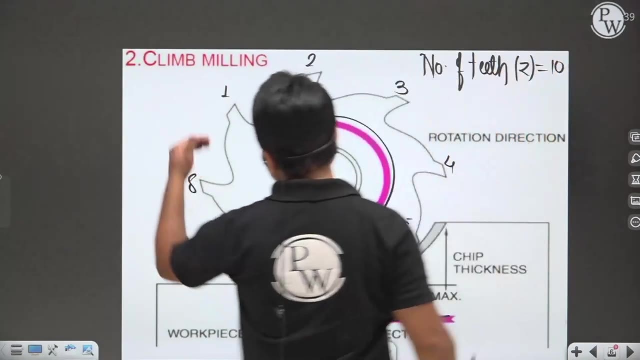 four, five, six, seven, eight. Let's say I am going to take the number of number of teeth. I am going to take number of teeth, number of teeth of the milling cutter. Let's say Z, I am going to take 10.. Here it. 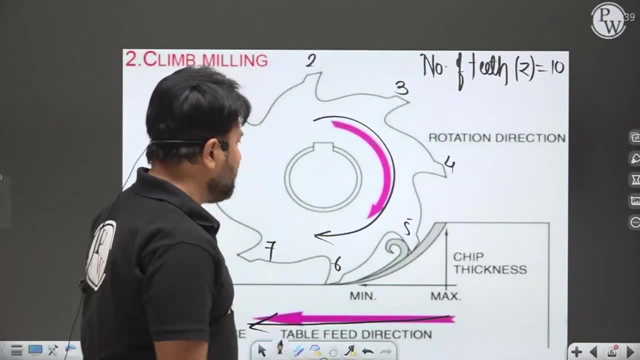 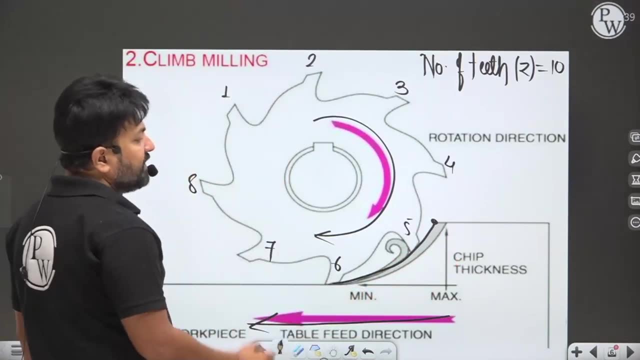 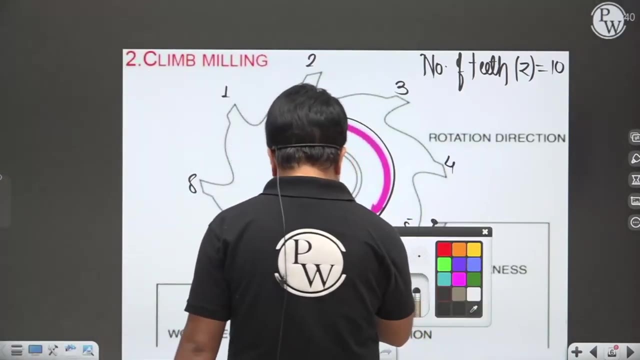 is 8, but I am going to round off, let's say 10.. Here you can see, when the milling cutter comes in contact with the work piece, The work piece will move along with the milling cutter. milling cutter teeth: that is feed per tooth. that is feed per tooth. that is known as what feed per tooth? fz. 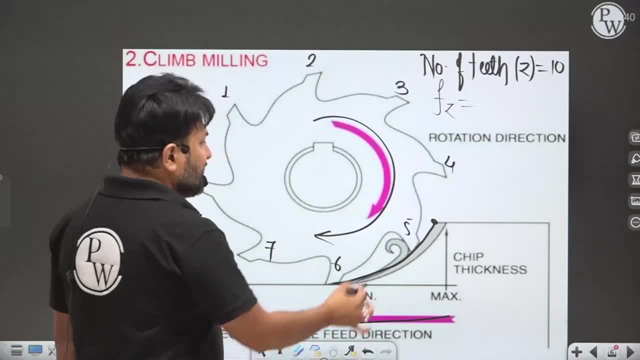 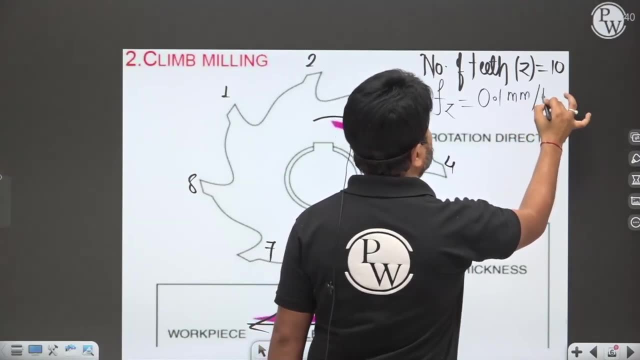 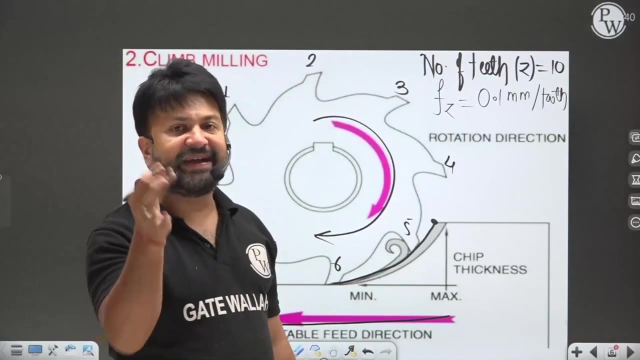 right, fz, that is feed per tooth. let's say one teeth of the milling cutter moves along the table. okay, 0.1 mm per tooth. 0.1 mm per tooth, and how many teeths are there? 10 means in one revolution 10 teeth. when 10 teeth comes in a contact with the workpiece, then the table will. 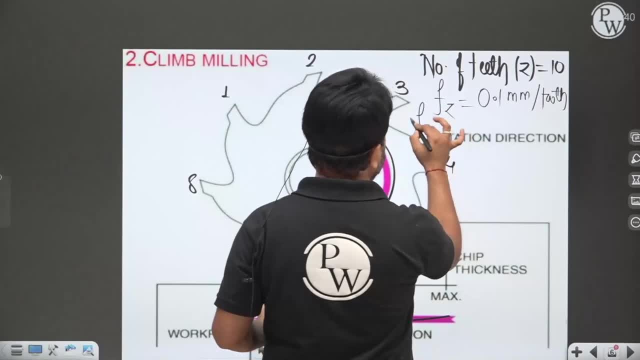 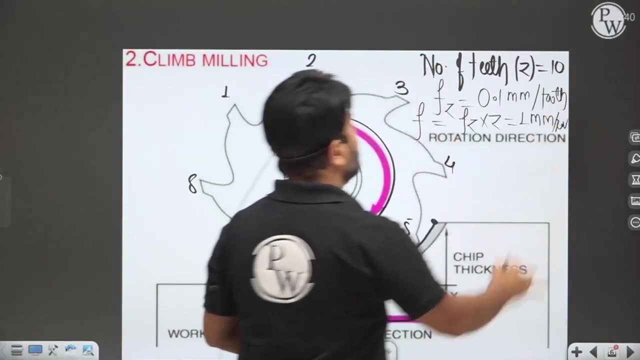 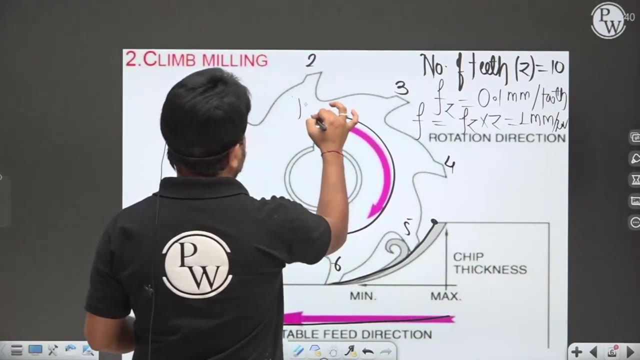 move up to a certain value, that is what feed, that is fz into z, it will come what? 1 mm per revolution. 1 mm per revolution, right? that is 1 mm per revolution, right? suppose that if you know the rpm, that is revolution per minute. if you know the rpm, can you find out the table speed? yes, you. 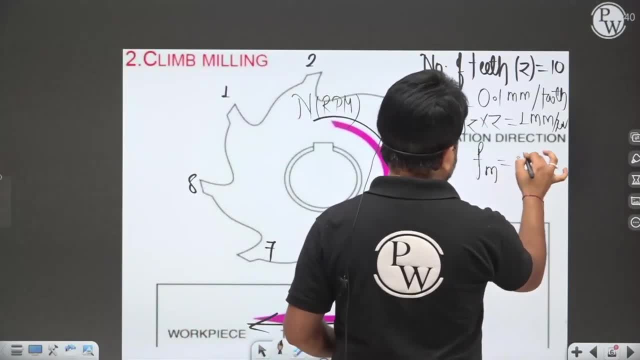 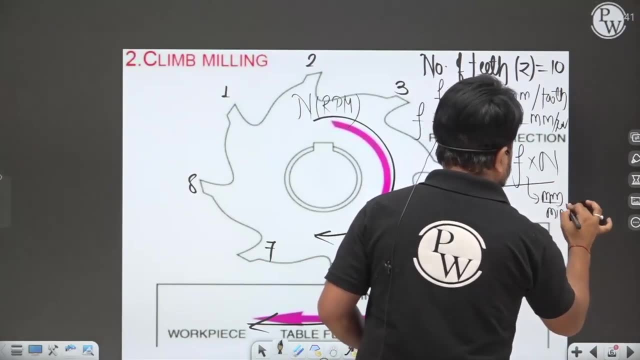 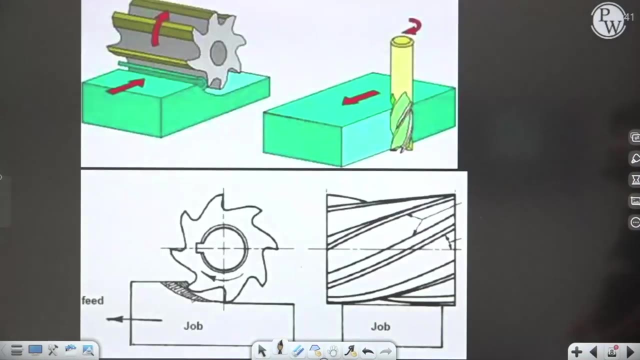 can find out the table speed. that table speed equal to what? f into n? that is the table speed. that will be in mm per minute. my dear, that will be in mm per minute. clear, that will be in mm per minute. now, this is the same thing which i have discussed, my dear uh, milling operation. 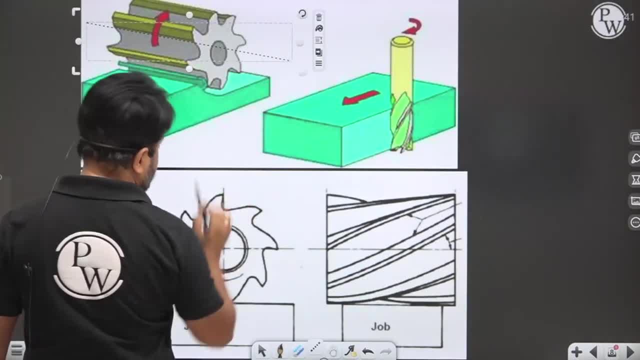 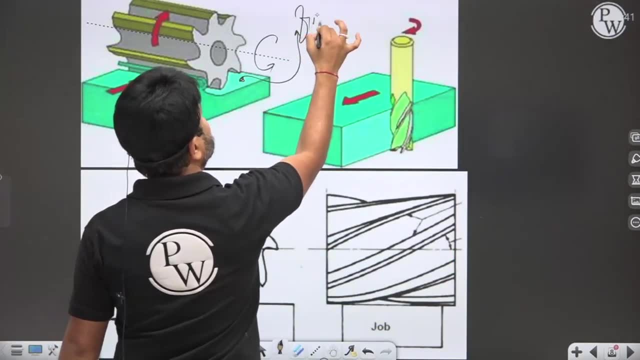 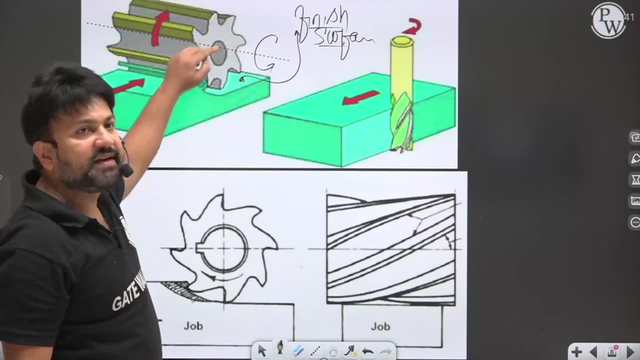 are of various kind. this is a peripheral milling. here you can see the axis of rotation. here you can see, this is the axis of rotation and this is what a finished surface. this is what a finished surface, right, this is what a finished surface. here the axis of rotation is parallel to finished. 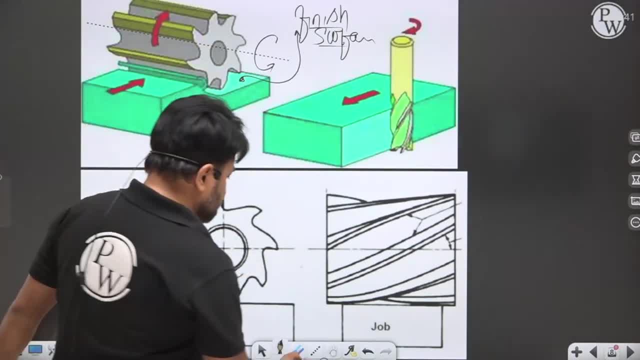 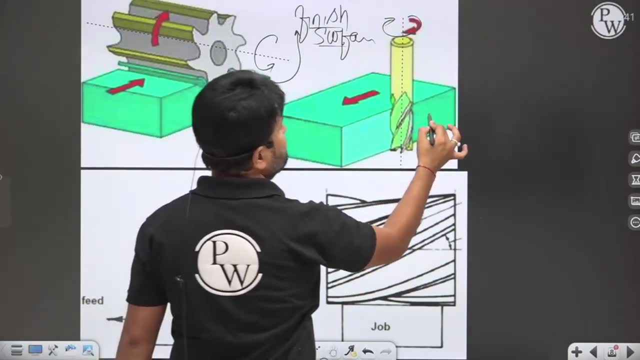 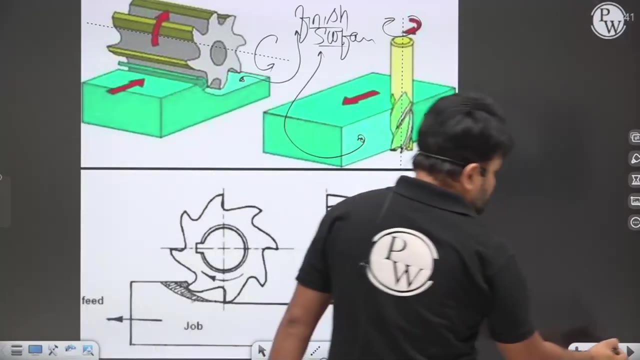 surface. that's why it is known as peripheral milling. here you can see, this is axis of rotation. right, this is the axis of rotation. this axis of rotation is parallel to what is parallel to, again, your finished surface. that's why, again, it is a peripheral milling. my dear, there is a face. 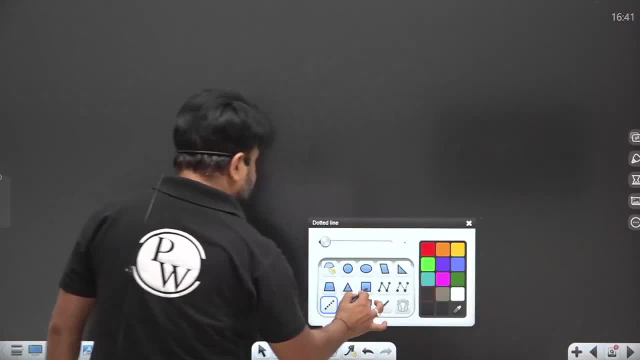 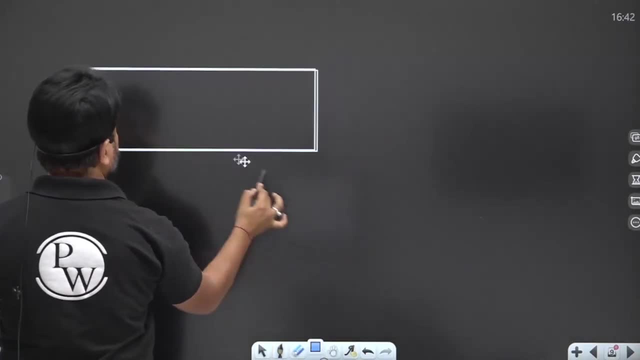 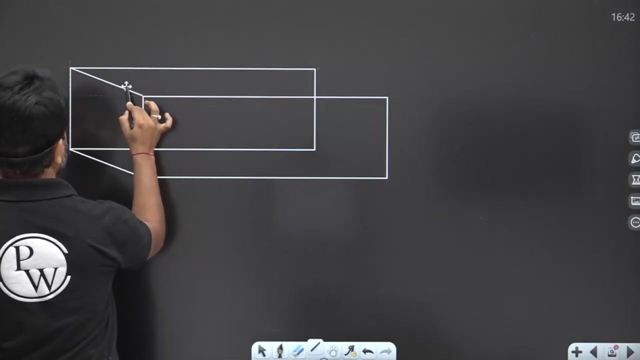 milling. also. let me show you the face milling a. face milling a will be look like this. Our face milling will be look like this: This is your workpiece. This is your workpiece. This is your workpiece here. This is your workpiece. 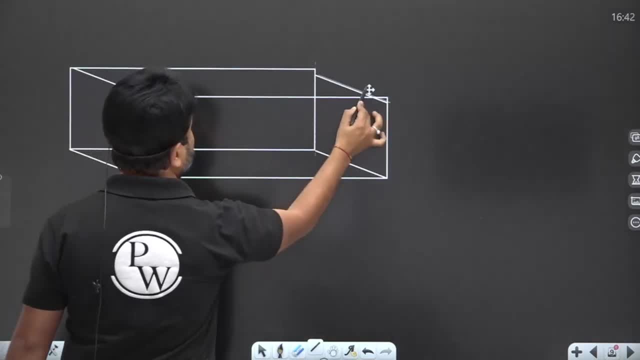 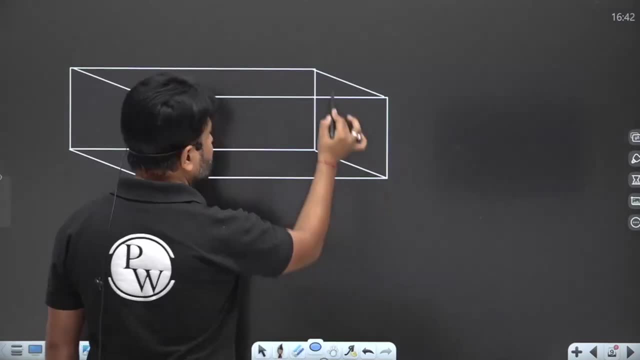 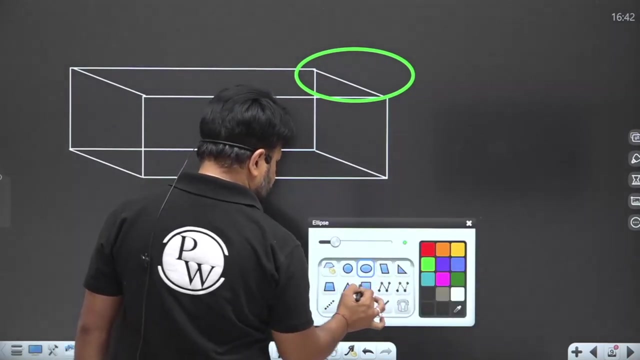 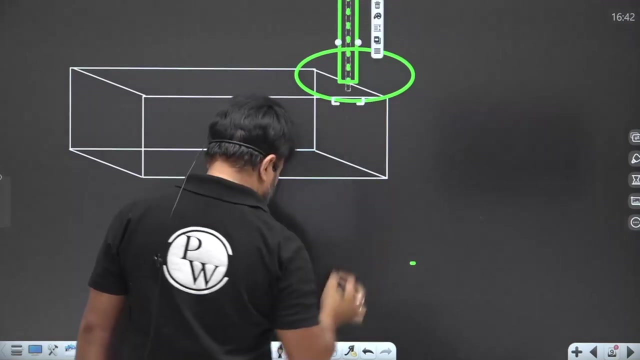 This is your workpiece. This is your workpiece And my dear. here I am going to draw a milling cutter, the milling cutter Here, the milling cutter teeth, here the milling cutter teeth. this is a milling cutter and this is an arbor about which the milling is going to be what Rotate, About which the 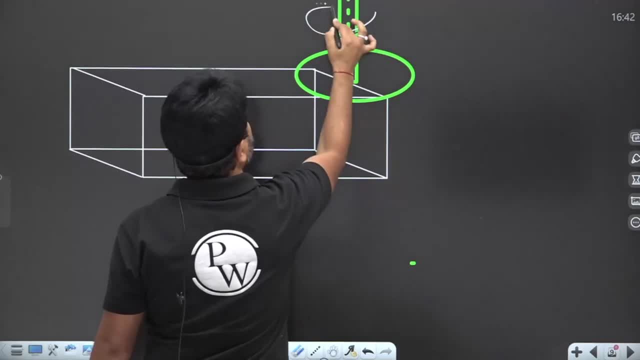 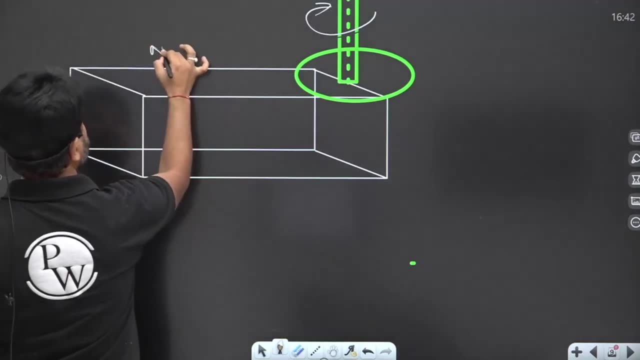 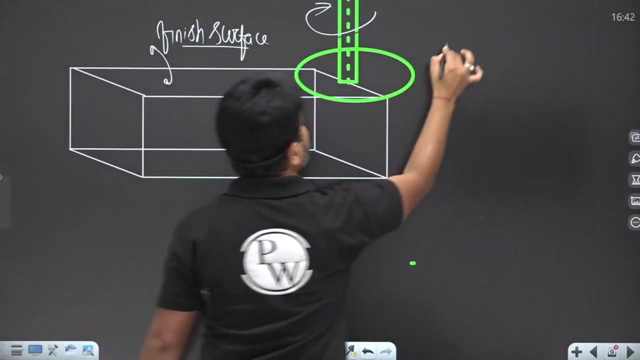 milling is going to. what About which? the milling is going to be what Rotate? right, It is going to be what Rotate. Now you can see the axis of rotation is perpendicular to what? The finish surface, the finish surface, right finish surface. so that is known as what face milling, that is. 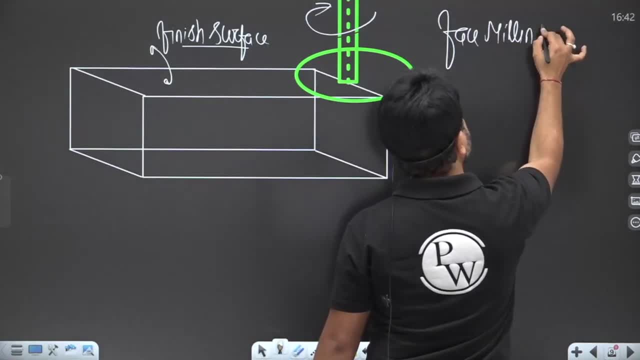 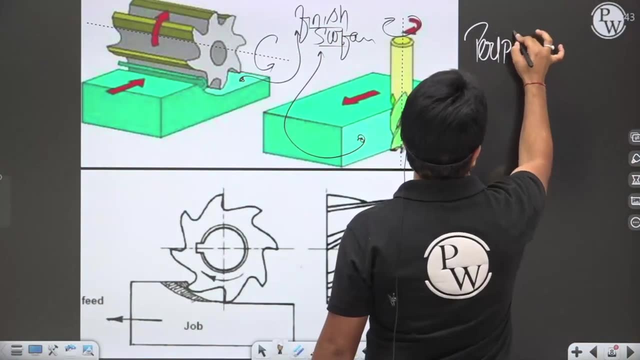 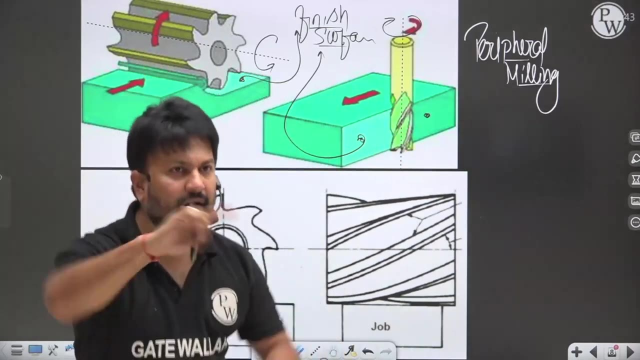 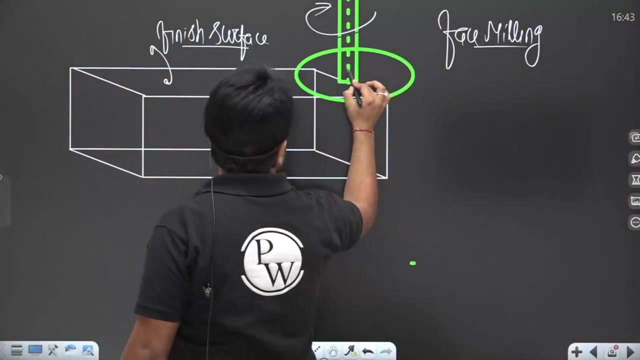 known as face milling right. that is known as what face milling right here? this is known as what? peripheral, peripheral, peripheral milling operation. that is known as my dear peripheral milling operation right peripheral milling operation. phase milling operation is clear when the axis of rotation is perpendicular to the, to the finished surface. that is known as what phase. 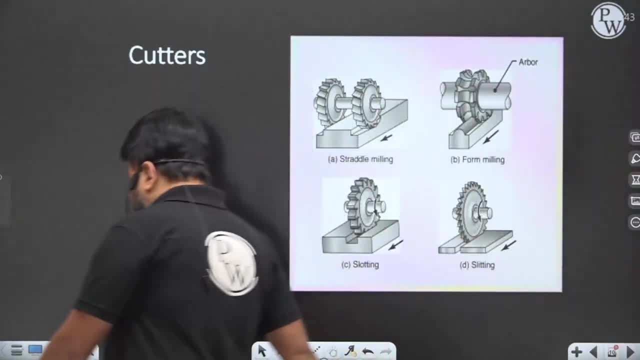 milling. now, there are various type of milling operation, my dear. there are various type of milling operation. one by one, i am going to discuss these type of milling operation. right? so the first milling operation which you are going to see is known as what straddle is known. 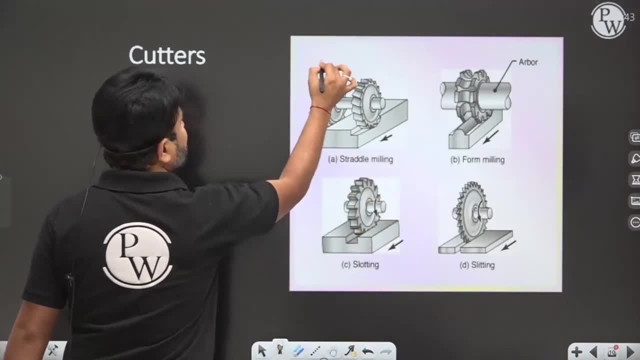 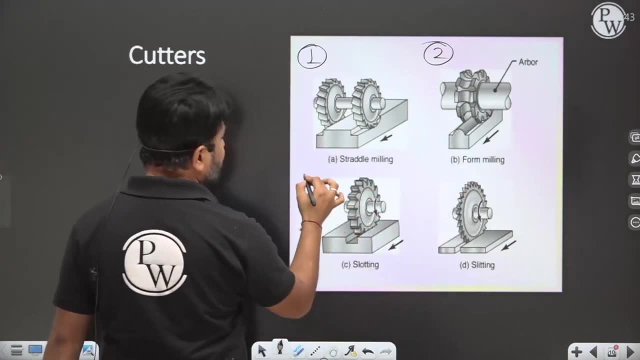 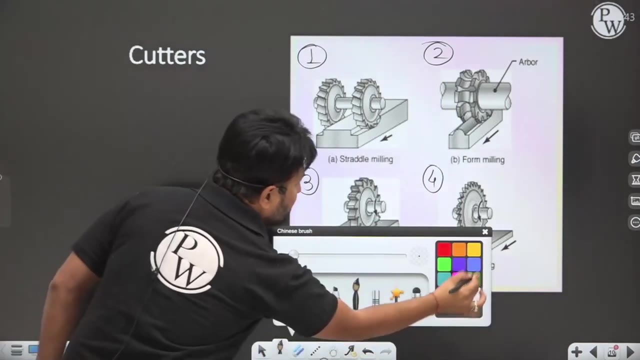 is known as what straddle. this is what this is. let's say first, this is. let's say first, that is straddle. it is what as form milling. this is known as third, that is slotting. this is known as fourth, that is what slitting. so, my dear, here, the straddle milling. here you can see a straddle. 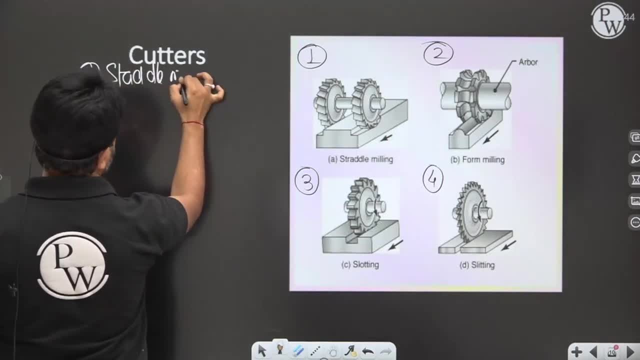 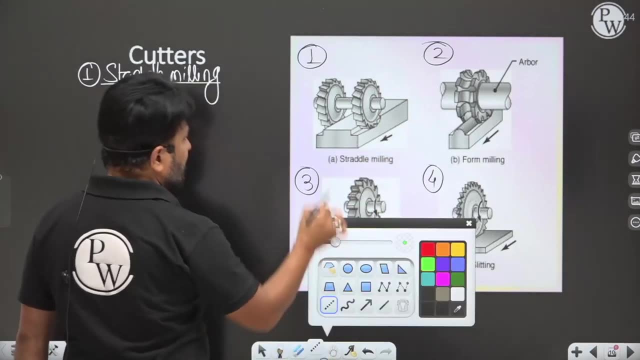 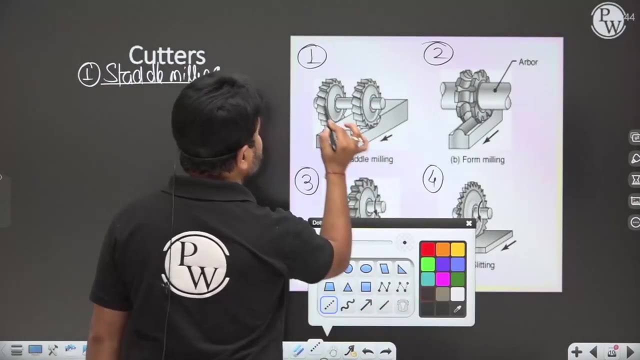 a straddle milling, a straddle milling, my dear in a straddle milling, a straddle milling. This is basically an arbor. Arbor is basically a shaft about which you can mount a milling cutter. So this is the axis of rotation right. 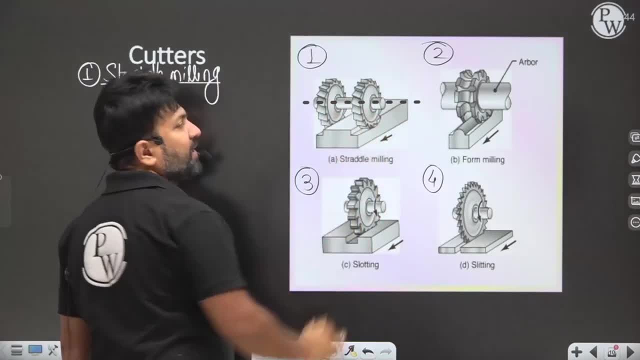 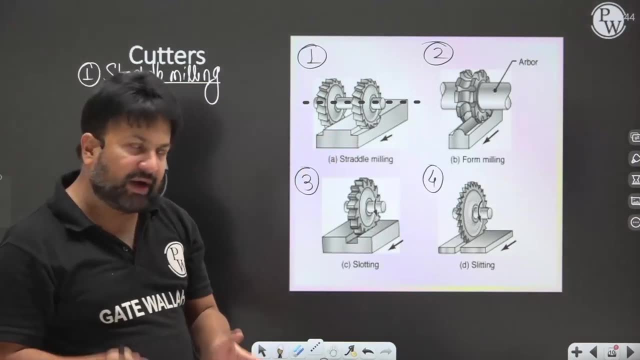 And this is the arbor you can see. And on the arbor we are going to mount two milling cutter which has some separation. In a gap the machining is not going to happen, But where the milling cutter is present, the machining is going to happen. there, right? 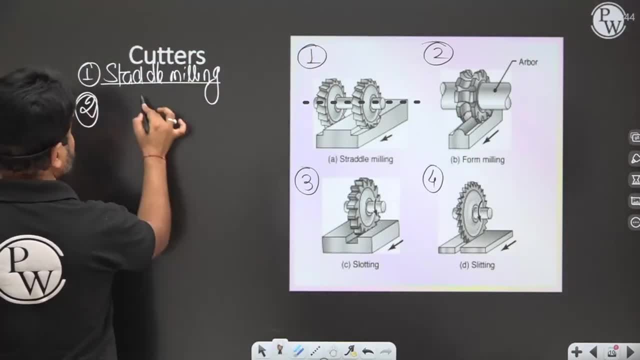 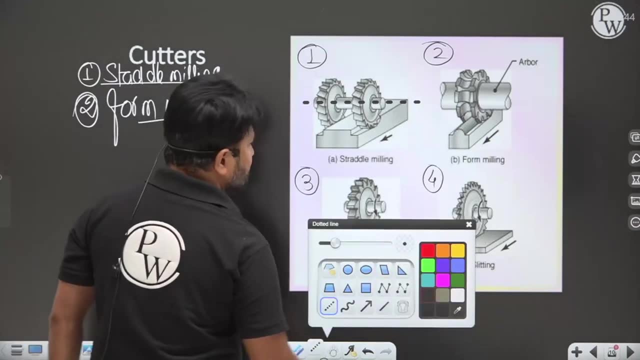 Like now. the second is what? The second is form milling. Form milling, My dear, form milling, My dear form milling. What is a form milling, My dear? you can see in the form milling. this is again the axis of rotation, that is. 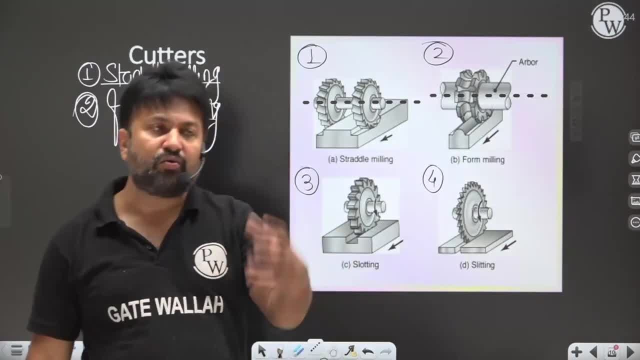 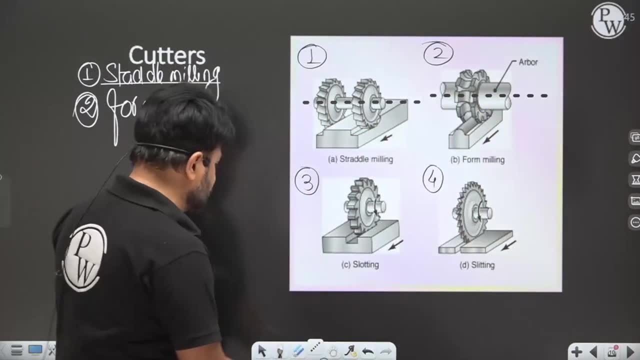 an arbor On arbor, we are going to mount a tool, a mount, a milling cutter, by which, when you do a cutting, the shape of the milling cutter is going to produce on the workpiece. that is known as what Form tool and form milling cutter. 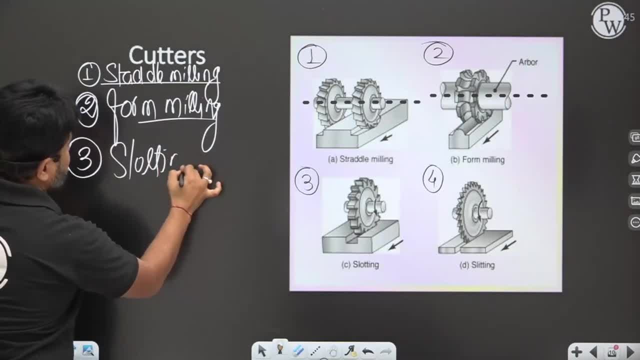 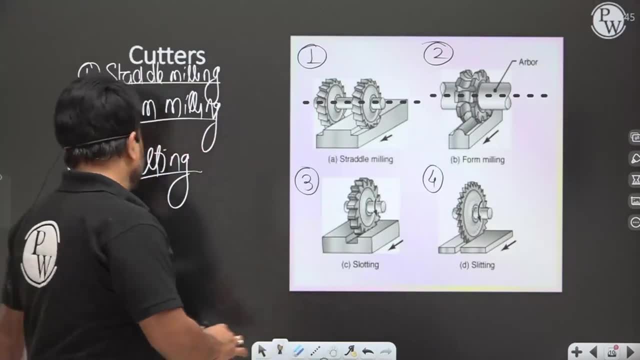 The third is your saw Slotting. The third is your slotting. By using this milling cutter, we are going to produce a slot in a particular workpiece right. And the fourth is- and the fourth is what The slitting? 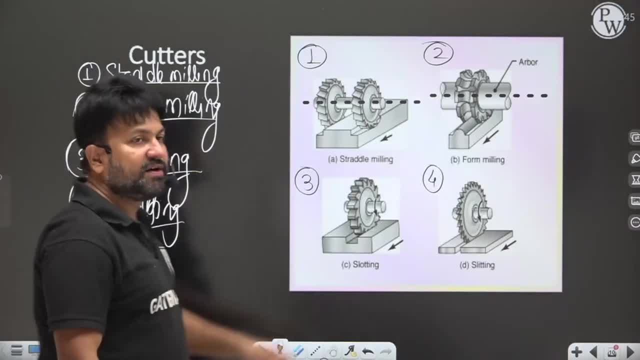 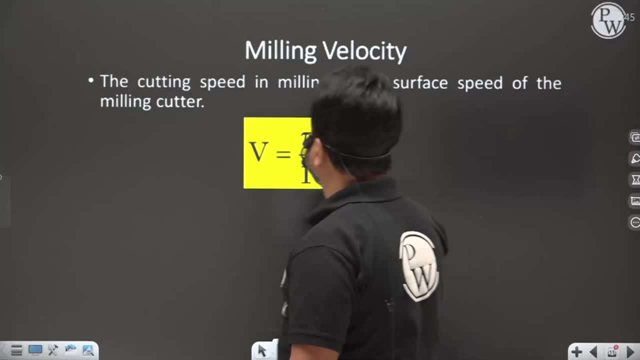 My dear, by using the slitting type of milling cutter, you are going to separate out, you are going to cut out a plate or sheet. You are going to cut out or separate out a sheet. Now let's discuss about the milling cutter velocity. 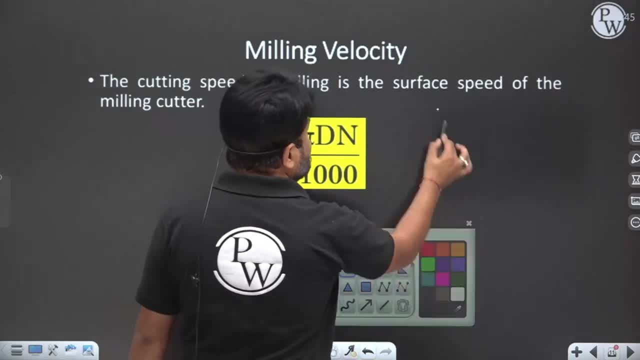 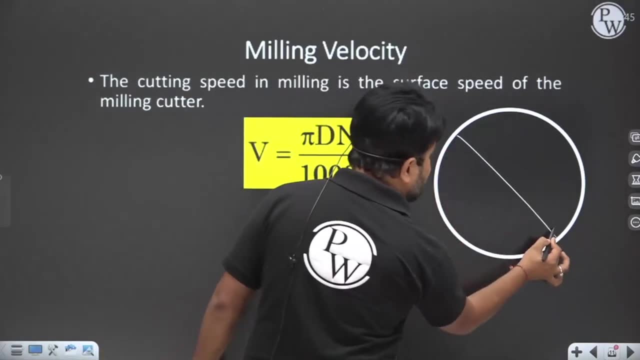 My dear, let me discuss about the velocity of the milling cutter. Suppose that, Suppose that this is the suppose that this is a milling cutter having a diameter, having a diameter, having a diameter D, and it is rotating about with the RPM N, then what will? 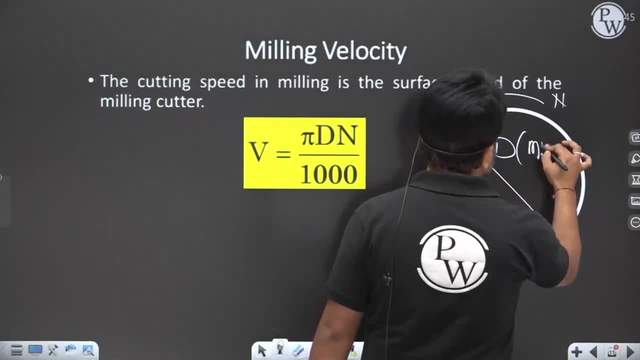 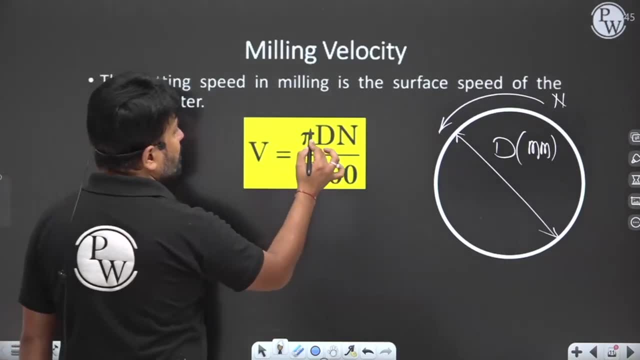 be the cutting velocity. diameter with a, with a diameter in the MM, diameter in the MM, So cutting velocity equal to what Pi D N divided by 1000.. If D is in the MM, then you can get the cutting velocity right. 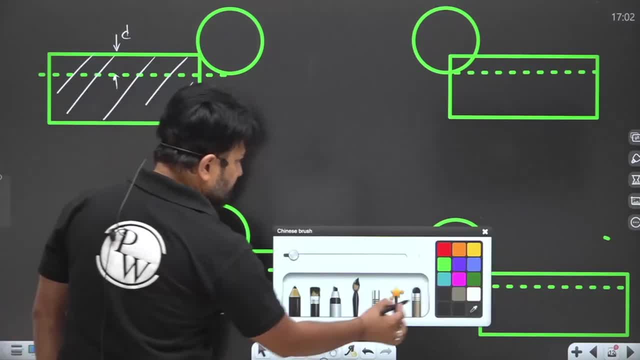 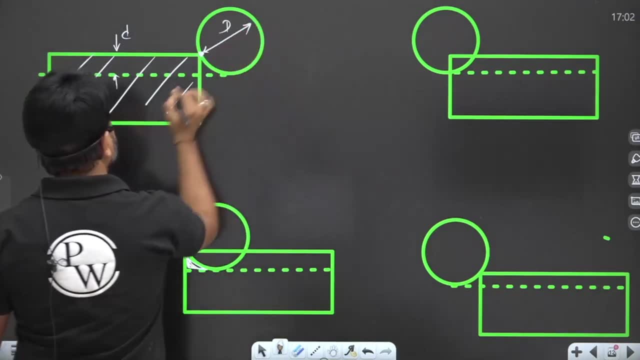 Yes, So initially. So initially, the milling cutter is here. okay, The milling cutter is here, having a diameter D, right, And this is the length of the workpiece which is going to what Machine, right? 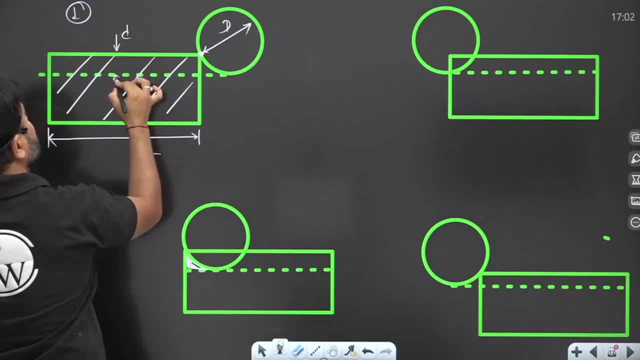 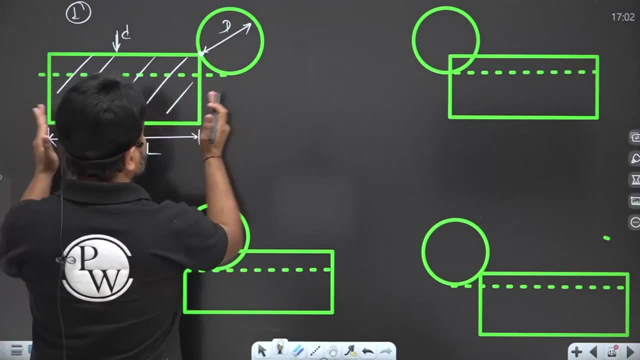 This is a position one, and that much depth I have to cut. What That much depth I have to cut? This is the entire workpiece. When the table moves from here to here, it is going to cover a entire length L, But still you can see. 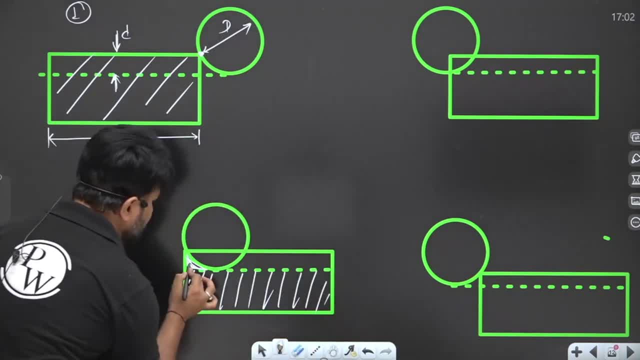 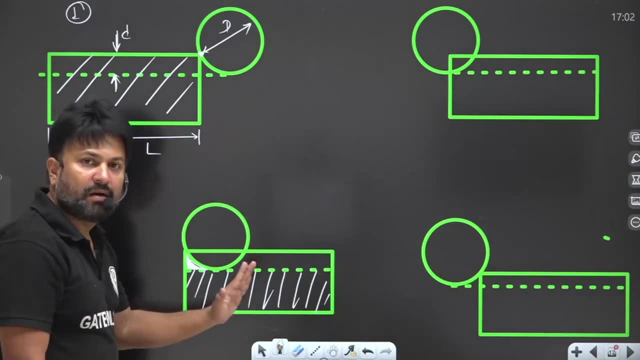 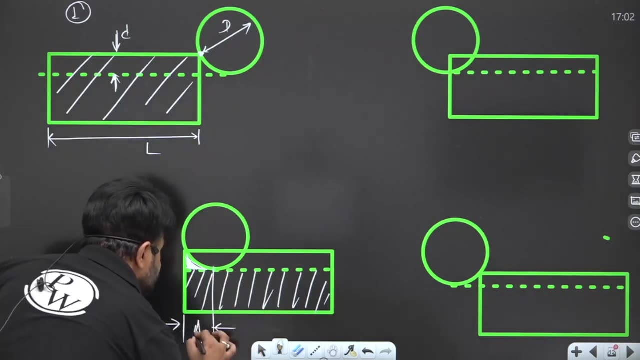 Still. you can see, this is the remaining material and this is the remaining material which is not cut yet. Here the table move by length, L right. So this is the remaining material which has to be cut. Let's say, this is the approach distance by which a milling cutter has to move. 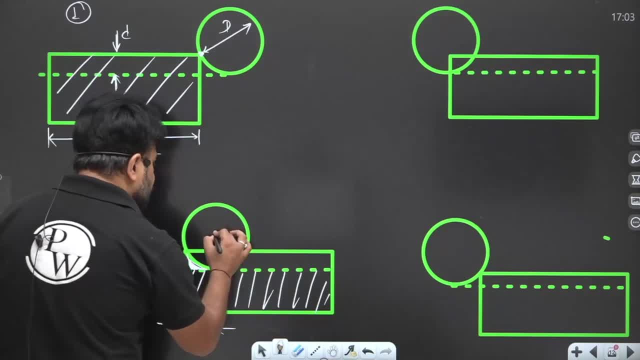 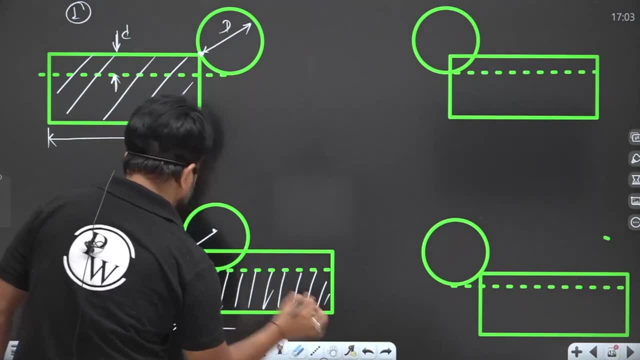 So that the entire workpiece is going to be what Machine? right, The entire workpiece is going to be what Machine? This is what D by 2.. This is what D by 2.. D by 2, right. 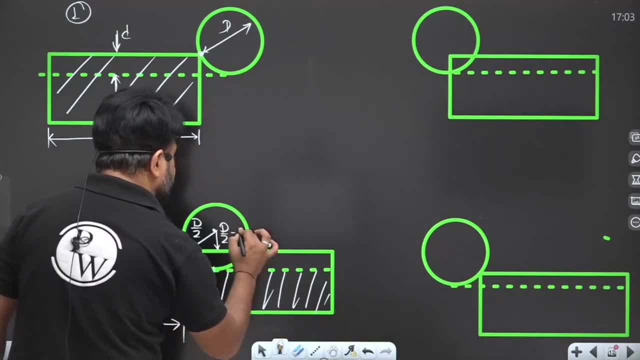 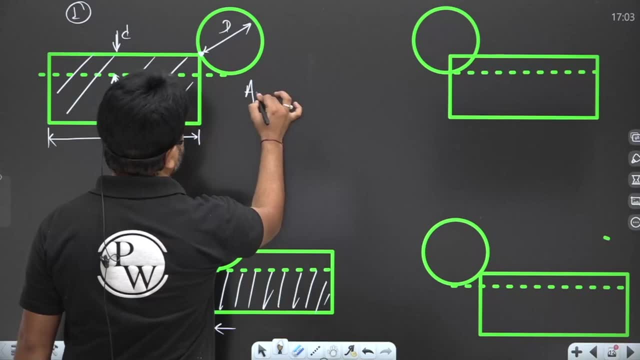 And this is what This is: D by 2 minus depth of cut. So we can calculate this much A, How much this A. This A is very simple. This A is that is what D by 2, right. 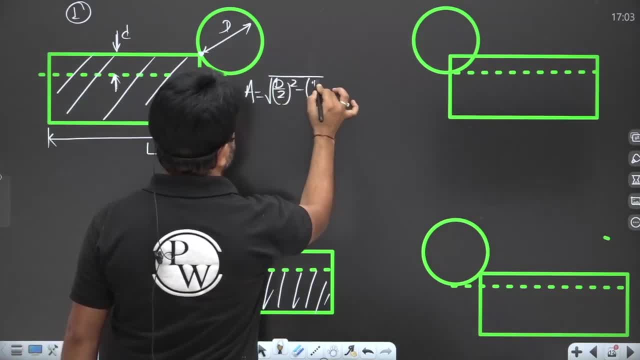 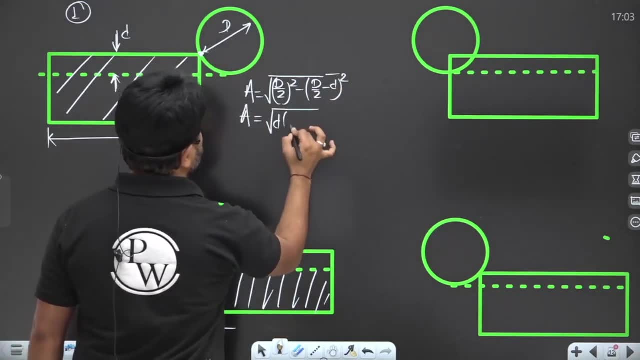 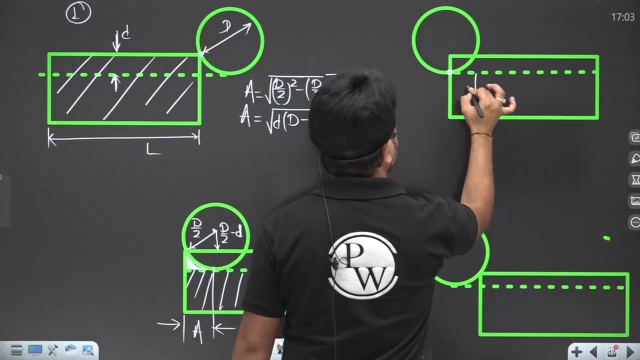 D by 2 whole square minus D by 2 minus of small d whole square. It comes about, it comes out, my dear, That is root of small d capital D minus small d. Now, here the milling cutter will reach here by, by, by, travelling that much distance A. 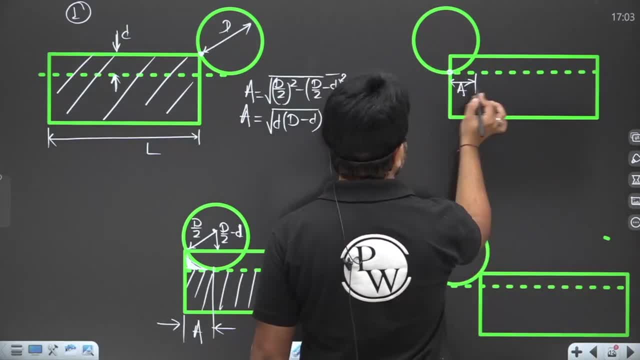 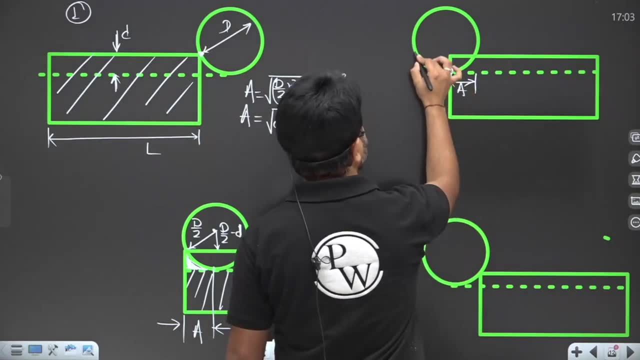 So the total length, the total length travelled by the table is what. The total length travelled by the table is what. That is okay, that much. I am talking about that A. So this is A and this is what. 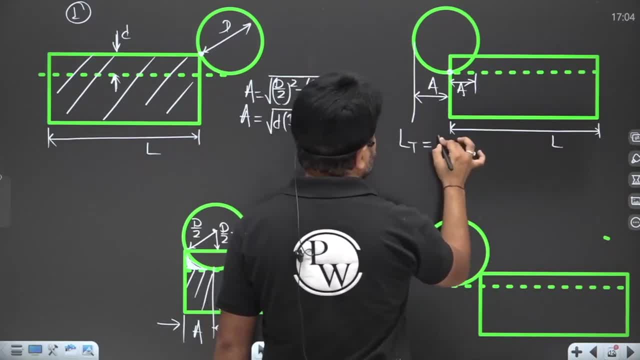 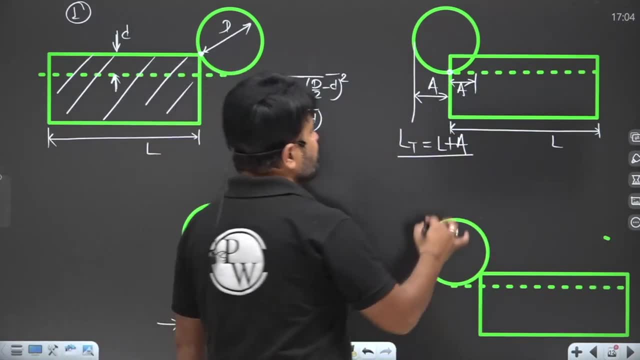 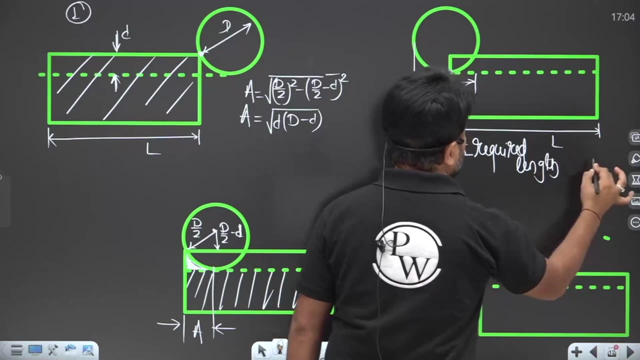 This is L, So this is the total, Total length which is moved by the table. My dear, this is the essential length, This is the required length, This is what A required length, This is what A required length which is required to machine a workpiece. 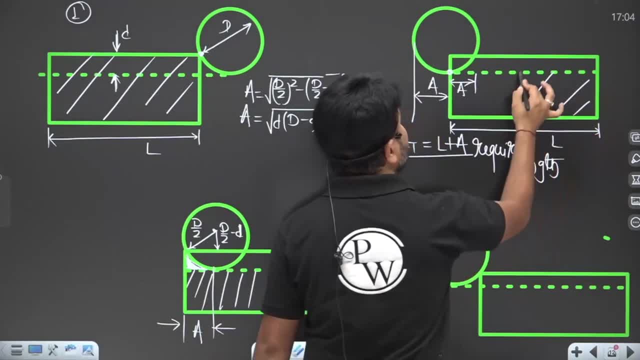 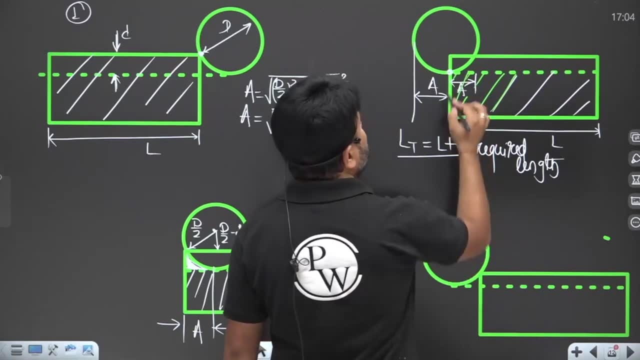 But still the milling cutter. here the machining is completed, Here the machining is completed, my dear. Here the machining is completed, But still the milling cutter is touching the workpiece. So we have, So we have to move the milling cutter. 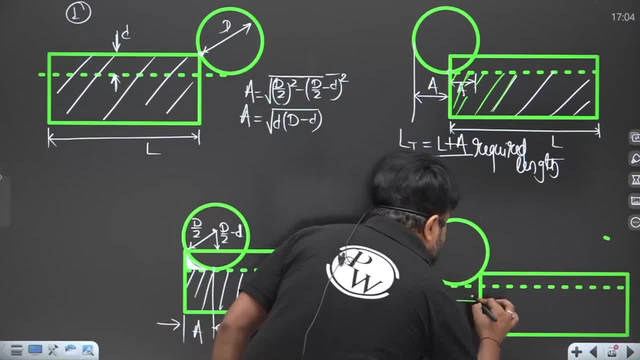 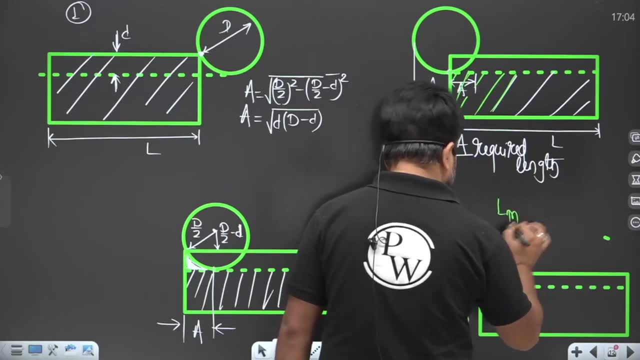 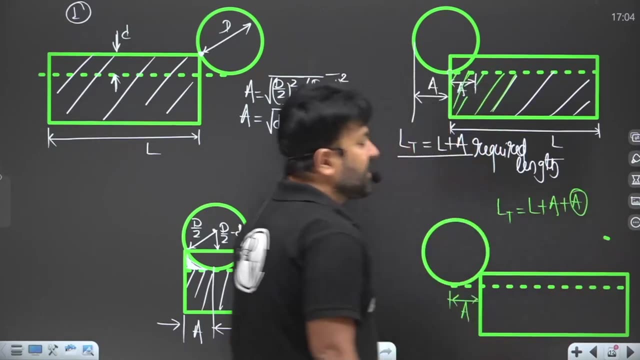 That is the over travel, My dear. if the over travel is not given to you, then move the milling cutter by same distance: A, So the total machining length. So the total machining length will be L plus A plus A. That is the over travel distance. 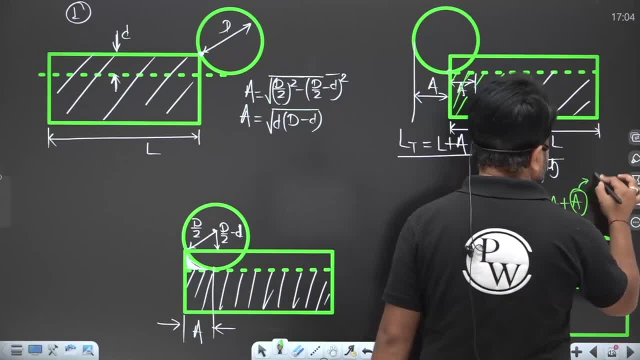 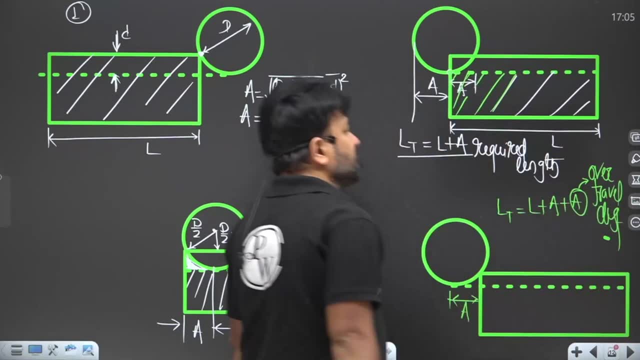 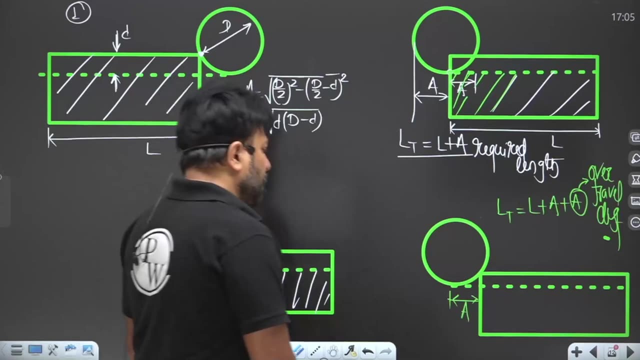 If it is not given, then take a same A. That is what, Over travel distance, Right over travel Distance, Or, or, or, yes, over travel distance, Or clearance distance Right Now, what will be the machining time then? 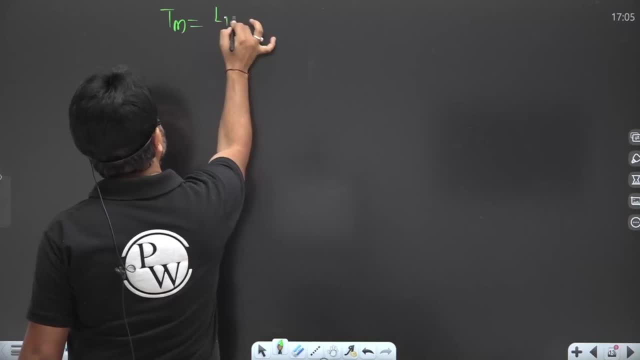 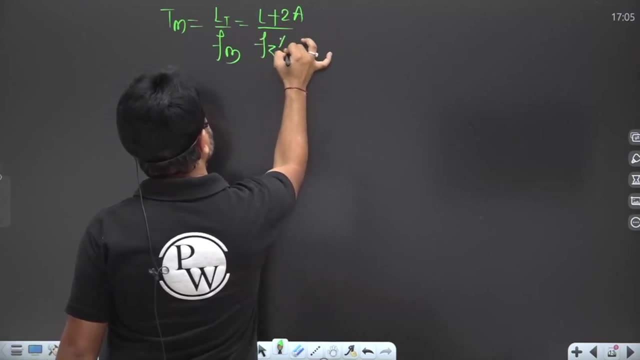 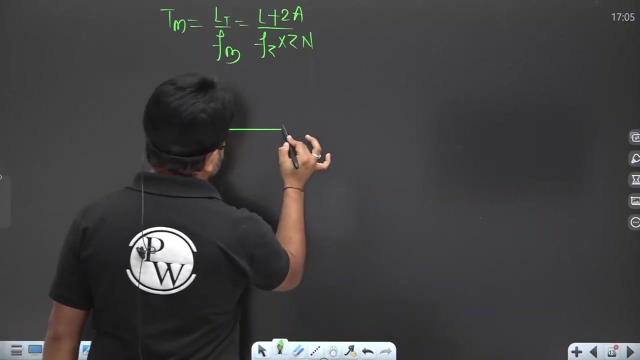 Then the machining time will be: that is L, T divided by F, M, L, T, that is L plus 2 A divided by, that is F Z into Z, into N. Right Now let me discuss you about the uncut chip thickness in the milling. 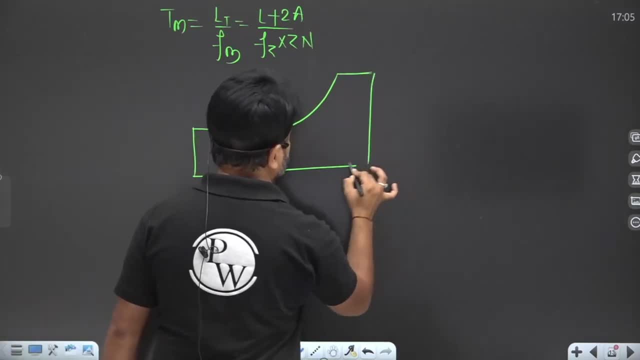 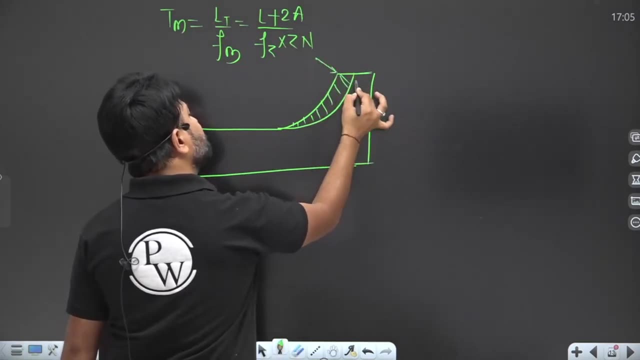 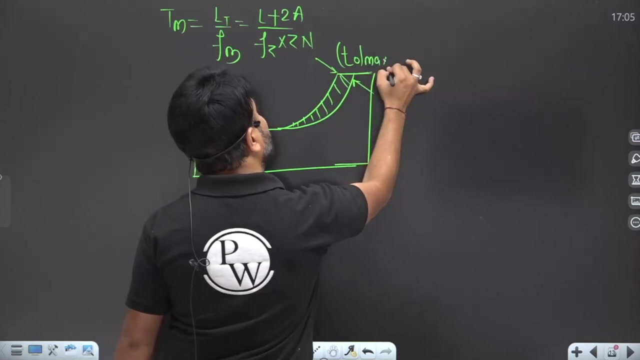 Right. Uncut chip thickness in milling. Okay, My dear, in milling operation there will be a maximum uncut chip thickness at the one end, That is T naught max, And the value of maximum uncut chip thickness is twice of F Z root of small d by capital D. 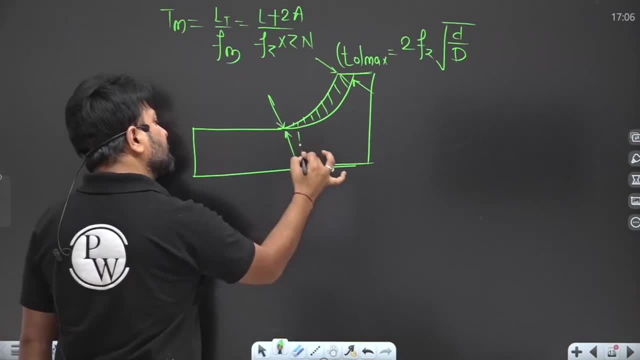 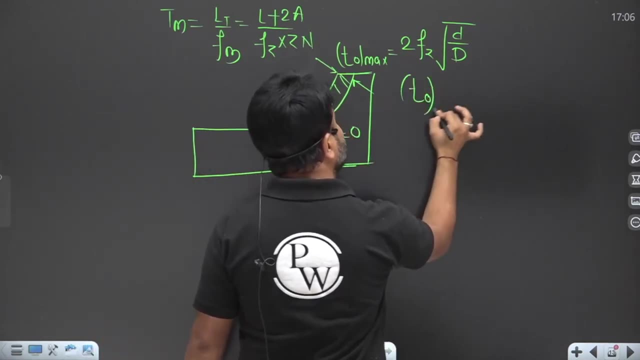 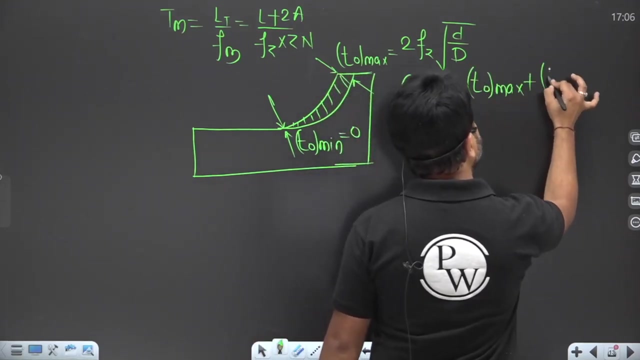 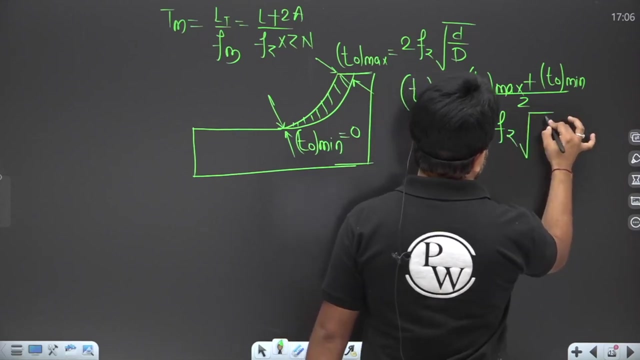 The minimum uncut chip thickness. The minimum Uncut chip thickness is zero, So the average uncut chip thickness is what T naught max. T naught max, T naught min Divide by 2.. It comes about F Z root of small d by capital, D in mm. 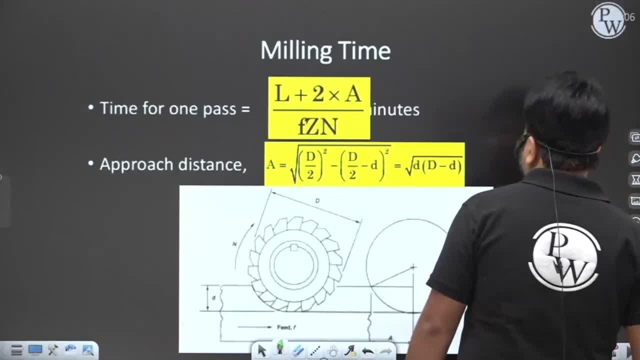 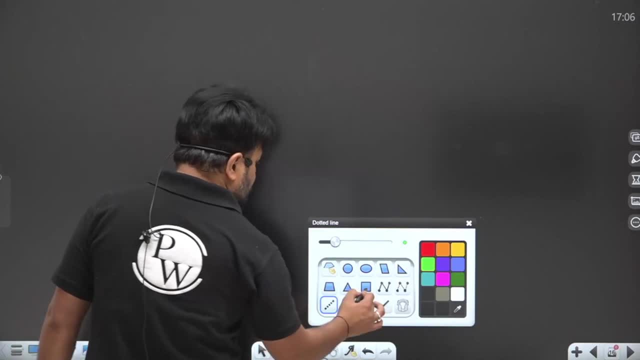 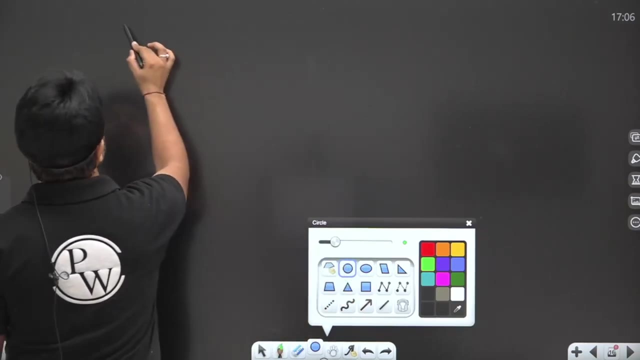 Right. So remember this thing. Now let us discuss about the facing time, Let us discuss about the machining time. in what? In the in the face milling operation, My dear, that is your, that is your milling cutter, Right. 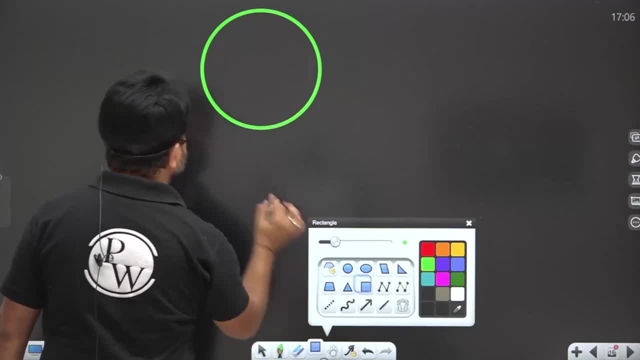 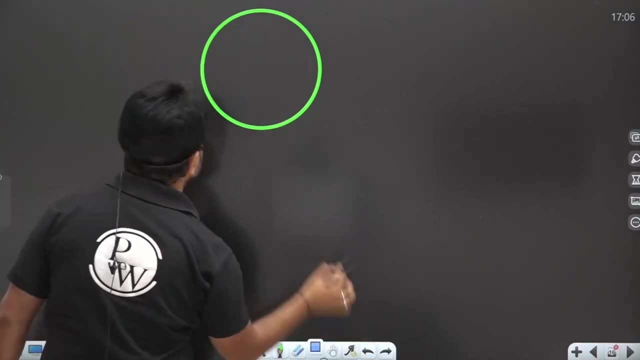 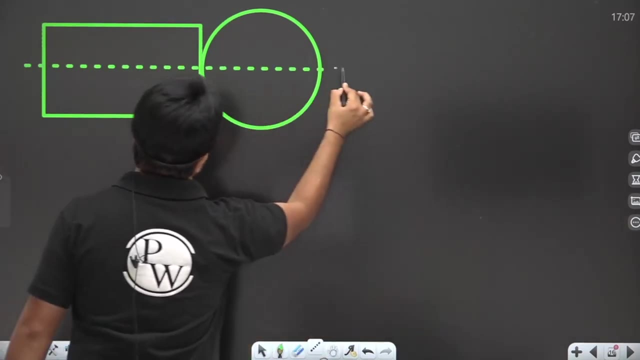 That is your milling cutter. Okay, Now, this is my workpiece. This is my. here you can see, this is my. okay, this is my workpiece. okay, which is going to be mill Now. here you can see the width of the workpiece. 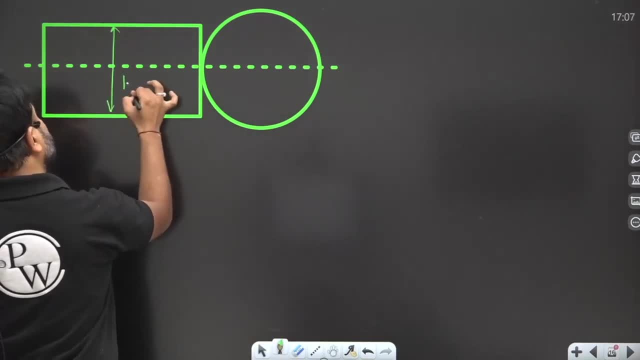 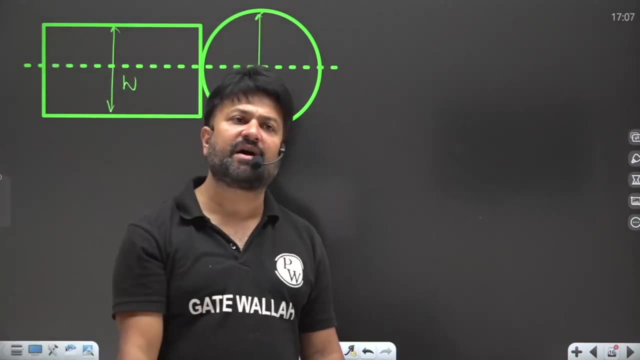 Here you can see. that is the width of the workpiece. okay, is smaller than the diameter of what Milling cutter. So in one pass we are going to machine the workpiece and the length of the workpiece. 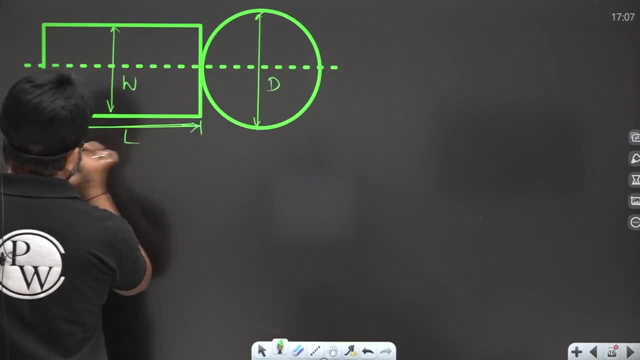 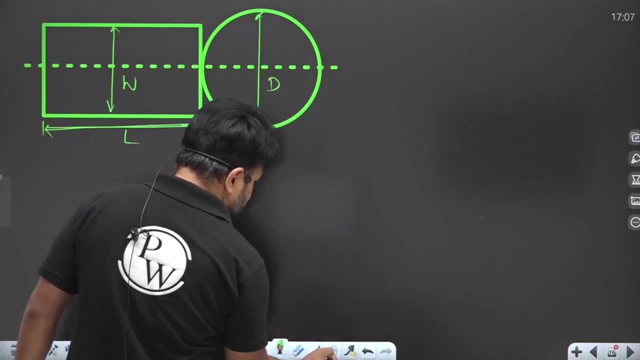 And the length of the workpiece is what. That is what That is a L Right Now. when the table is going to move, when the table is going to what? When the table is going to move, my dear See here. 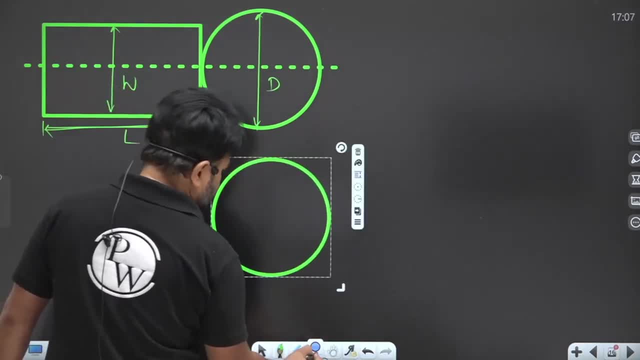 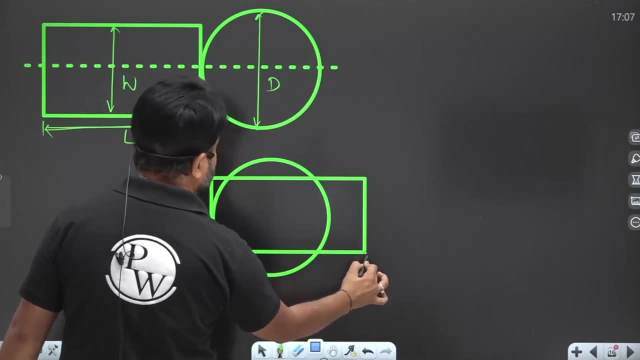 This is a milling cutter Again. this is a milling cutter Again. now, when the table is going to move right up to L distance, is the milling completed? Here the table move the L distance, Still the milling is not completed. 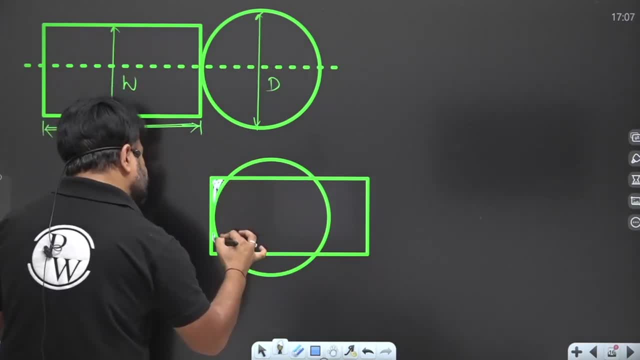 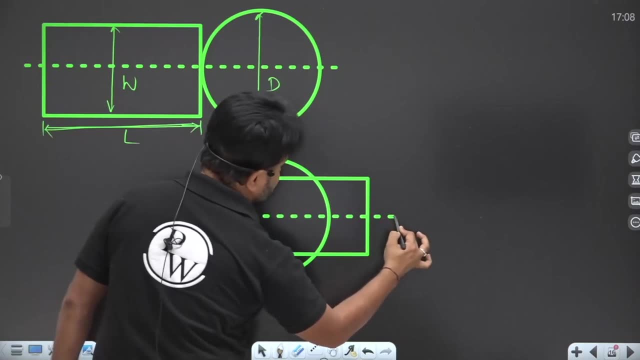 Why You can see, here There is the, that much material is remaining, which is symmetrical about the, which is symmetrical about the, this axis, This axis of what Symmetry? So it means that much distance. 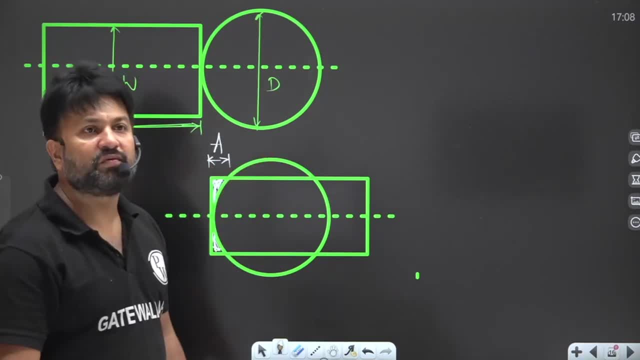 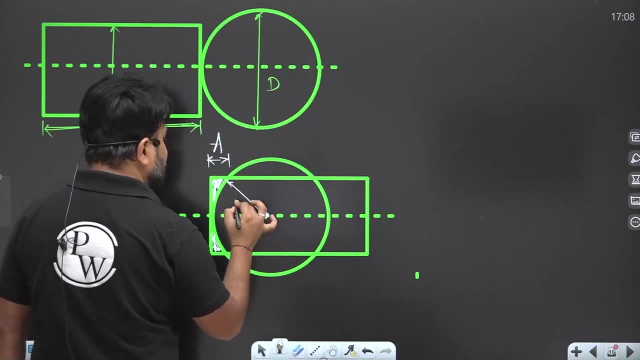 The milling cutter has to move or table has to move. So what is that A? You can find this A in a very easy manner. That is what That is: D by 2.. Right, That is what D by 2.. 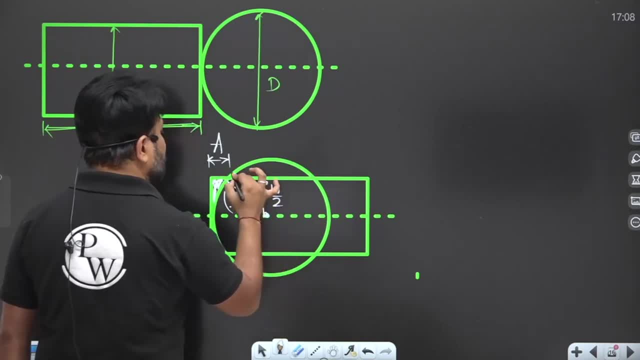 And that is what That is: W by 2.. Can you find this length? Yes, we can find this length, This length. okay, that A, How can I find that A? Still, this is what my dear D by 2.. 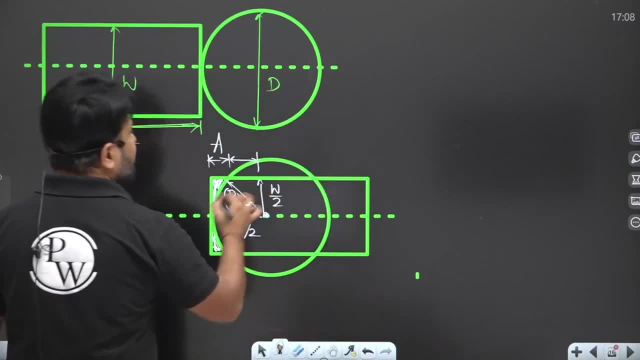 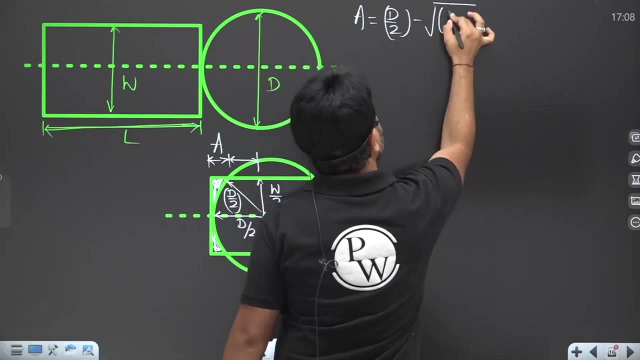 So from this length minus this length, So that A will be comes out, that A will be comes out: D by 2, okay, minus D by 2 whole square, minus W by 2 whole square right. 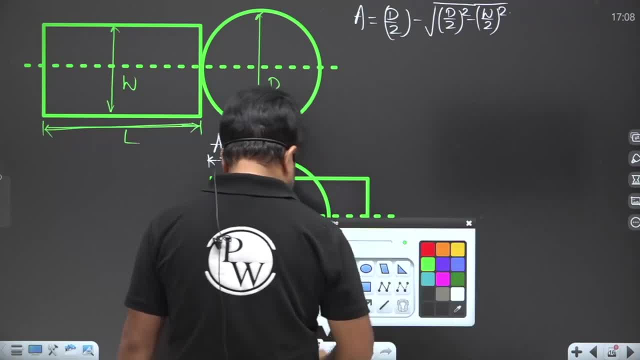 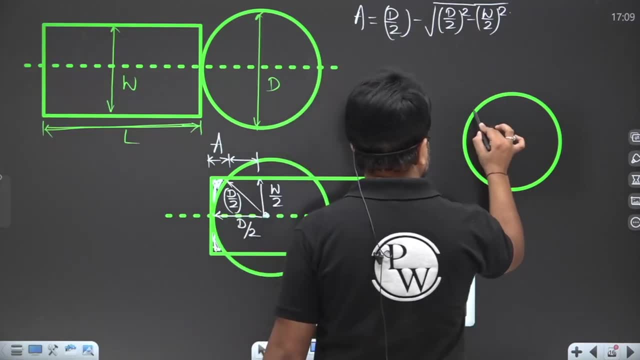 So this is the required distance which the milling cutter has to move, has to move right Now. here you can see, now this will be the final. okay, Now this will be the This thing. see. 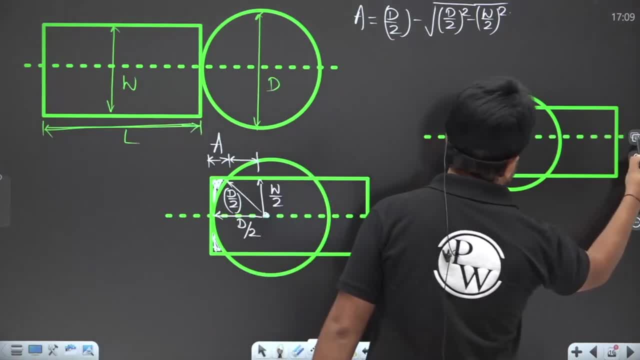 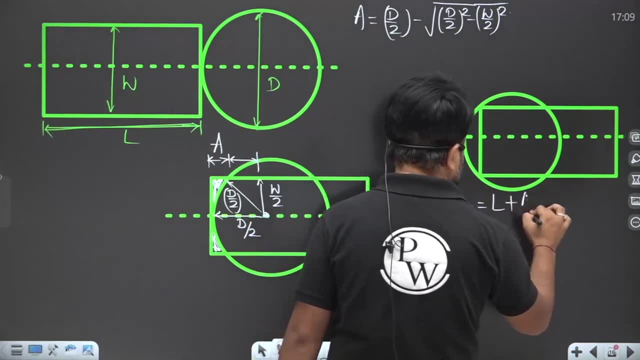 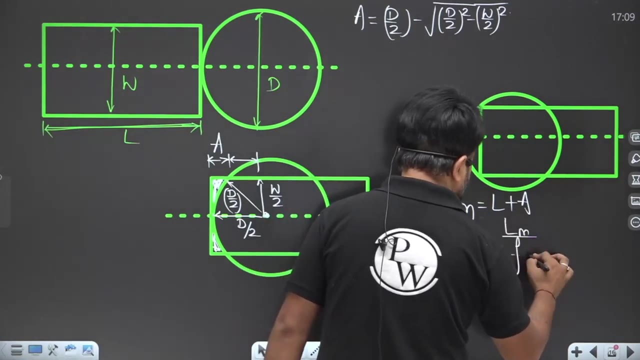 Now the machining is what Machining is completed. Now here that machining length is what The total machining length is. that is L plus A, Now the machining time. you can find out. that is what. That is the machining length divide by what. 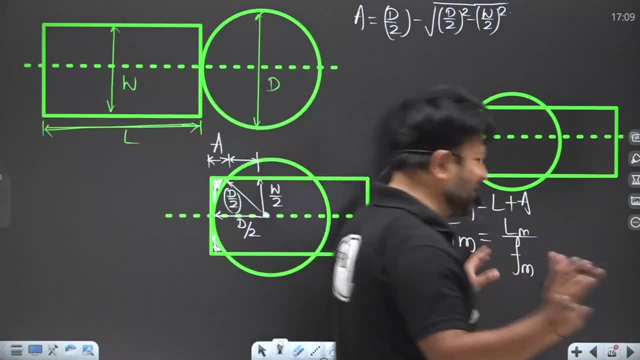 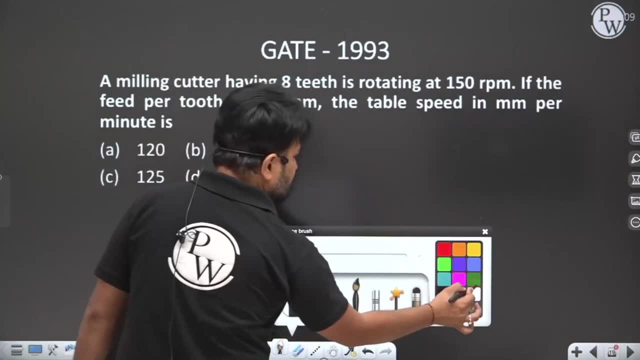 Table feed: Clear, Simple, very simple. Now let us discuss some question, My dear, this is a question. See, a cutter has a 8 teeth. that is Z equal to what? 8. Rotating with the RPM: what? 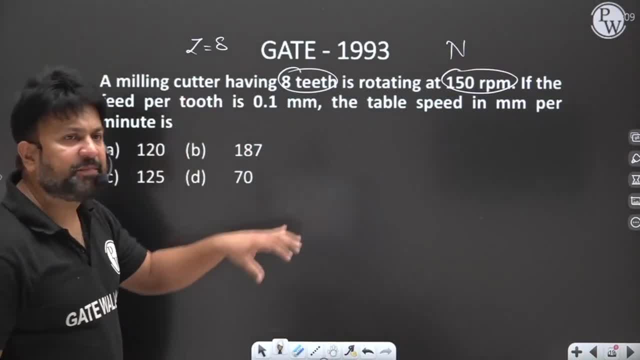 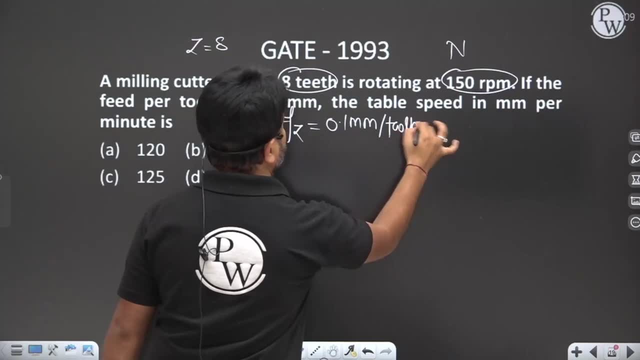 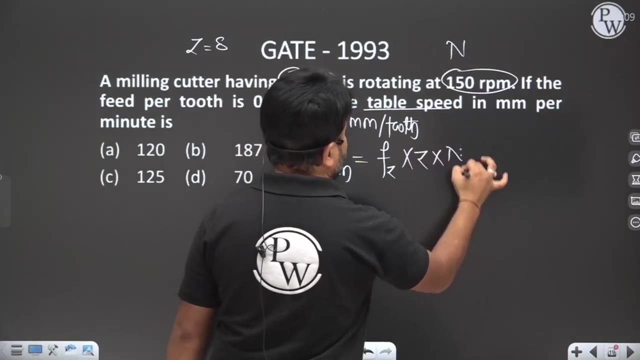 150.. So N is what 150.. If the feed per tooth, that is FZ, equal to 0.1 mm per tooth, right, then you have to find the table speed. Table speed is what That is: FM, FZ, into Z, into RPM. 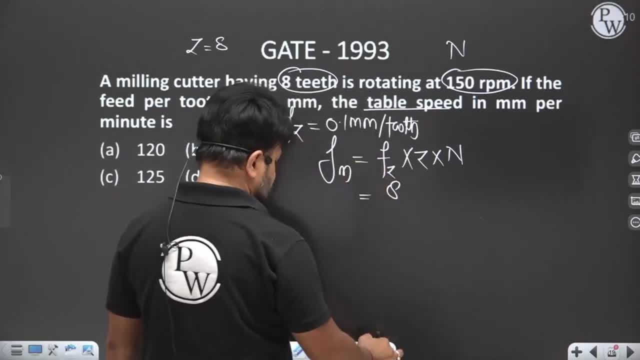 So FZ is what That is. FZ is what FZ is given to us. FZ is FZ is 0.1, right Z is what 8.. RPM is what RPM is 150.. 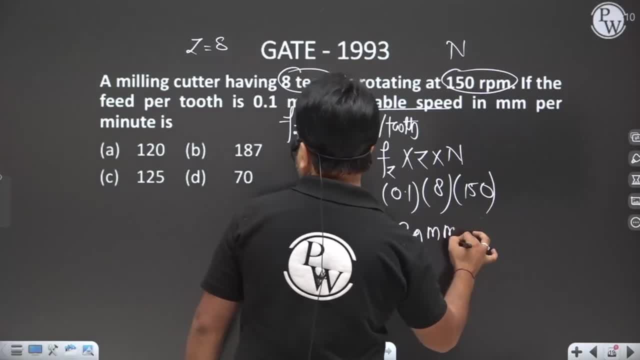 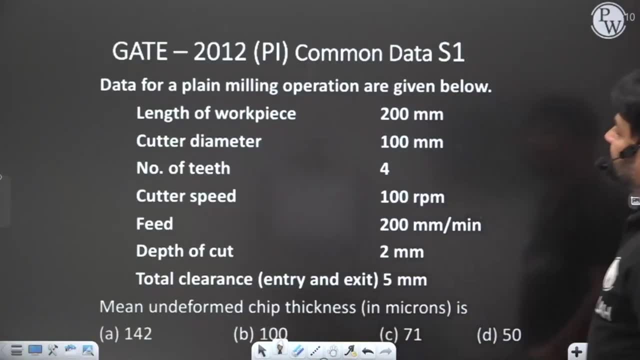 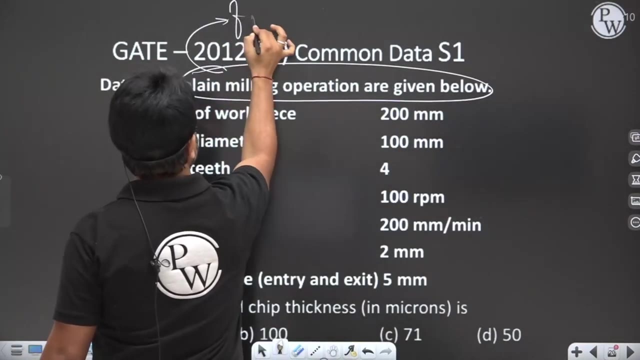 My dear. it will become 120 mm per minute. 120 mm per minute, Clear 120 mm per minute. Now our next question: data for plane milling, operation, Plane milling generally- what A face milling? Sorry, peripheral milling. 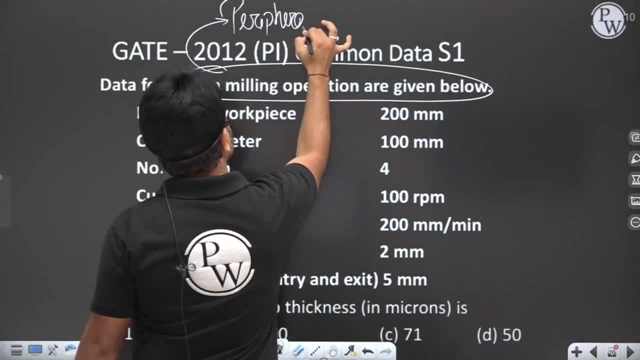 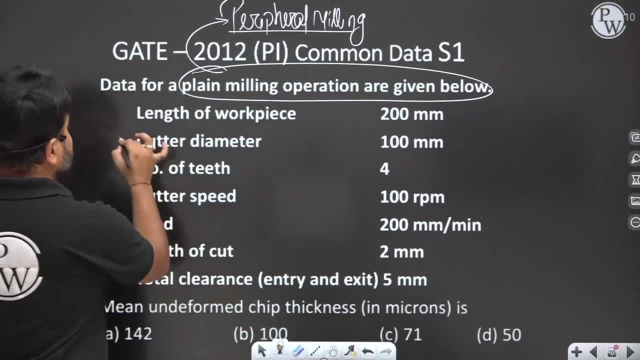 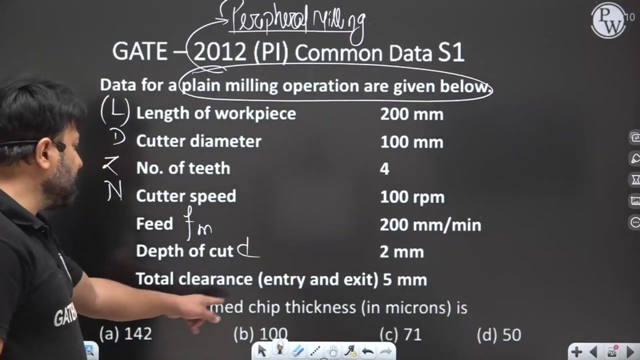 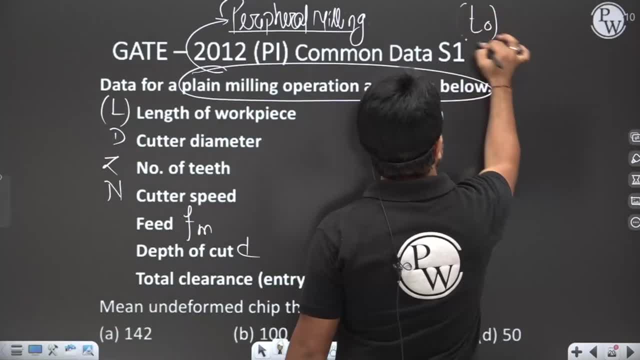 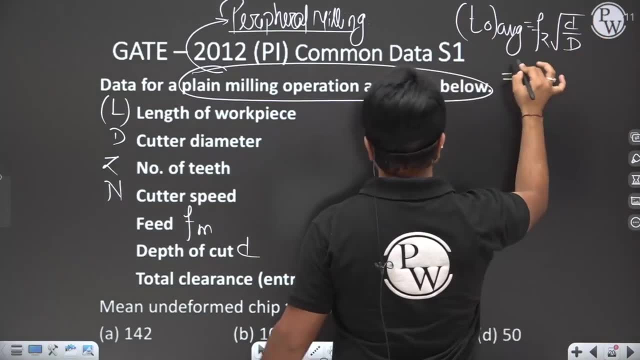 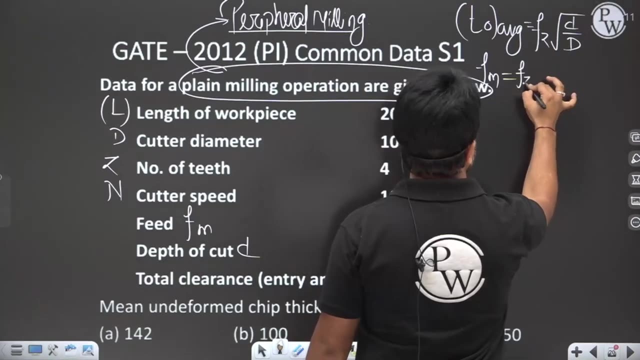 chip thickness mean undeformed chip thickness, that is a average chip thickness. you have to find that is fz root of small d by capital d, my dear, you have to find the small fz. so here, fm equal to fz into z, into rpm. fm equal to what fm equal to, given? that is 200 fz into number of t, that is 4. 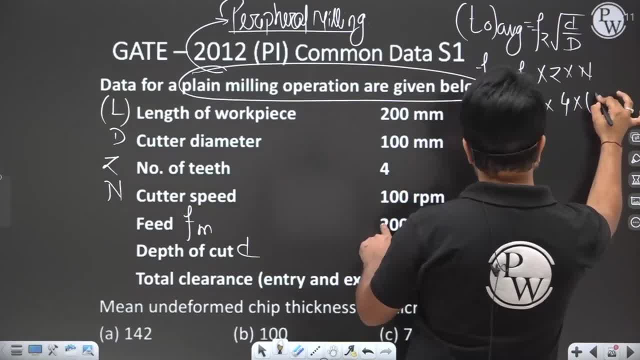 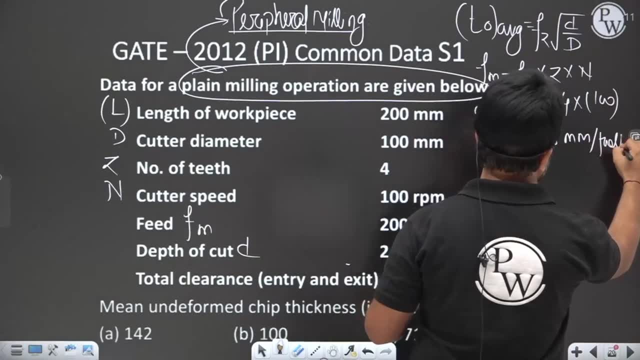 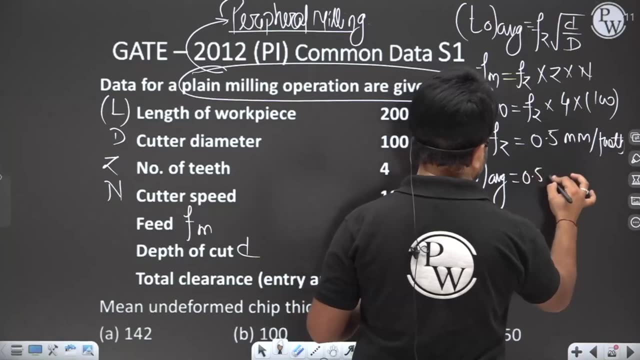 into rpm. that is what. how much that is? that is, that is 100, right? so fz will become 0.5 mm per tooth right. 0.5 mm per tooth. now t, not average, mean undeformed chip thickness is 0.5. root of small. 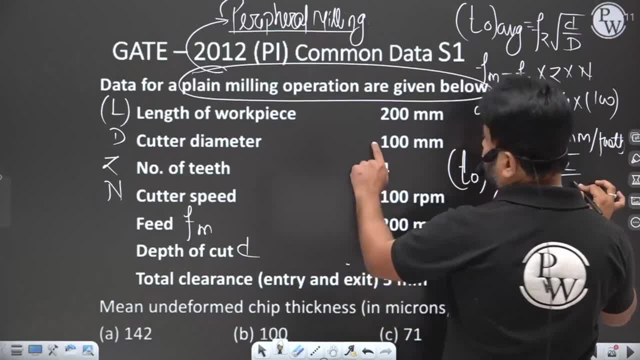 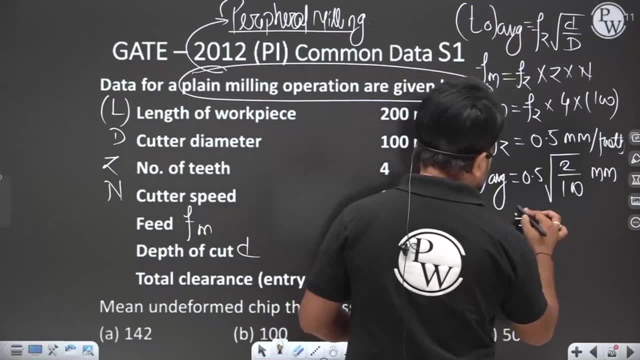 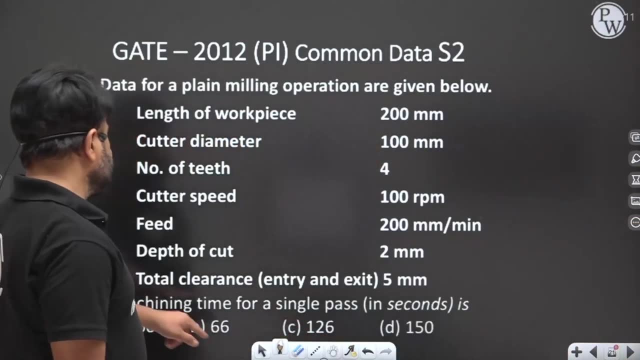 d. that is what depth of cut. that is 2 divided by diameter of the cutter, that is 100. okay, it will becomes in mm, but he is asking in micron. so nearby, it will become 71 micron. 71 micron it will be come right now. the next is the machining time for a single pass you have to find here. 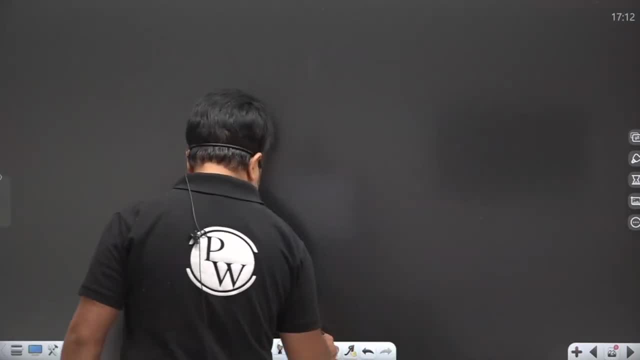 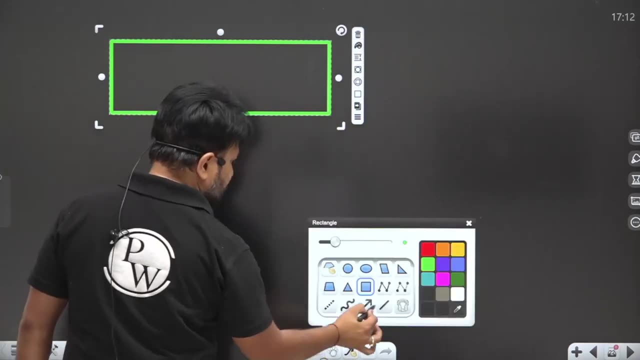 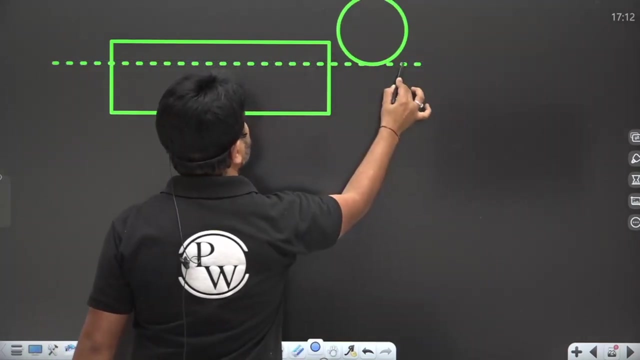 total clearance, entry and exit- is given. the thing is that i told you already my dear, i told you already here, basically, what is going to happen. this is a work piece, right? this is a work piece, and and, and, and, and, and. you have to machine this work piece, right? you have to machine this work piece here, my 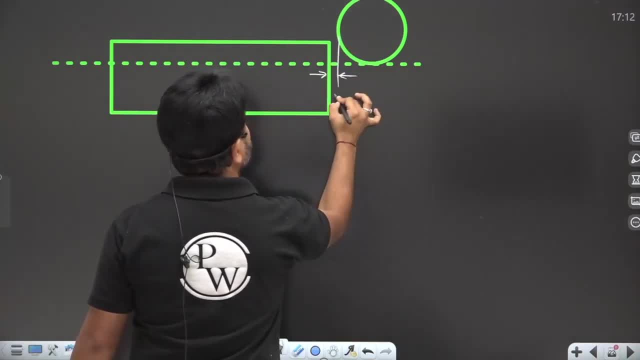 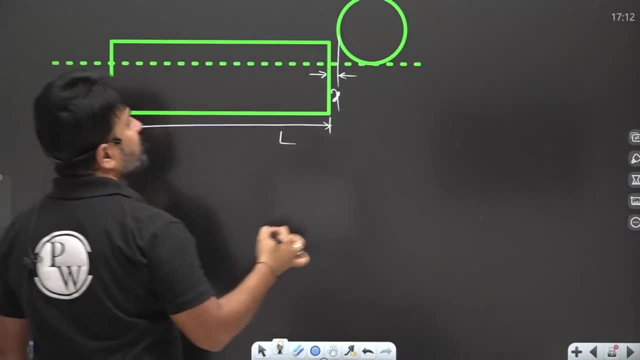 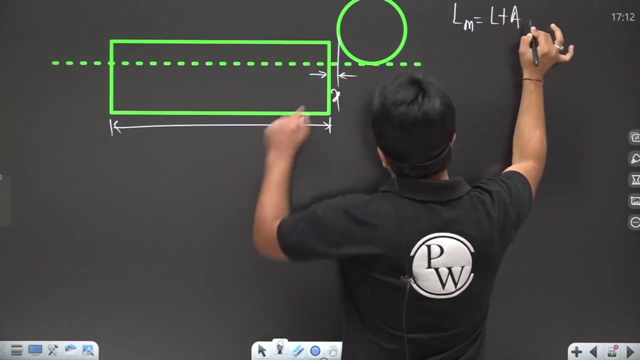 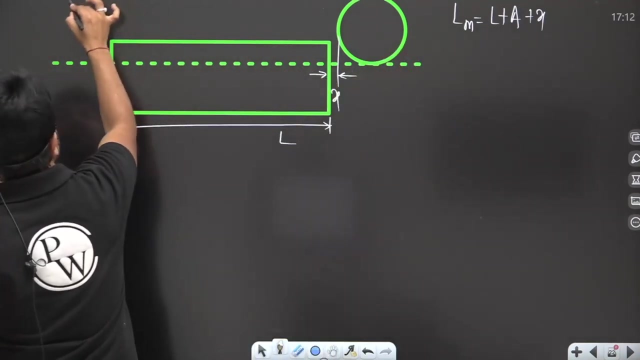 dear student, here you can see, this is the entry, that is x is given right. this is the machining length that is l is given, now basically the required. the required machining length is what l plus a here x is given. that is a approach now over travel. that is clearance. okay, that is what clearance it is given to us. 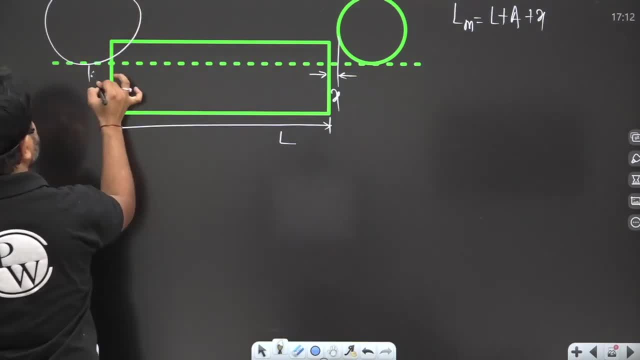 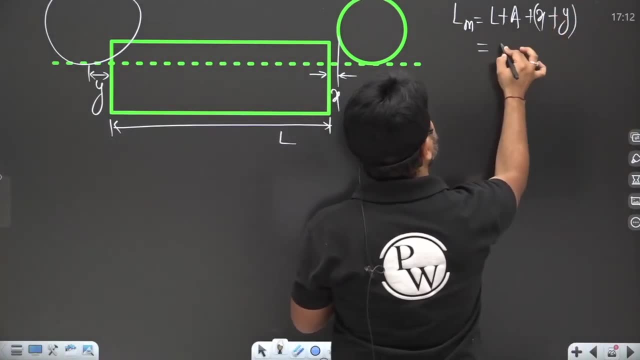 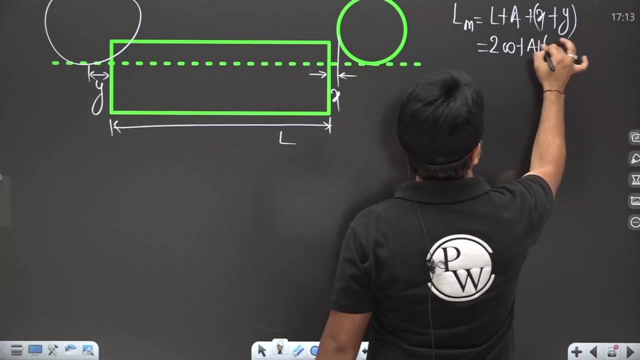 that is what clearance that is given to us. this is what this is. let's say y, that is clearance. let's say y and x plus y, equal to what that is 5. l is what l is given to, what that is. 200, that is what 200, right. a x plus y, that is what. 5, what is a? here a, you can find a that is root of. 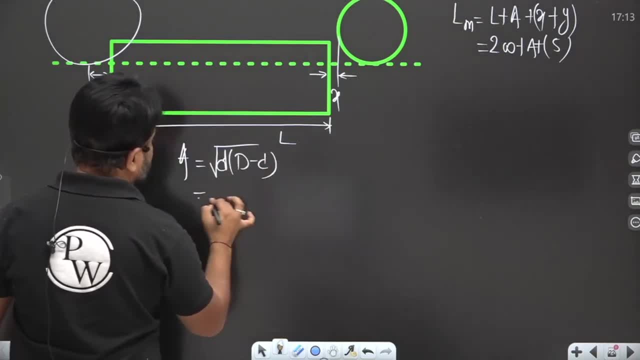 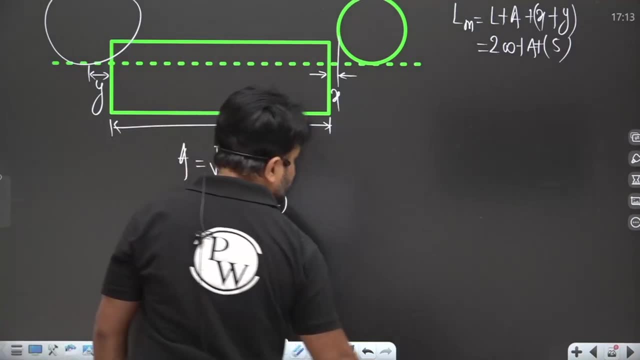 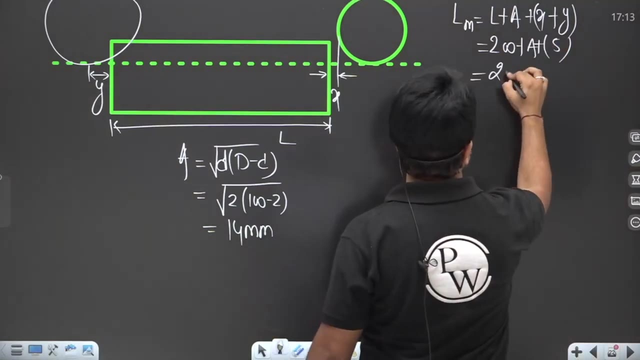 small d, capital d minus small d. root of small d, that is 2, capital d, 100 minus 2, it will become what? 14 mm? right, it will become 14 mm. idea now, once you get the a, so add here 14, 14, so 200 plus. 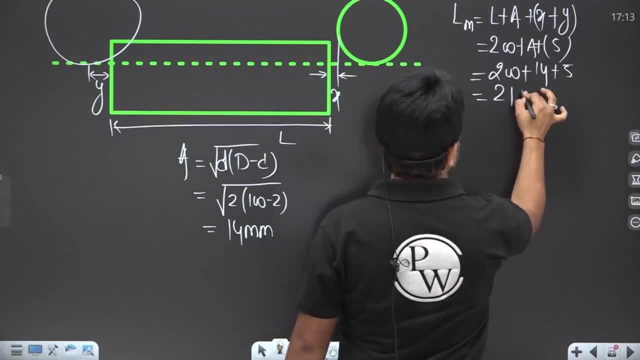 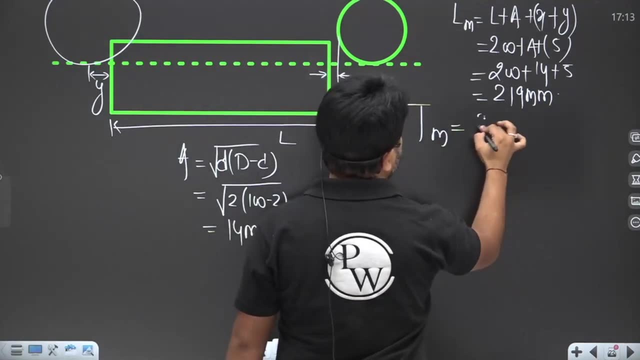 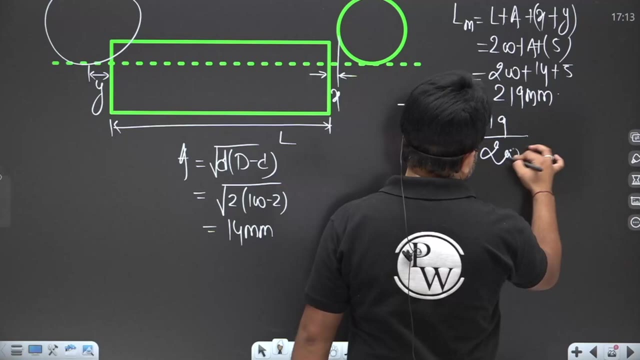 14 plus 5, so it will become 219 mm. right, 219 mm. now we have to need the machining time, that is lm. machining length: that is 219 divided by what? divided by 200 mm per minute. 200 mm per minute. so here the answer. 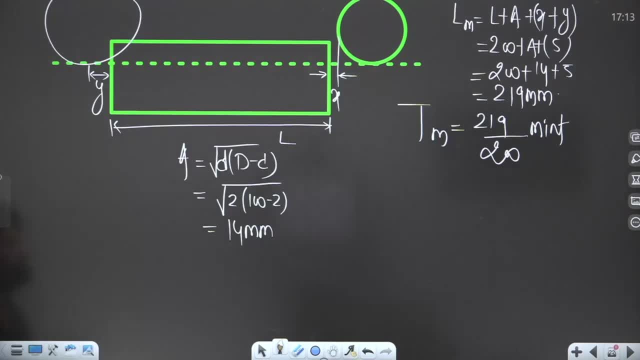 comes here minute, but but. but the given answer is given in the second. so 219 divided by 200 answer into 60, it comes 65 0.7 second right, that is approximated as 66 second. now we are going to start a grinding. 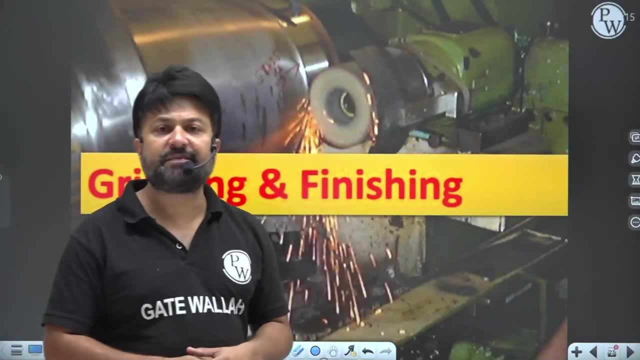 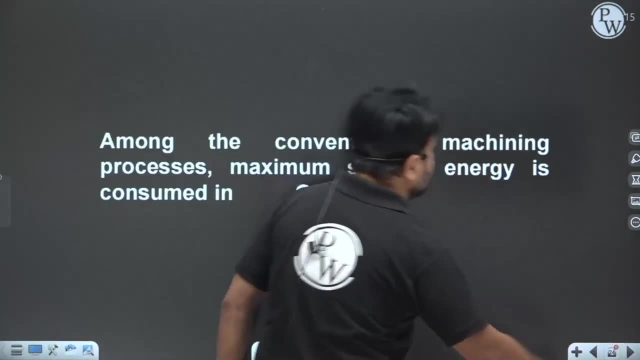 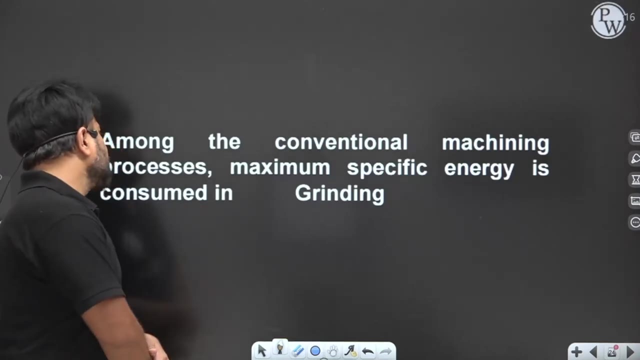 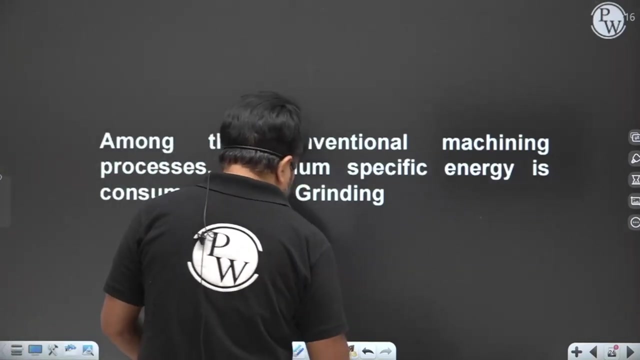 operation. right, grinding as a finishing. basically, grinding is what grinding generally is: a finishing operation. right now let me discuss with the grinding, my dear grinding. basically in conventional machining, grinding is a process. grinding is a process which has a maximum is possible and that G right which has a maximum, a specific energy right, why let 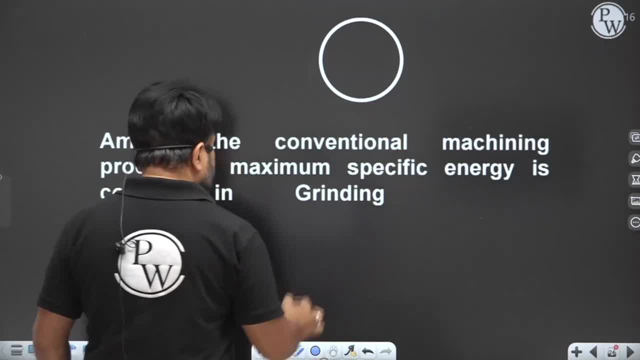 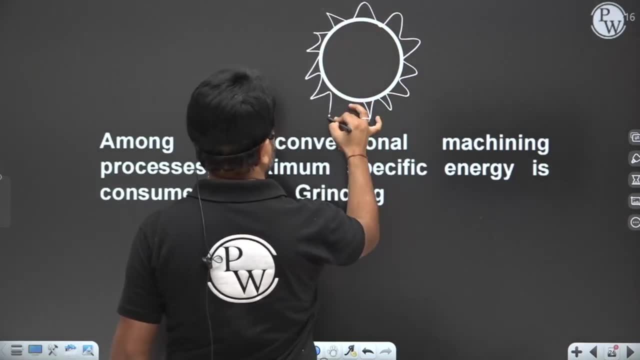 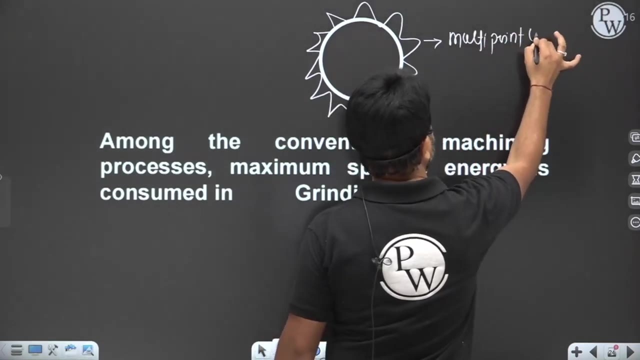 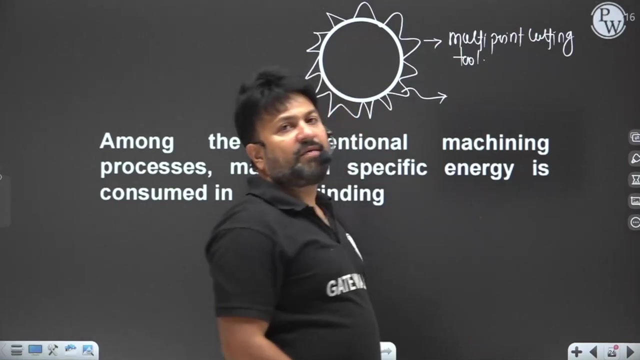 me give the explanation. this is a green ink bead on, this is a abrasiveIO Right. give you the expliation. this is a grinding wheeland this is a abrasive particle. this is a abrasive particlethis is всем eye a abrasive angle. These are what These are, generally negative rake angle. I am going to tell you. 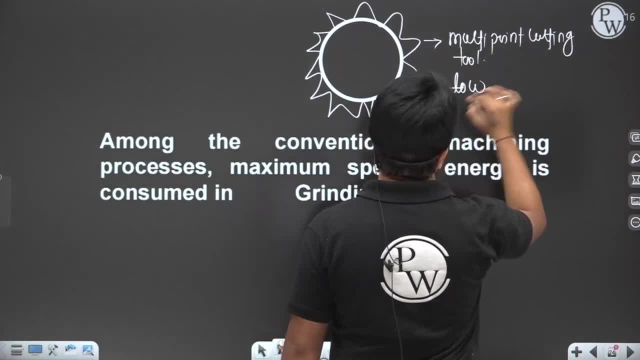 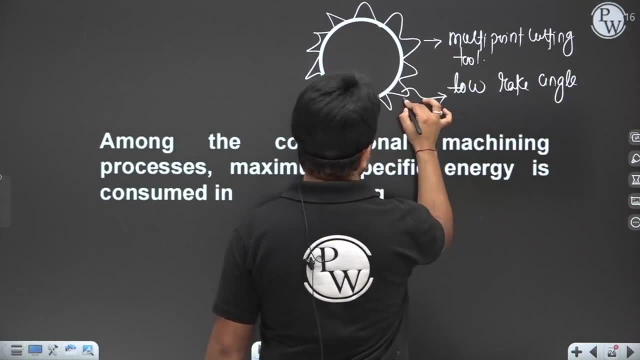 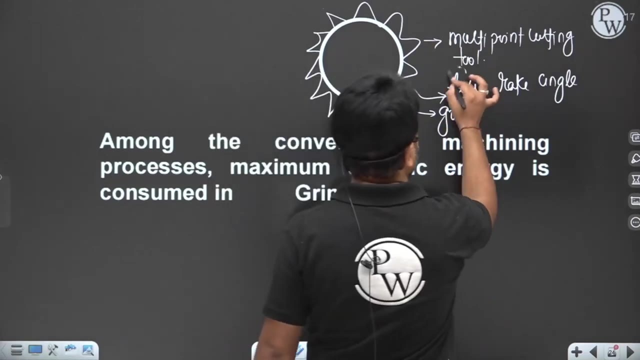 generally, these are what Low rake angle, Low rake angle, Low rake angle. Okay, Low rake angle. These grit, These are what These are known as grit, These are known as grit And these grit or abrasive particle has low rake angle And you know the concept As the 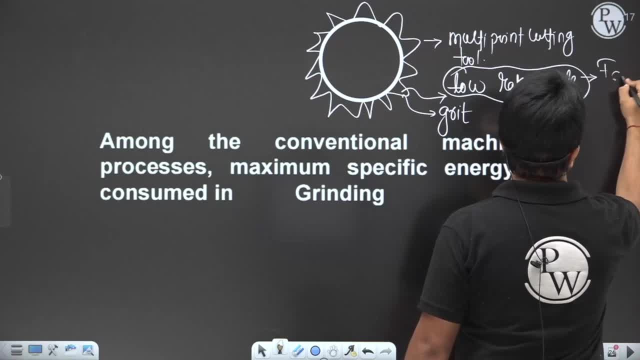 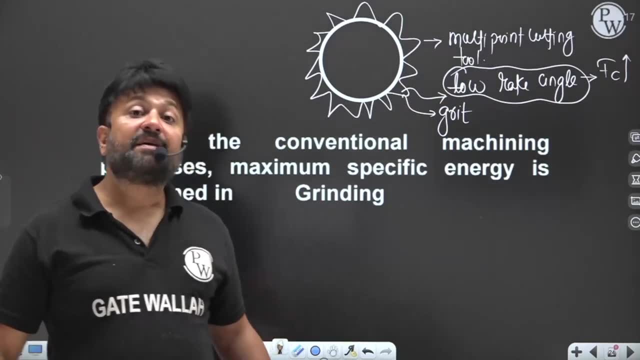 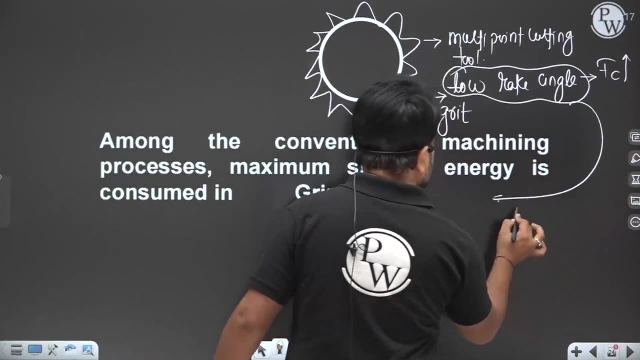 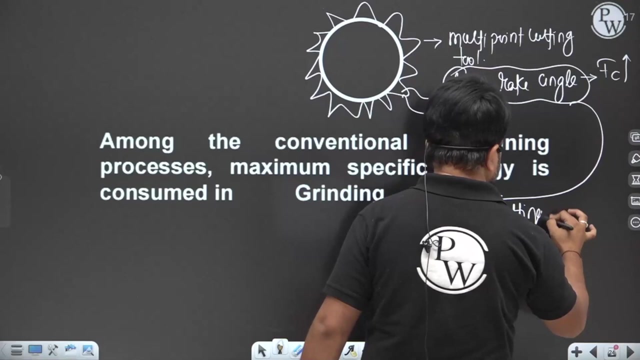 low rake angle is low, then the cutting force increases. Then here every grit is going to do a machining operation means the cutting force is going to increase in a very high manner. Also in a low cutting rake angle. the required cutting velocity, Required cutting velocity, Required cutting velocity is what Is high. 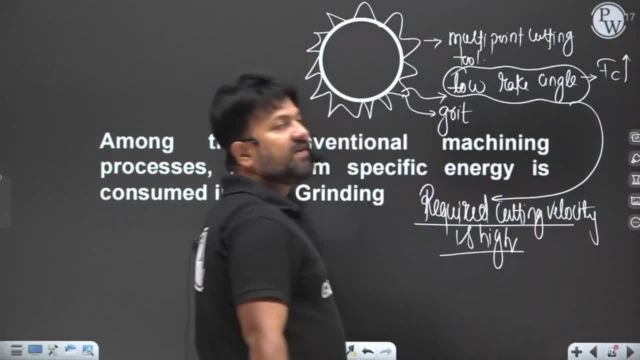 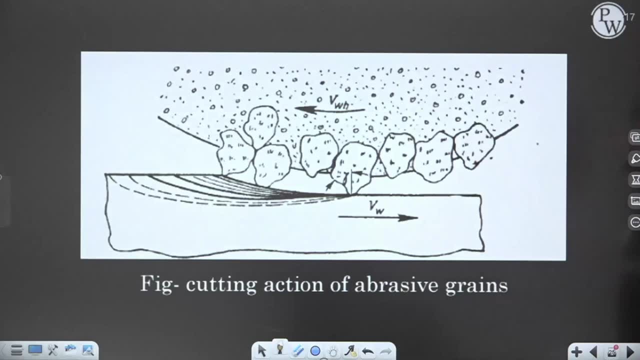 Because low rake angle tool are not able to penetrate into the work piece. So that's why power consumption is going to be increases. That's why lot of heat is going to be produced in the grinding operation. Here you can see the grinding wheel And here in the grinding 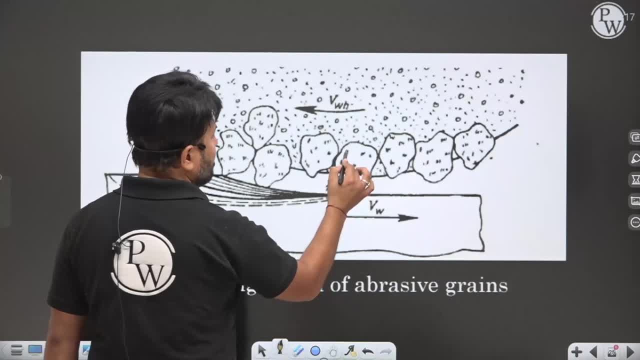 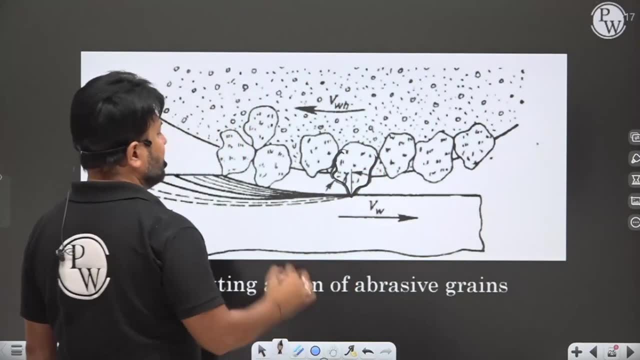 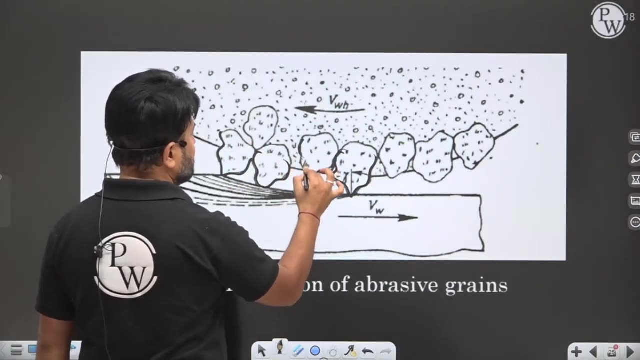 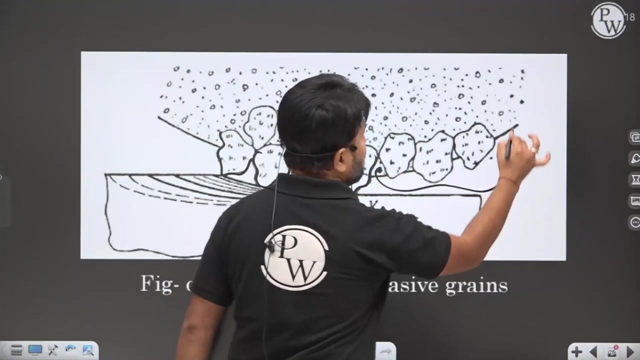 wheel. you can see that a grinding- Okay, Grit, That a grinding grit, Grinding grit. See. See, this is a grinding grit. See, this is a grinding grit. See, this is a grinding grit. Generally, grinding grit has what A low rake angle. Now, this space is known as intergrit. 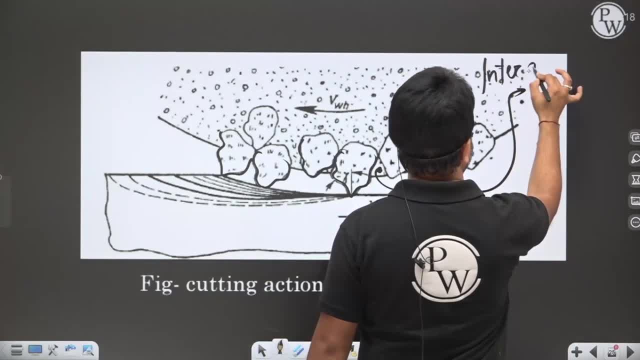 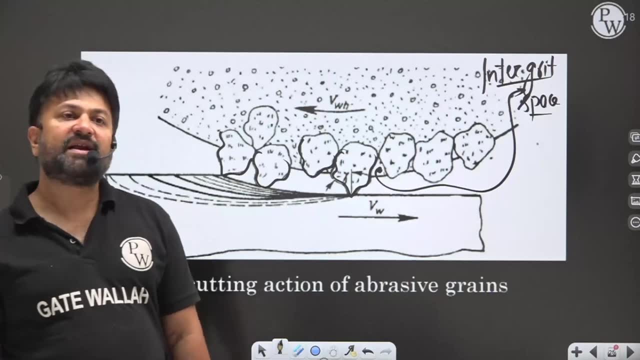 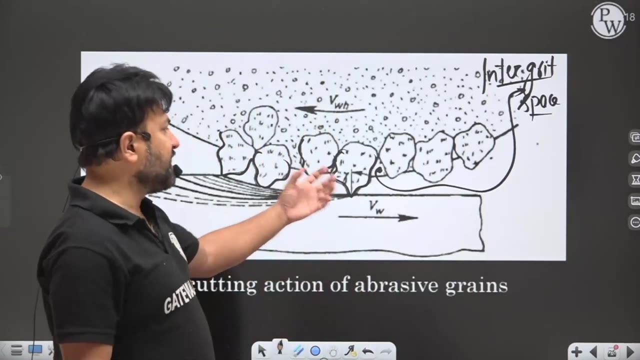 space, Intergrit space- Okay, Intergrit space. Generally, in intergrit space, the chip is going to be accommodate here. Cutting fluid is going to be accommodate here. Okay, This is a pocket of what Cutting fluid. Right, This is a pocket for what? A cutting fluid? Okay, This is a 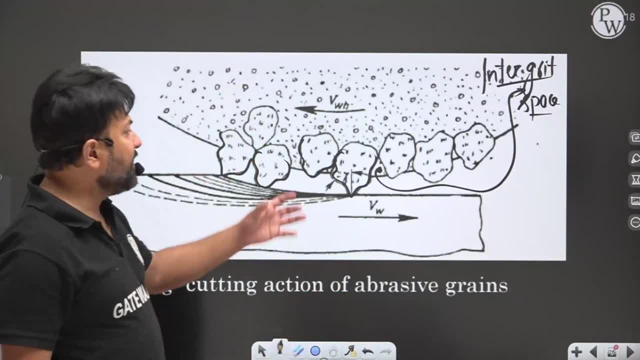 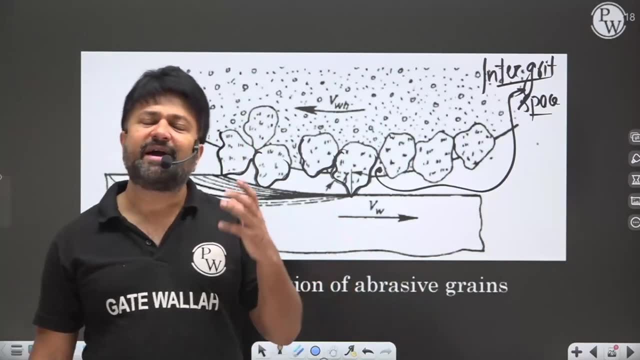 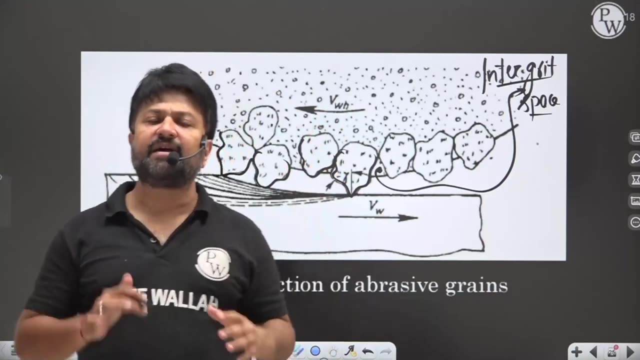 pocket of what A cutting fluid. As I told you why we require high cutting velocity, Why we require high cutting velocity in the grinding, It is desire to offset the adverse effect of, It is desire to offset the adverse effect of very high negative rake angle and 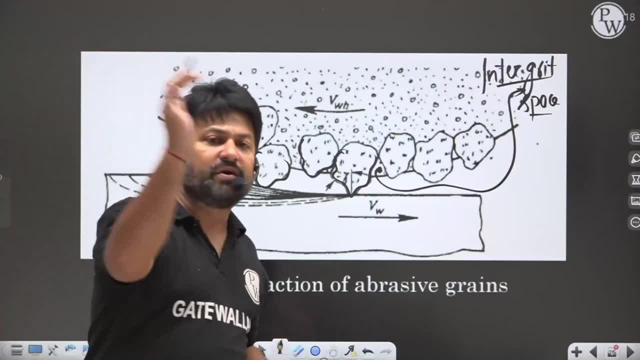 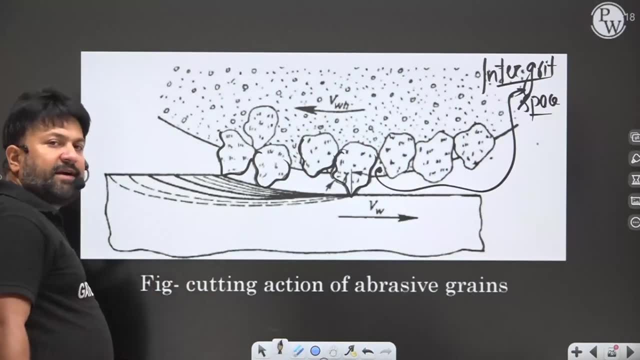 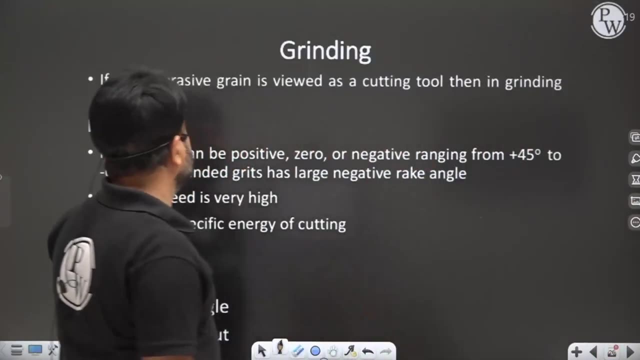 low rake angle of the working grit To reduce the force per grit as well as overall grinding force. Right, Otherwise the grit is not going to be penetrate into the work piece. Right, The grit is not going to penetrate into the work piece. My dear, you have to remember some. 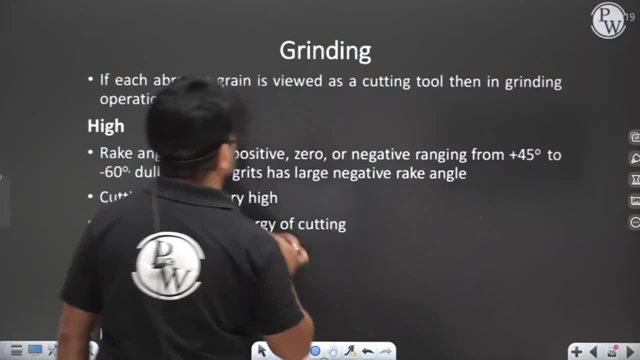 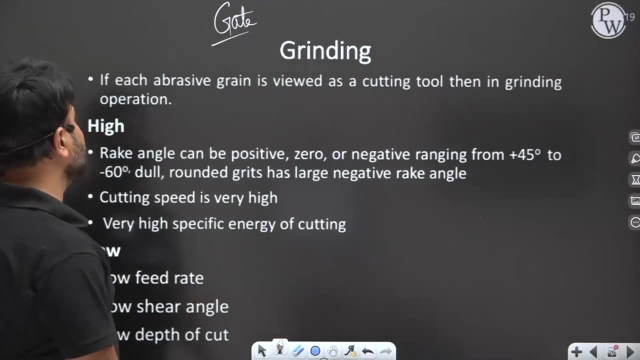 of the very important thing. Okay, In this operation for a gate purpose, For a gate, for a gate exam, you have to remember some few point which is very important. Okay, In terms of grinding. In grinding, some of the parameter are high, like rake angle. Rake angle may be. 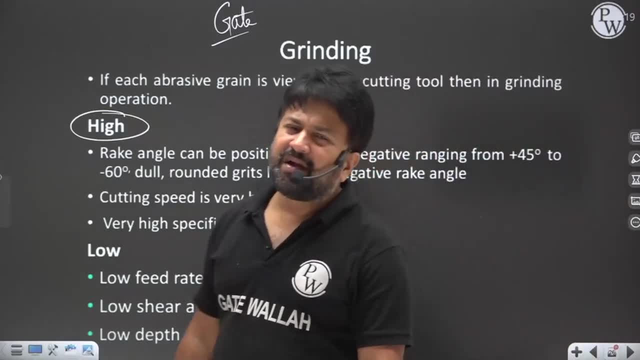 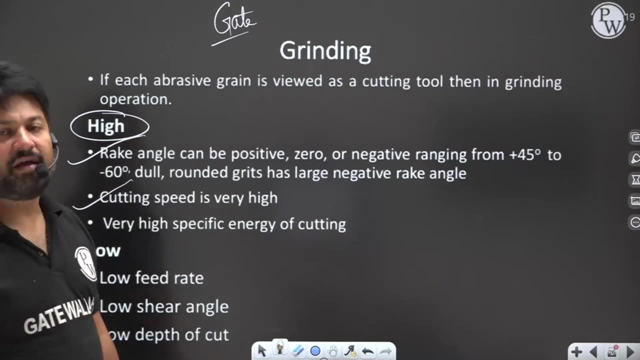 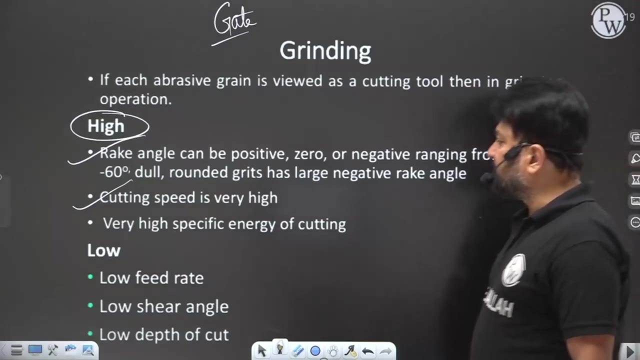 highly positive, highly zero or highly negative Right, But mostly low rake angle, we are going to be found. Okay, In grinding the required cutting velocity is very high because we have to overcome the adverse effect of negative or low rake angle. Here the specific cutting energy is going. 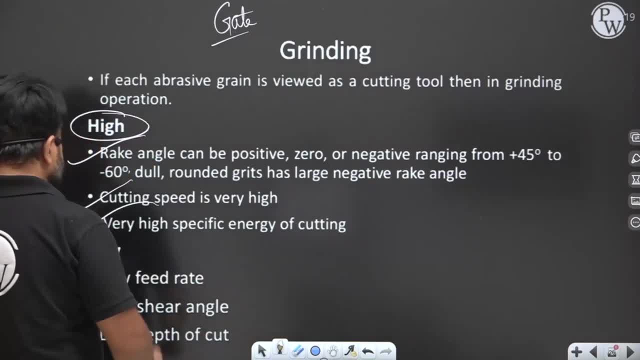 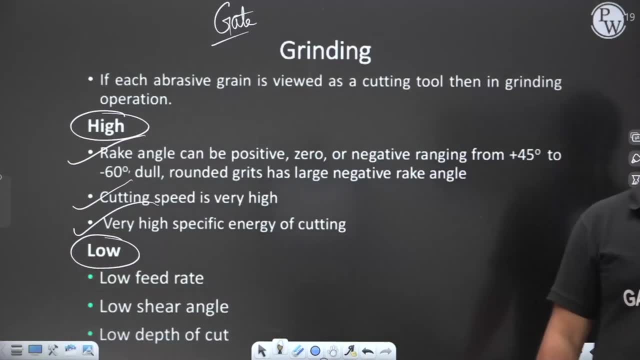 to be what? Very high, Even. there are some parameter which are very low. and what are they? Here we keep low feed rate. Here we keep low feed rate. Okay, Because of, because of low rake angle, the shear. the shear angle is also low, My dear. we have already seen. 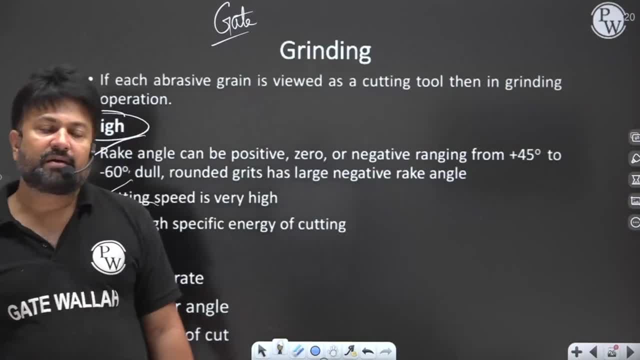 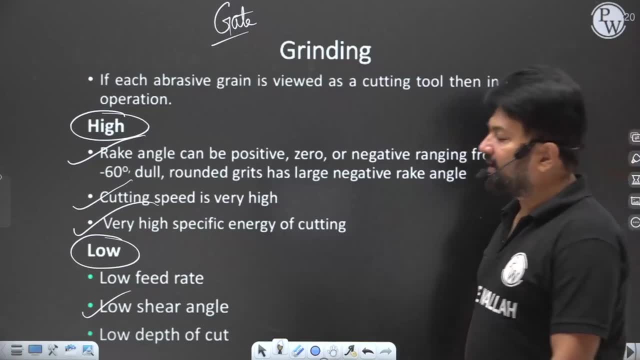 that, because of the low rake angle, the, the grit, are not able to okay penetrate into the work piece. that's why we need a high cutting velocity and because of the high cutting velocity and because of the low rake angle, the overall power consumption is going to be increases. 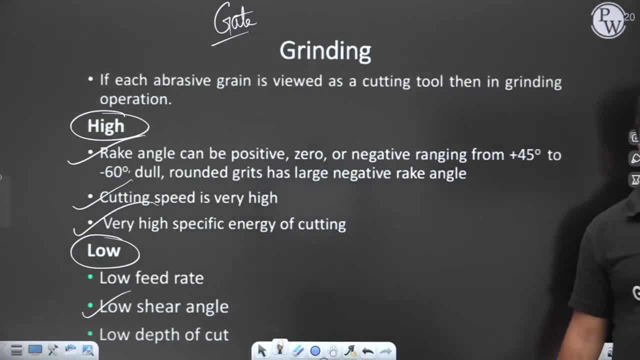 So we are not going to, we are not able to, we are not going, we here, we are not going to increase the depth of cut. Why? Because if you are going to increase the depth of cut, in that case, then what happened? Then? what happened, my dear, If we increase the depth, 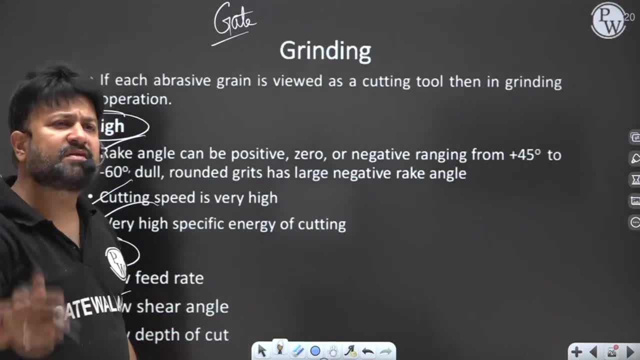 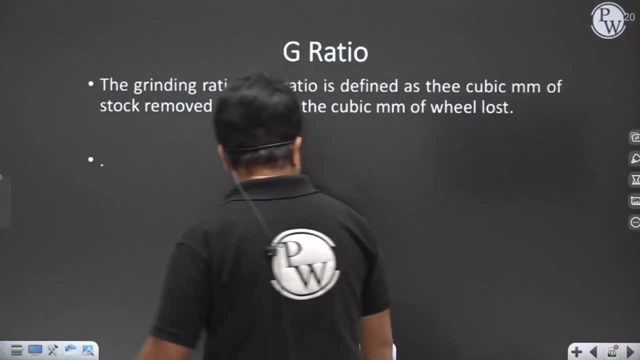 of cut my dear, then power consumption again is going to increases, okay, which is not very economical. which is not very economical? Now, what is the g ratio? What is a g ratio, my dear? This is a grinding wheel, right? This is what This is: a work piece. Okay, Suppose. 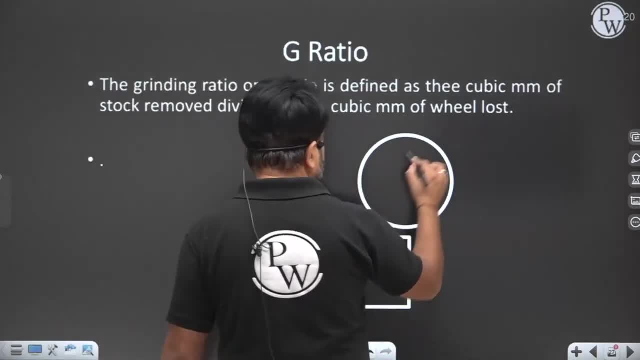 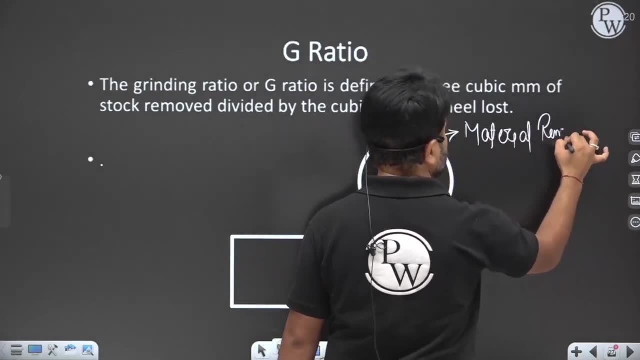 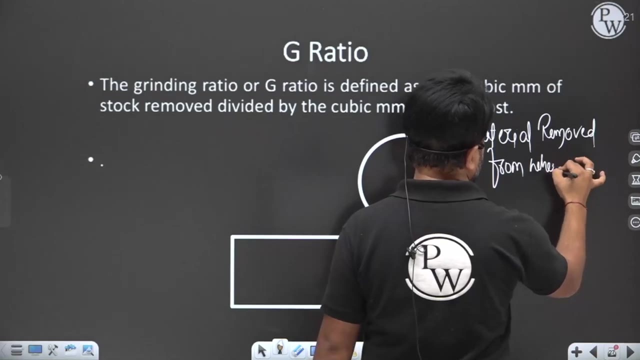 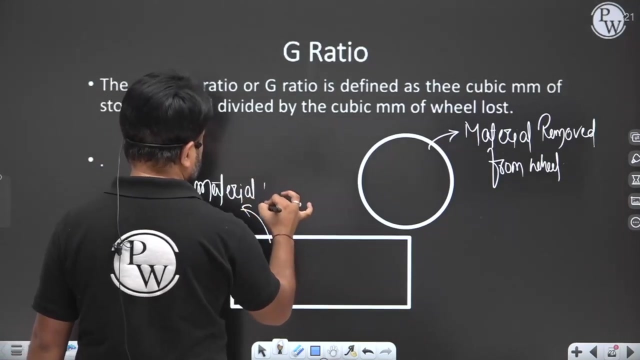 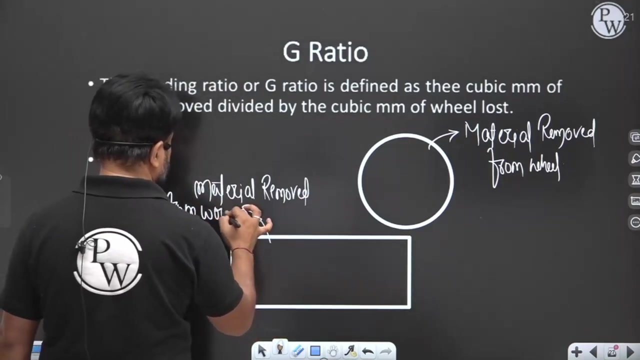 that during machining, some of the material is going to be removed, some of the material, material material removed or MRR material removed, Okay. So material removed from wheel from wheel: okay, while machining and material removed and material removed from work piece from work piece. during what? During machining? 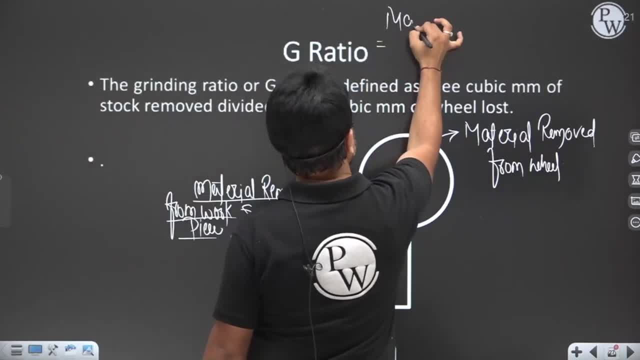 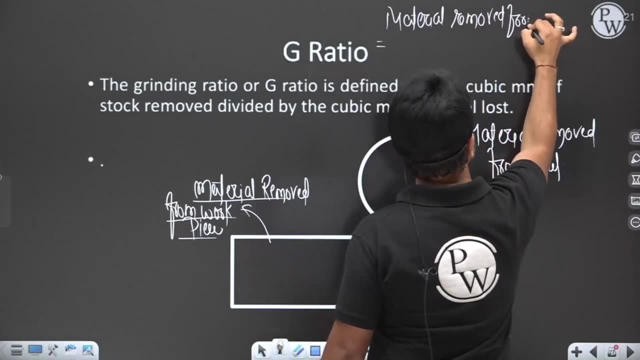 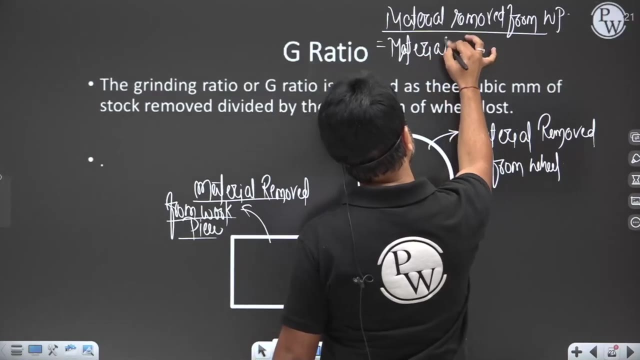 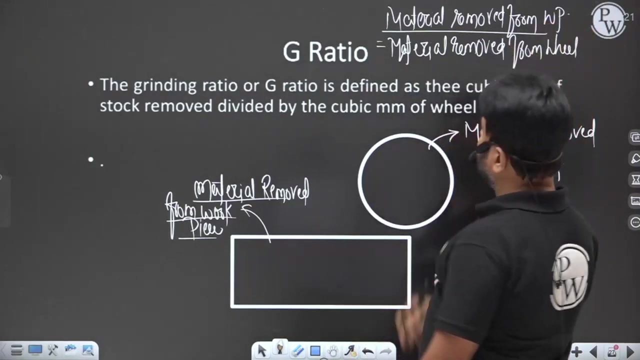 So g ratio, basically material removed, Material removed from work piece. WP stand for work piece. divide by material removed from wheel, from wheel, right from wheel. that is a g ratio. Let me tell you about the grinding ratio. Let me tell you some fact about the grinding ratio, my dear, In conventional grinding. 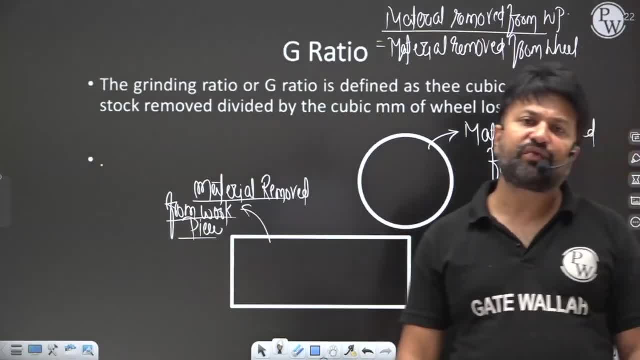 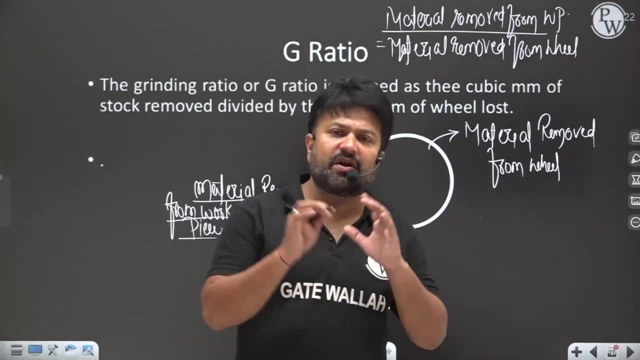 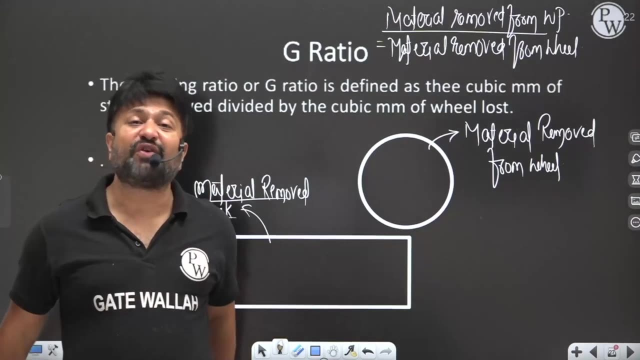 the g ratio is in the range of 20s to 1 to 80s to 1.. The g ratio is a measure, the g ratio is a measure of grinding production and reflects the amount of and reflects the amount of what amount of work, amount of work a wheel can do during its useful life, during its useful 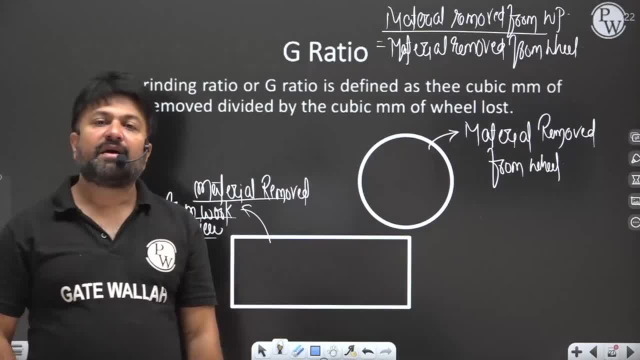 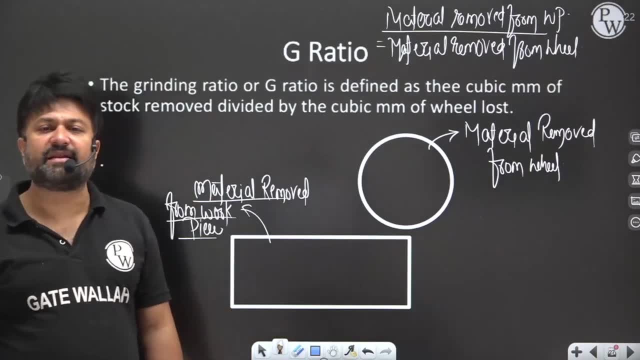 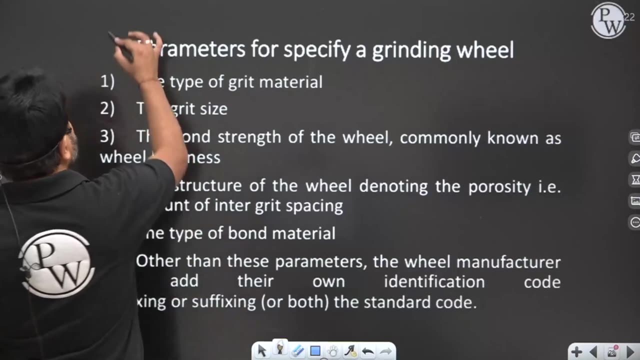 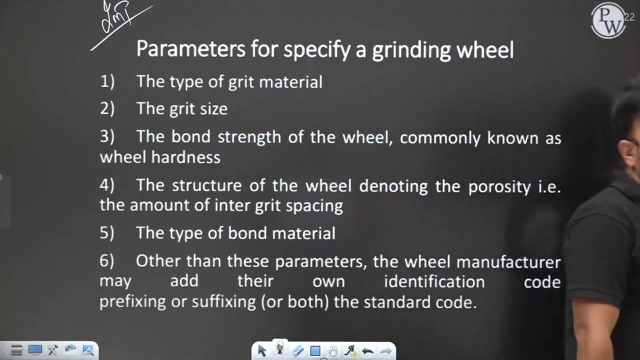 life. As a wheel losses material, it must be reset or repositioned. repositioned to maintain the work piece size right, to maintain the work piece size right There are. this is a very important side, my dear. by this parameter you can- you can basically decide that which grinding wheel we have to use, basically in 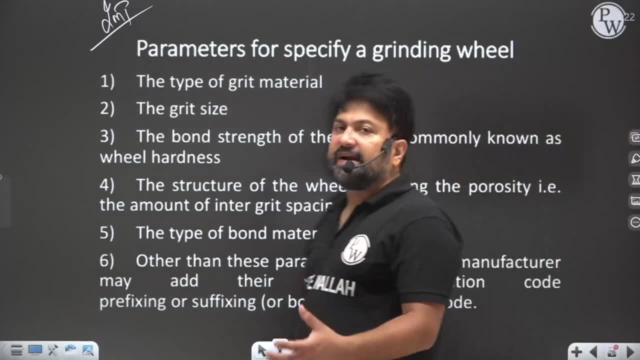 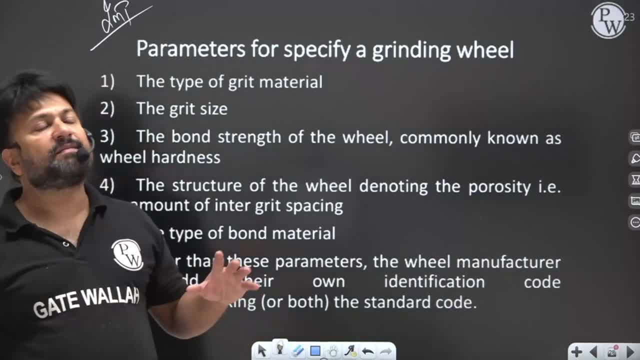 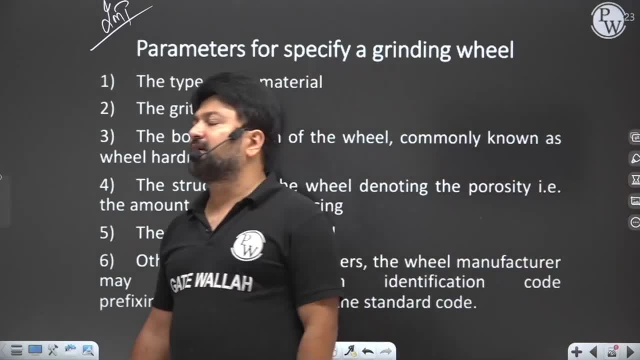 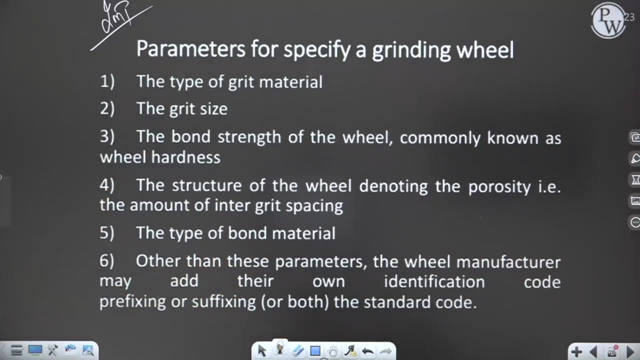 In finished grinding, we have to select somewhere some type of other field, right? So by which parameter? You can decide that for Guiding, we will select, that will. finish grinding, we will select, that will Be right. So we are some parameter. this is about a lot, right. There are basically five main parameter. the first parameter is: 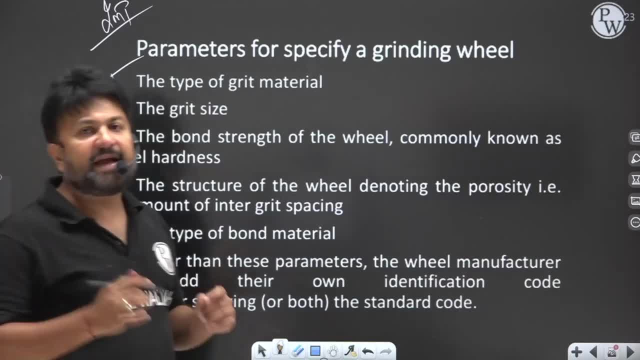 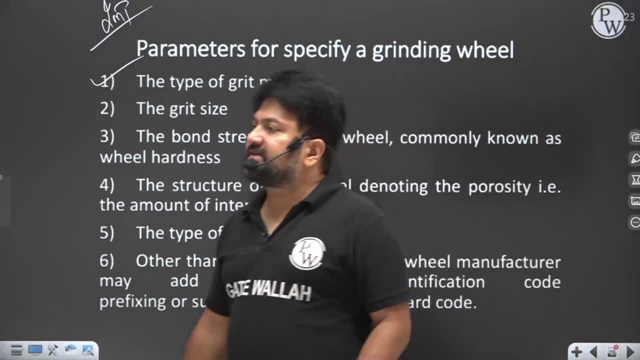 what? the type of grid material, my dear, Yes, the type of grid material. what are the type of grid material? okay, What type of material? basically, the grit basically we select, like it is not going to react with the workpiece at a very 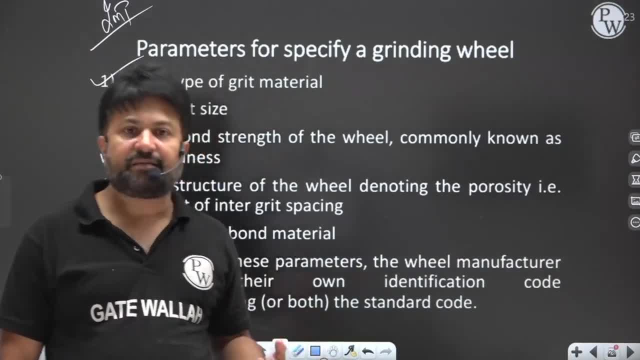 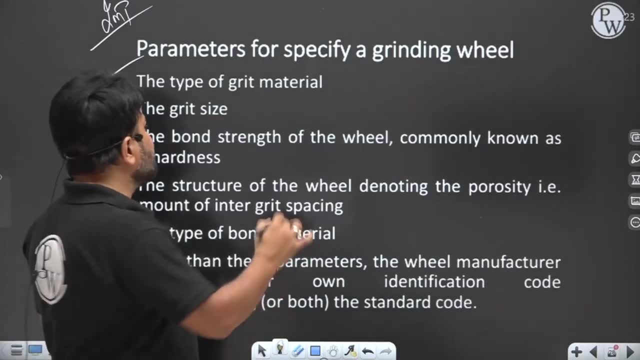 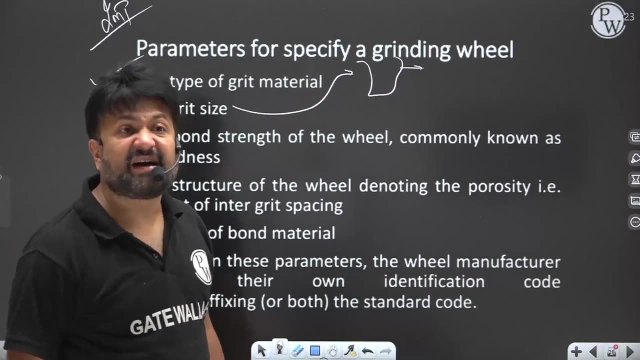 high temperature, generally, silicon carbide and aluminium oxide. right the grit size. yes, the size of the grit may be large and the size of the grit will be low. if the size of the grit is large is large, then material removal capacity is high. if the material removal capacity, if the size of grit 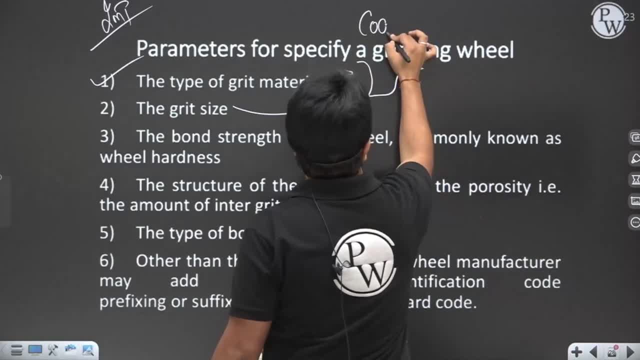 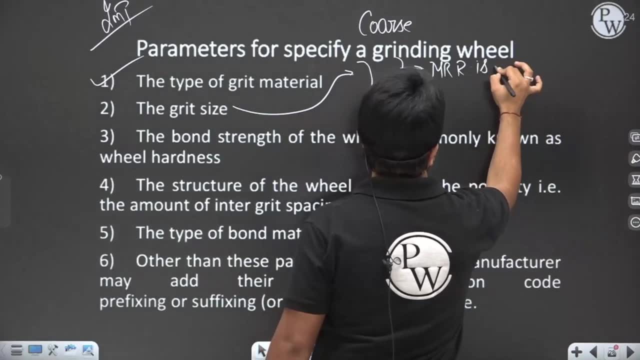 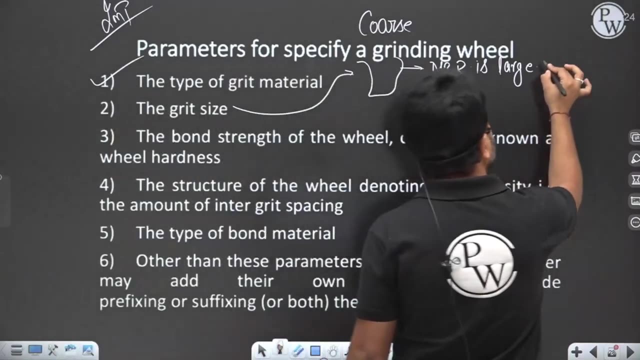 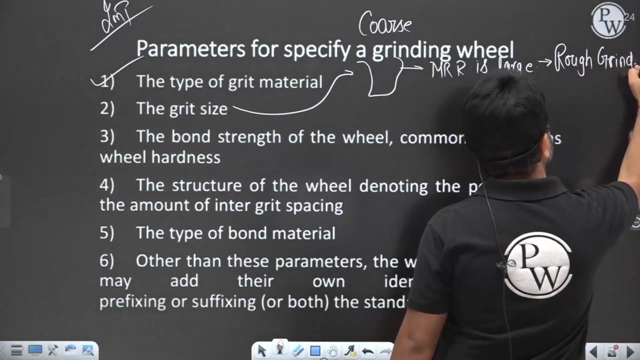 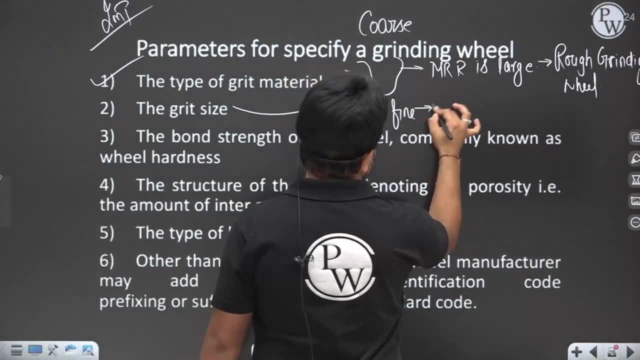 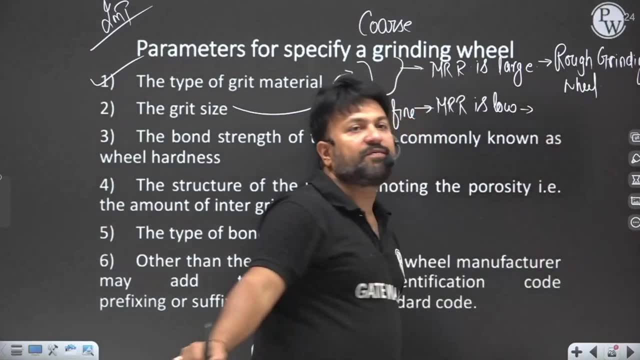 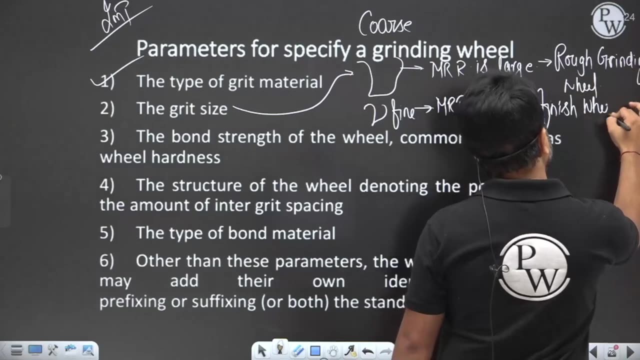 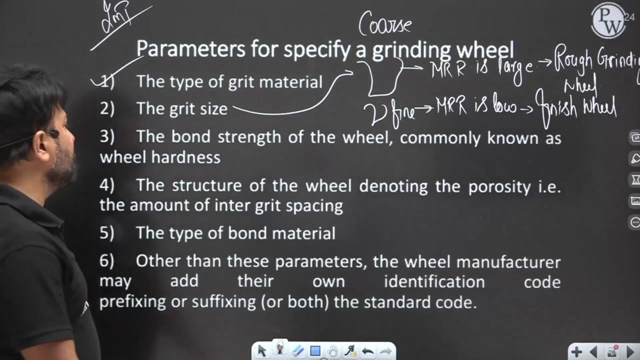 then if we select a fine grit- this is what fine grit- then mr r produced by this grit is low. then this type of grit we are going to use in finish, we in finish, we right in finish wheel. now let me tell you the next parameter, that is, the bond strength of the wheel, commonly known as what? 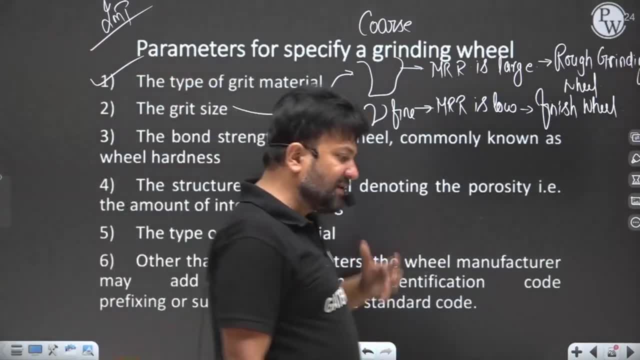 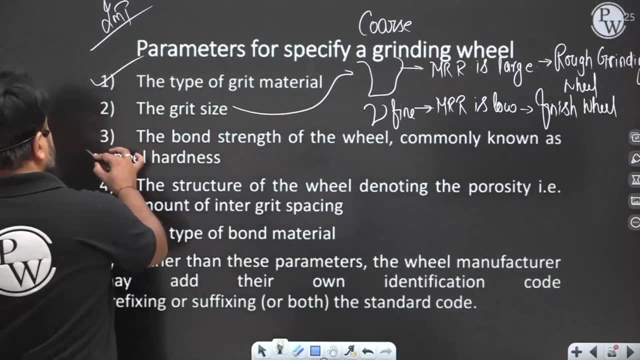 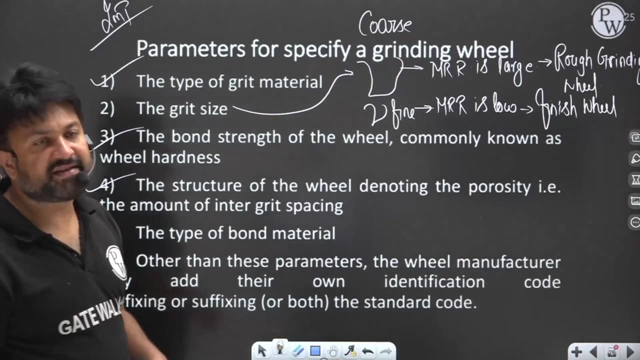 will hardness that. that parameter tells that how tiny, how much harder these cornerkam's much tightly the abrasive particle are hold in the wheel right, how much tightly the abrasive particle are hold in the work piece. Fourth parameter is structure of the wheel. yes, open structure or chorus structure. 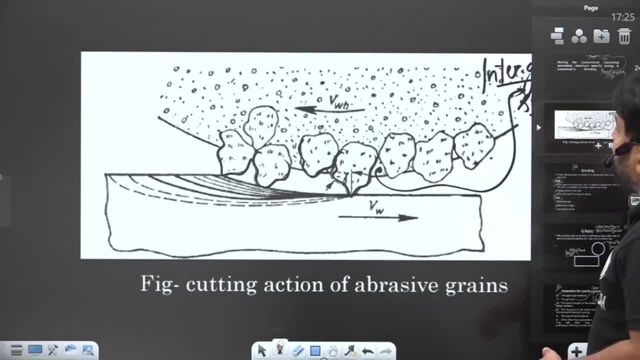 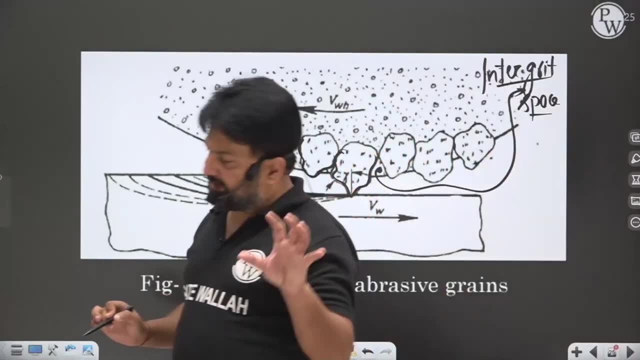 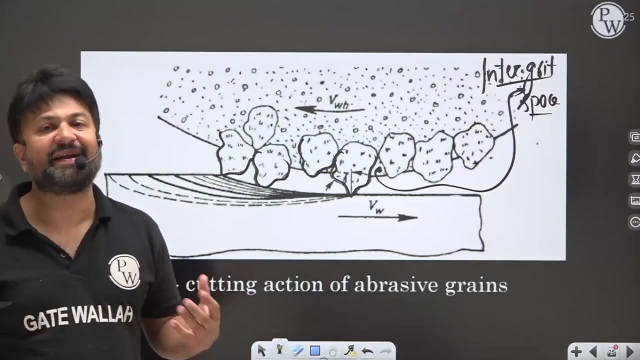 My dear. you have seen, you have seen that. you have seen this wheel: porosity, basically intra-grid space, intra-grid space. if the intra-grid space is large, then the wheel is, then the wheel is what you can say: open density, okay, the open, basically intra-grid. 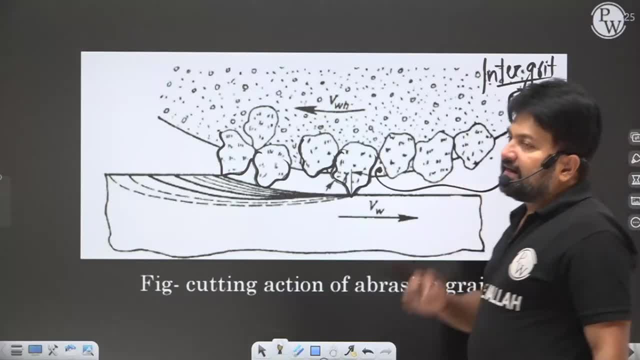 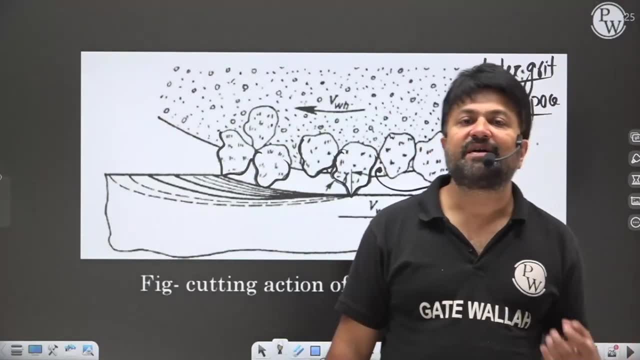 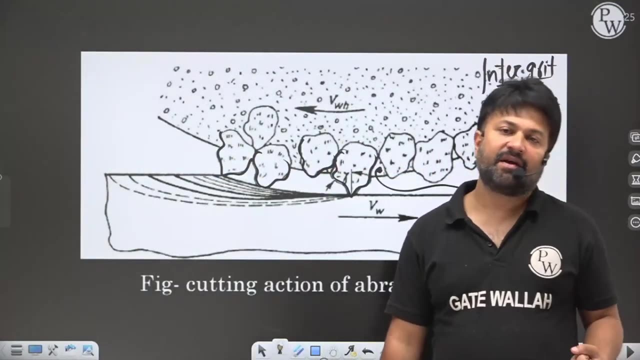 space is high, then then its density is low. if the intra-grid space is low, okay, or the space in between the grid is low, then the wheel is known as what dense, generally in the fine. If you use a fine grid, then the intra-grid space is what less. in that case, the wheel 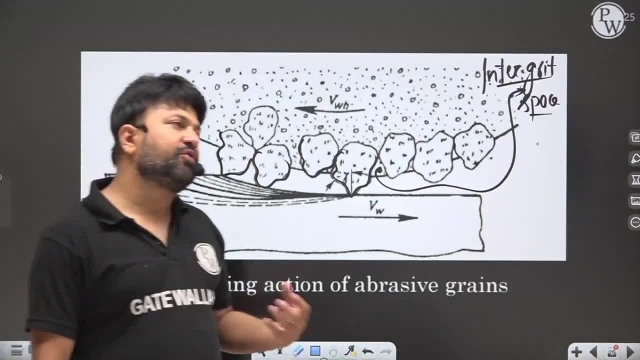 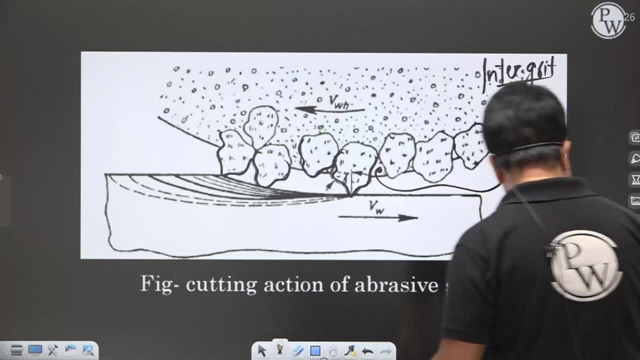 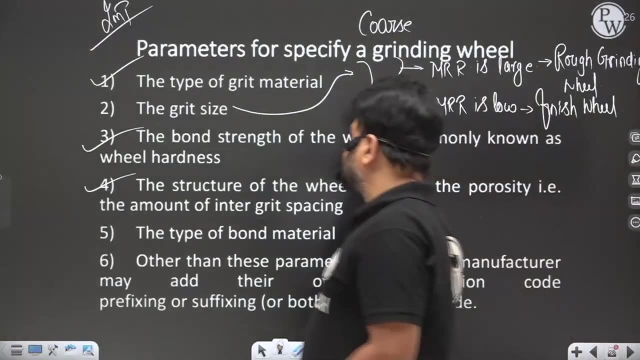 is what less. but if you use a, if you use a chorus grid, then the intra-grid space is high. then the wheel is what open structure? the wheel is known as what open structure, otherwise it is dense structure. if the space is what, very fine. if the space is what? 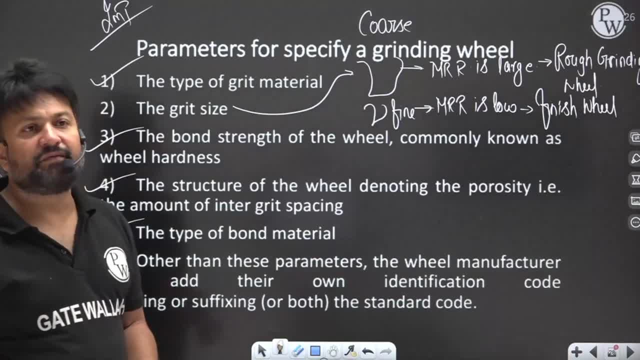 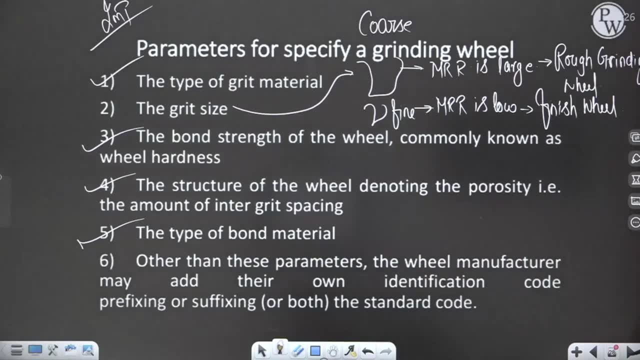 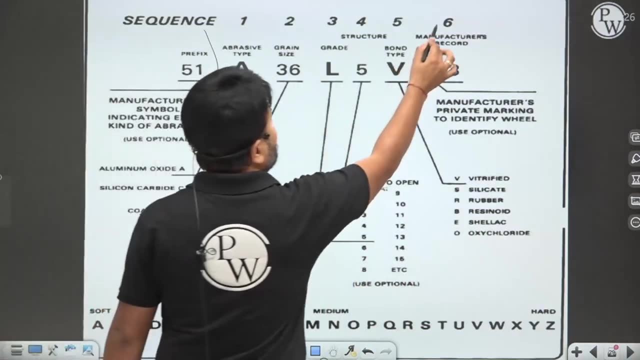 very less. Fifth is the type of bonding material which you are using. Suffix and prefix. Suffix we use to define the lots, the lot of the wheel in which, in which they are going to be manufactured. My dear student here, this prefix and suffix is not useful for us. what I told you first, 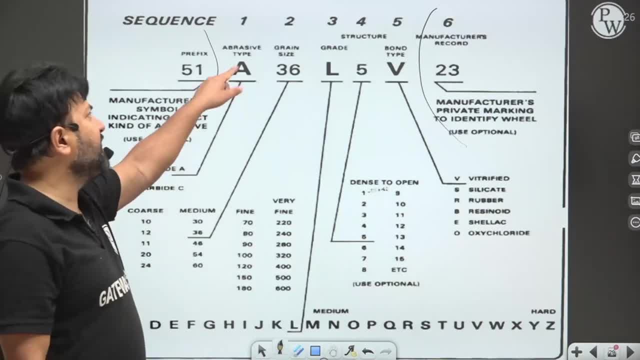 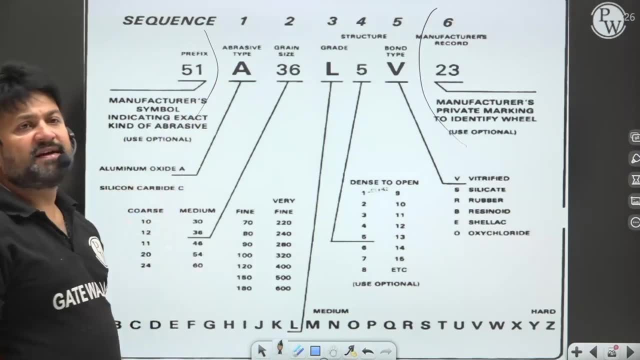 parameter told you the type of abrasive particle. A abrasive particle, that is the aluminium oxide instead of A. suppose that if C is written, then we are using silicon carbide as a abrasive particle? Let me find that out. So what I have written is C. this is the number. okay, this is the number. C size is: 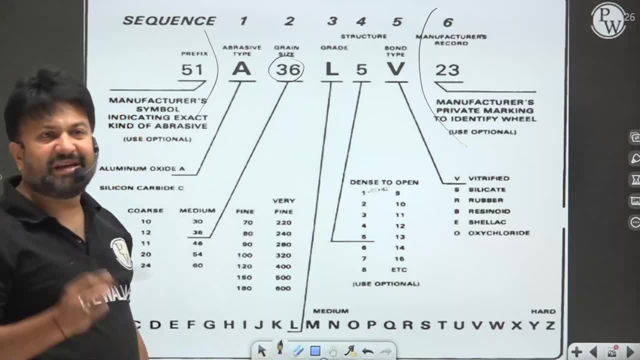 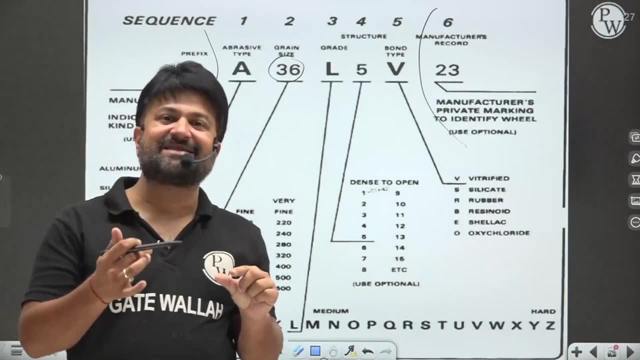 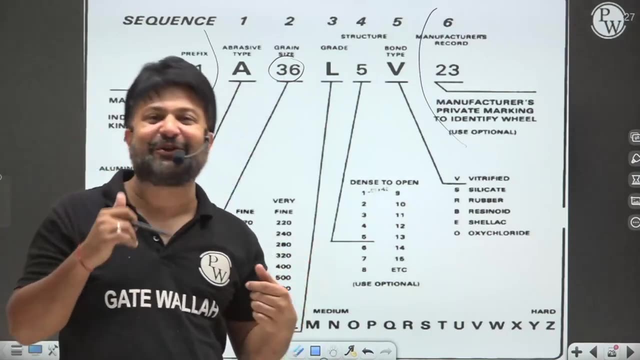 the number of the. so this is the number of the material. C size is the size of the material and this is the number of the material. So you do not want to write that as C, but you have to write it as C size. 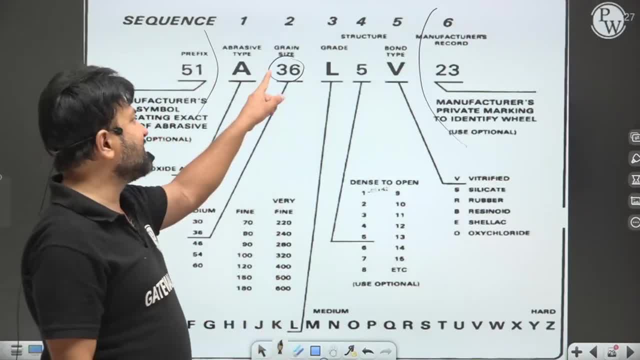 You have to write it as C size, So I am going to write it as C size. Let me write it again: Grid become finer. If this size is going to be reduces, if this number is going to be reduces, then grid become. 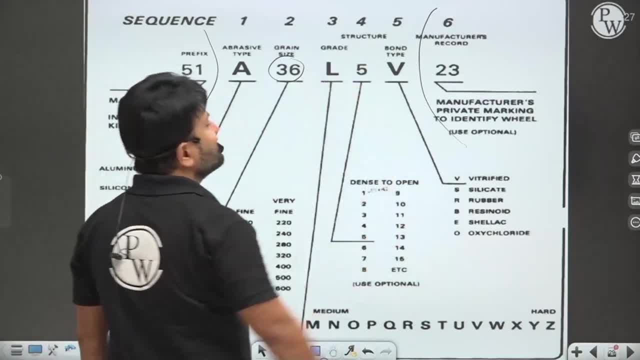 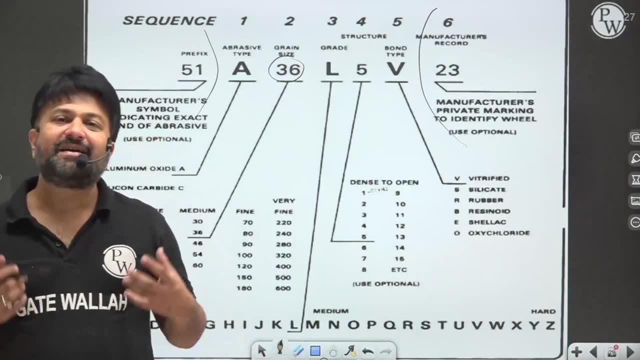 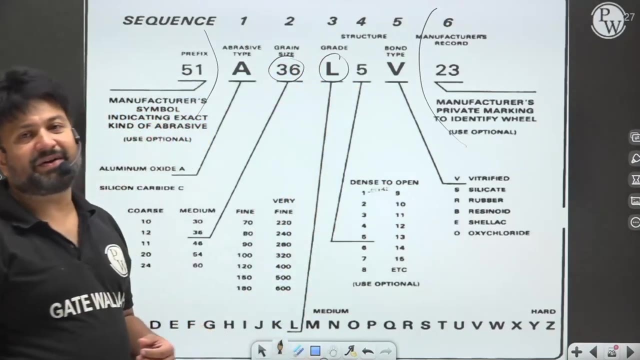 chorus. Now at the third position, what is that Grid? That is wheel hardness. Wheel hardness tells that the bond strength of the wheel. Okay, How much tightly abrasive particle are hold in the grinding wheel Right. So that letter will tell us about the hardness. 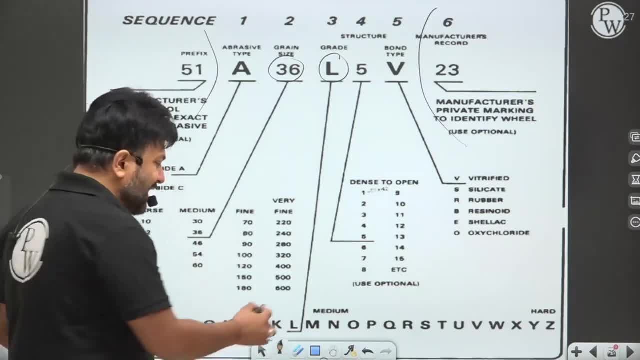 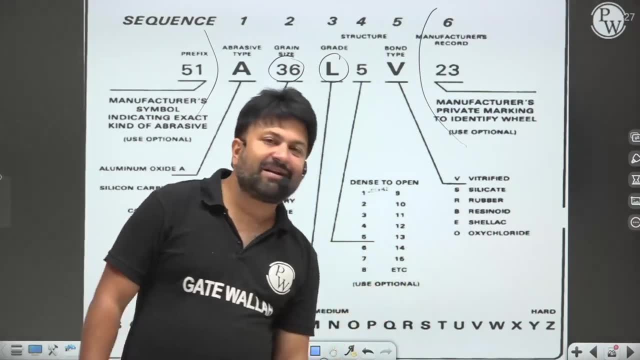 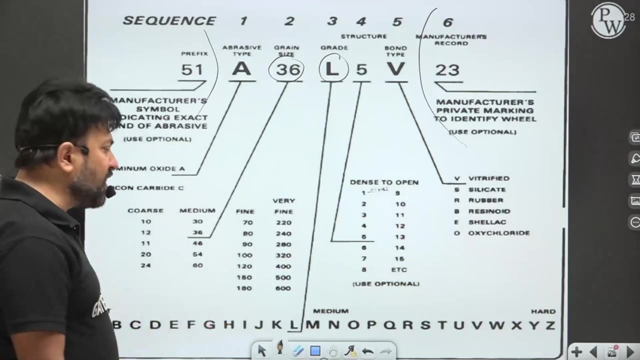 If the letter below L, then the wheel is what Low? If the letter is crosses the L, or if the any letter will find, okay, that side of the L, then the wheel become what? Hard. Or you can simply say: if you go from L to A, then the wheel become soft. 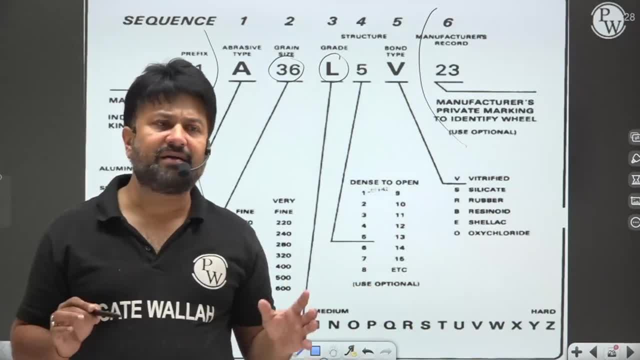 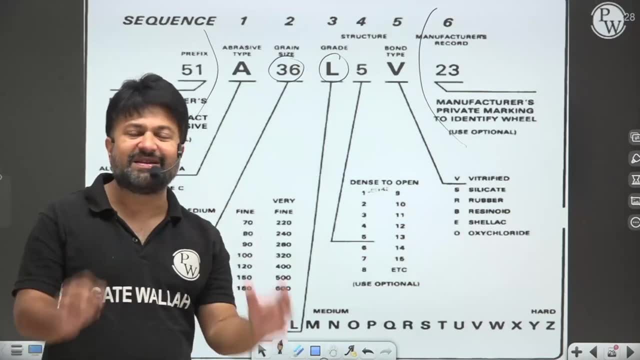 If you go from L to Z, then the wheel become hard. Right, The next parameter will tell you the structure of the wheel. Okay, Structure of the wheel. that is what That is: porosity. Porosity: the amount of intricate space. 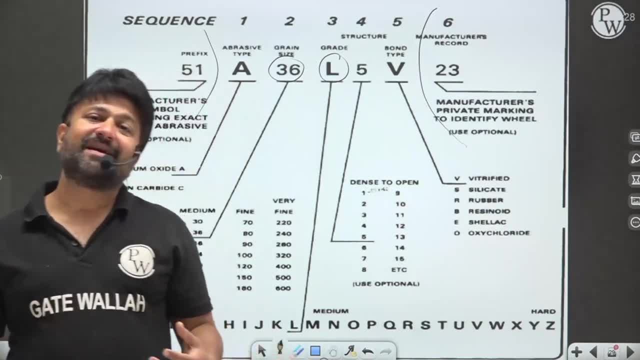 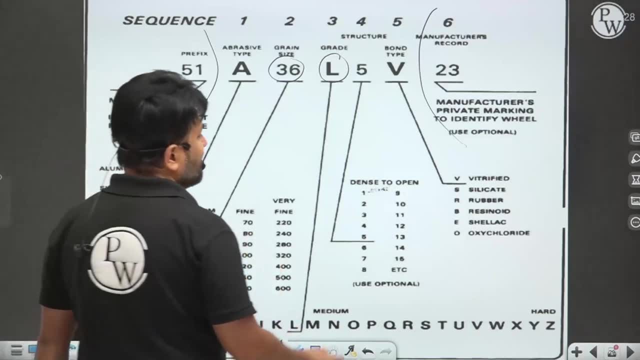 Okay, If the amount of intricate space is high, then it is open structure. If the amount of intricate space is less, that is it is a dense structure. So here: number the number is going to, when the number is going to increase. let us say: 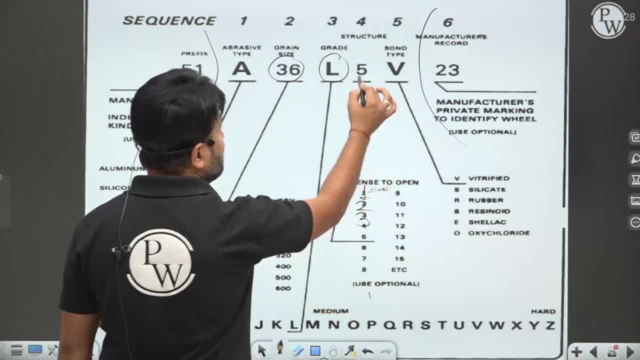 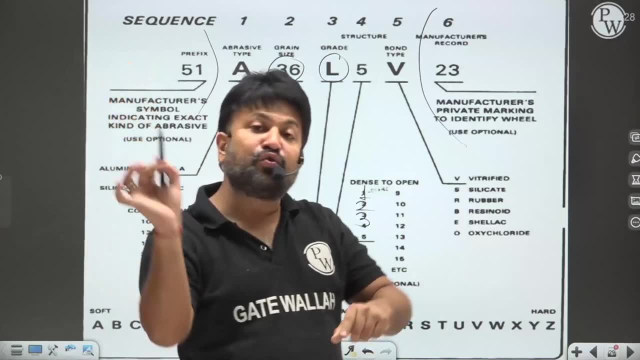 1,, 2,, 3,, 4,, 5,, 6,, 7,, 8,, 9,, 10, then it is going to open. It is going to open When the number is going to decrease. then it is going to dense. 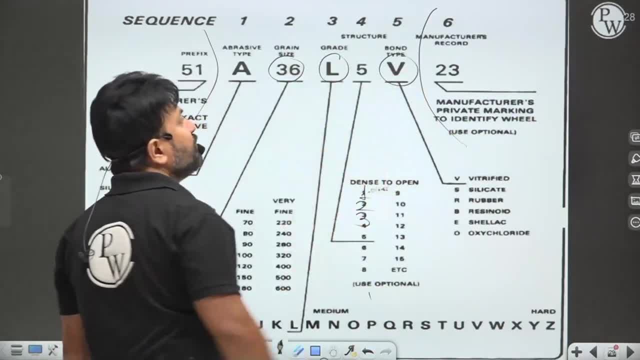 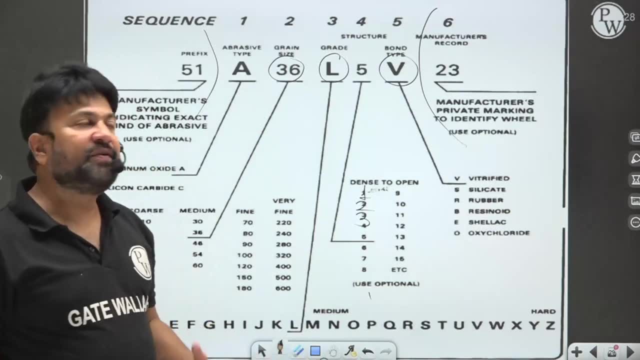 Right Now. the last parameter will going to tell you the type of bond which you are going to use to hold the abrasive particle. V stand for vitrified Right. V stand for vitrified Instead of V. suppose that if S is written, then S means silicate bond we are using. 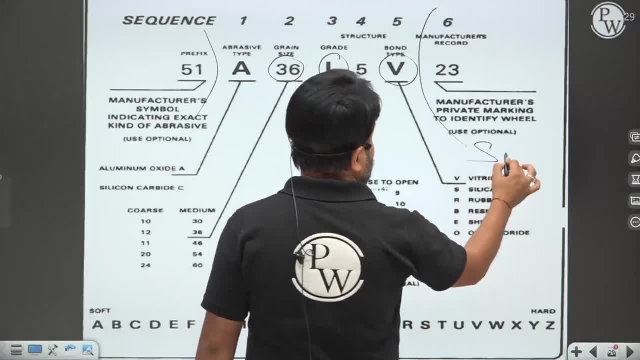 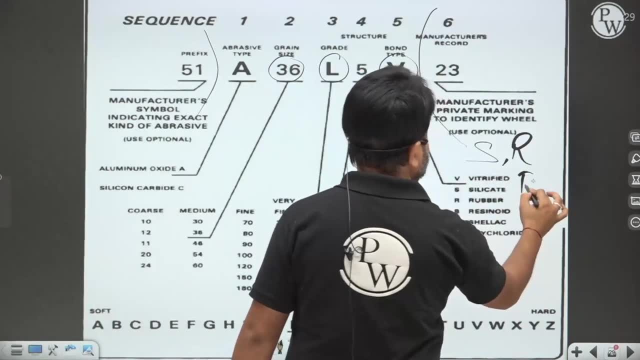 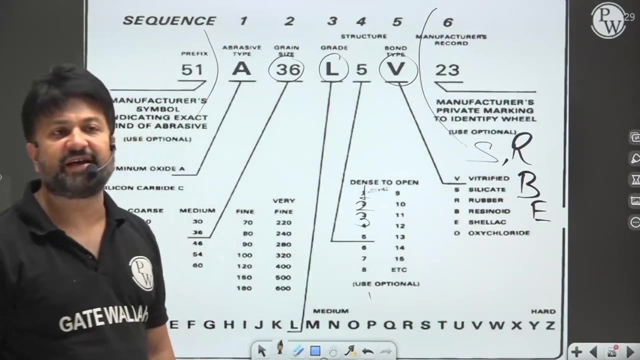 Instead of S. suppose that. suppose that if R is written here, then the rubber type of bond we are using here Instead of. if here B is written, then resinoid bond we are using Here instead of B. if E is written, then shellac bond is shellac material as a bond. 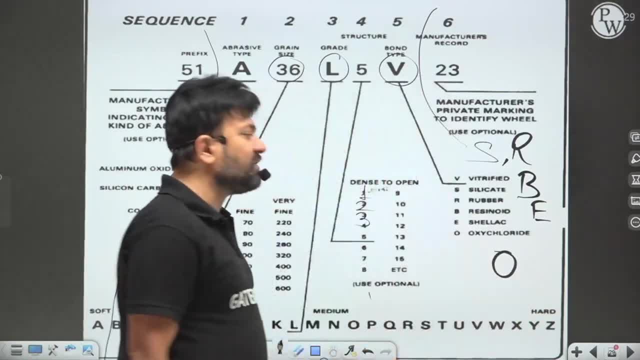 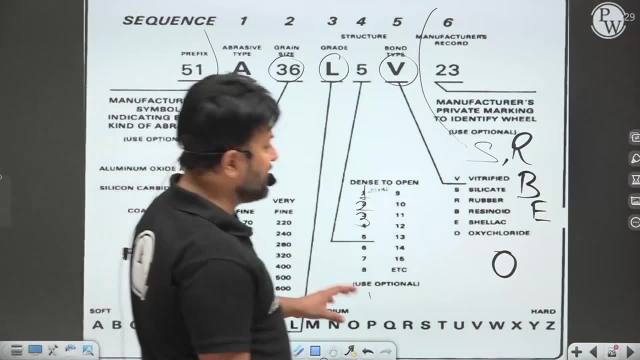 shellac bonding material is using here. If O is written, then oxychloride is using as a bonding material, Right, As a bonding material. So this is a very important slide. Please remember this slide Right Now. what is a centerless grinding? 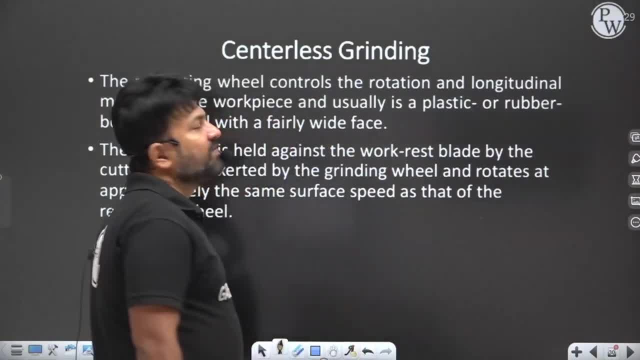 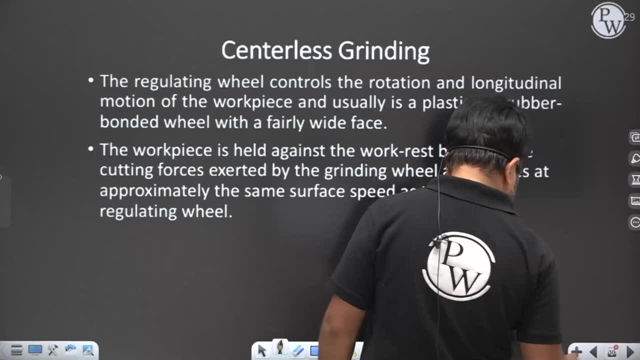 My dear, centerless grinding is a process where we are not going to mount the wheel. We are not going to mount, We are not going to mount a wheel Right. Basically, what is going to happen in a centerless grinding. Let me show you. 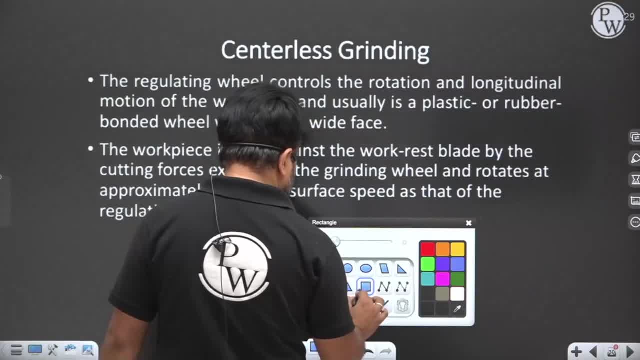 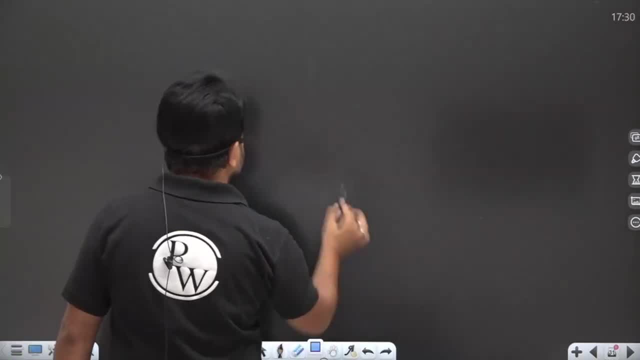 In a centerless grinding. there is a wheel. Okay, There is a wheel. Let me show you. There is a wheel. This is a. this is a first wheel. Okay, This is a first wheel. Right, This is a first wheel. 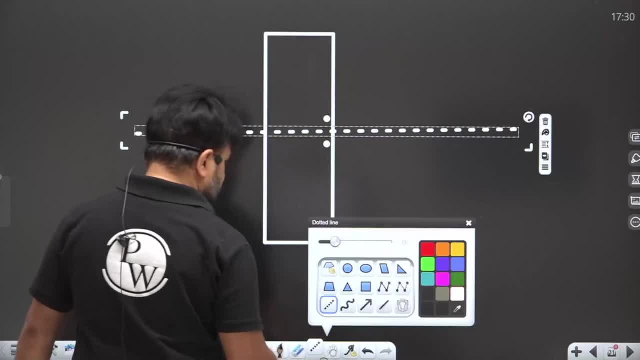 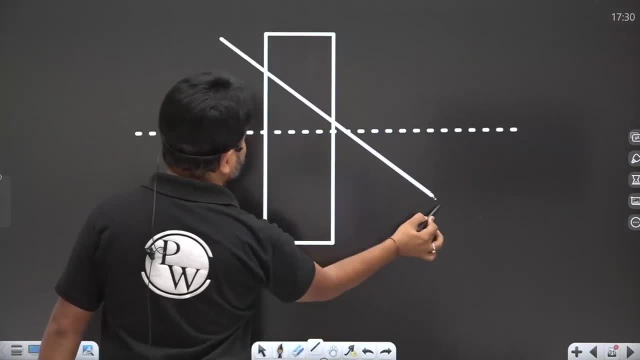 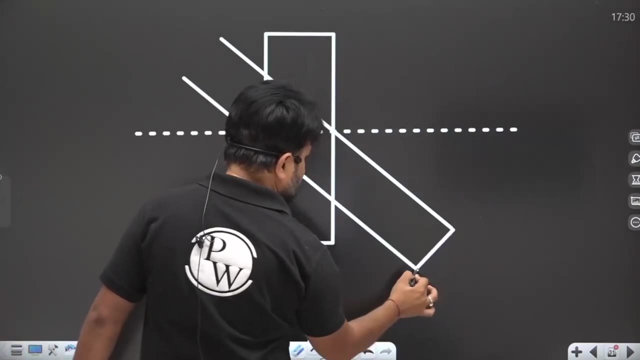 Let's say, this is an axis of rotation. There is a another wheel which is little bit inclined. Okay, Which is Little bit inclined, Which is little bit inclined. Let's see, See here, Which is little bit inclined. 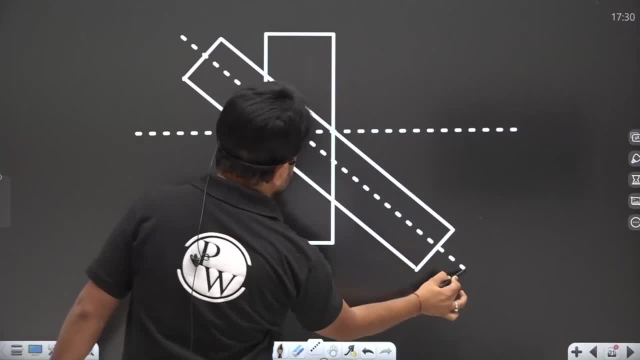 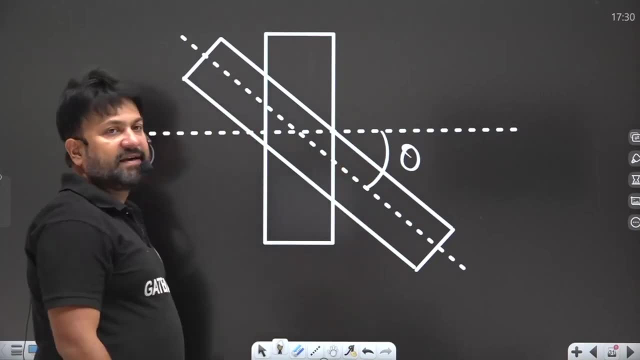 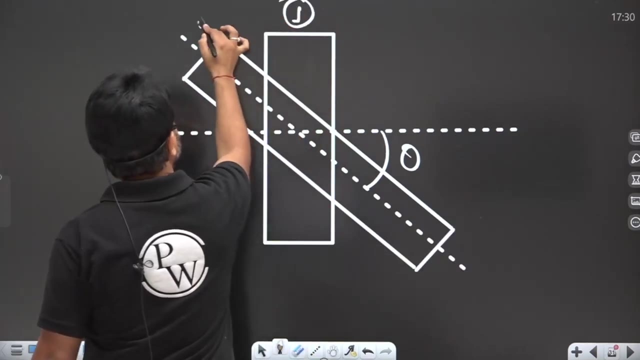 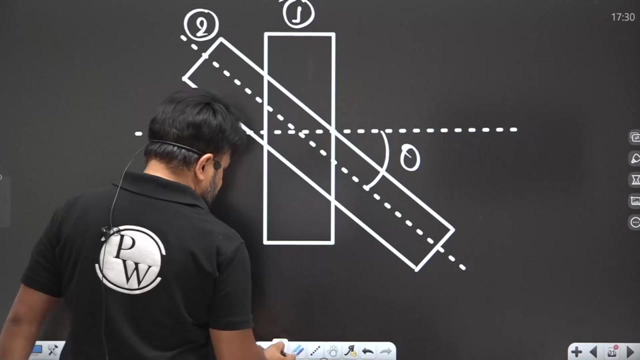 Right, Which is little bit inclined, See, Which is little bit inclined. Which is little bit inclined, Centerless grinding. Okay, Now, this is grinding wheel one, This is grinding wheel one, And this is grinding wheel too, if you see from that side, if you see from that side or that side the wheel. 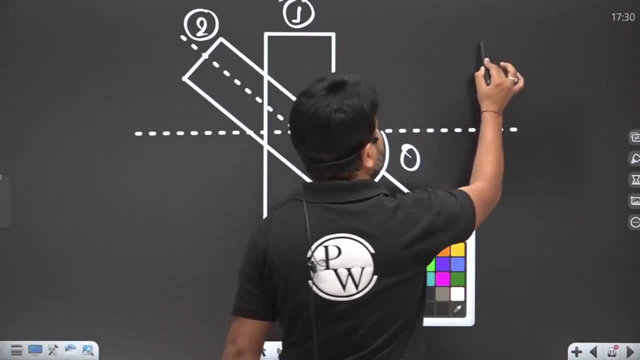 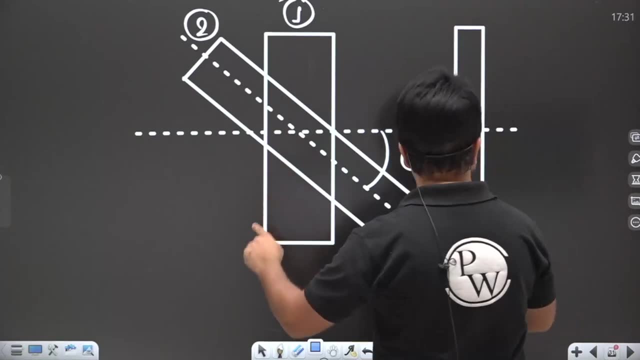 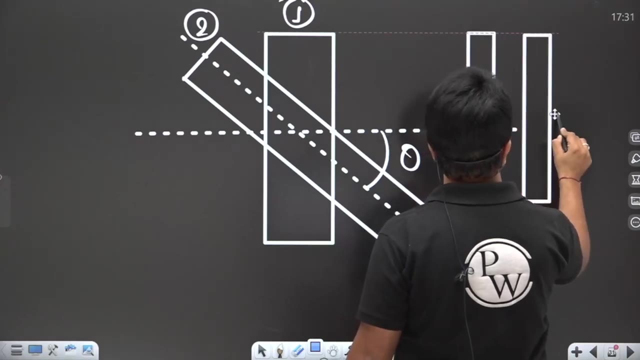 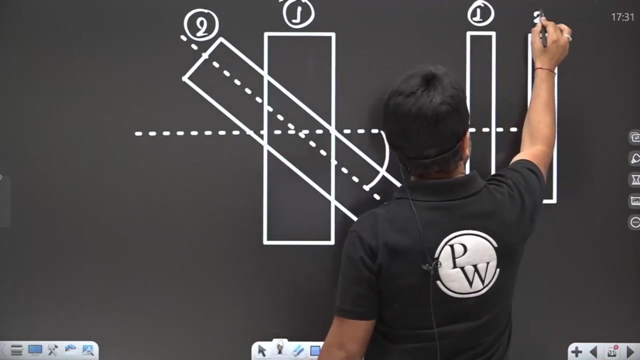 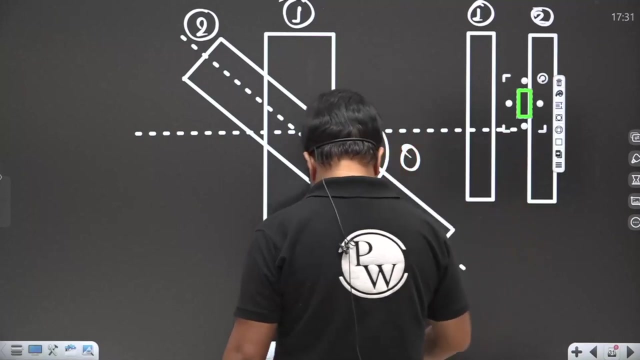 will be look like this. the wheel will be basically look like this. let me tell you, let me show you, let me show you. this will see, this will right. another wheel, this wheel number one, wheel number two, right in between. a workpiece comes here in between, a workpiece will comes here in between, a workpiece will come here, right, which is placed. 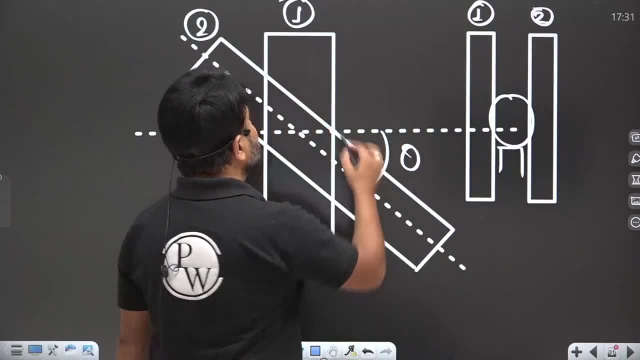 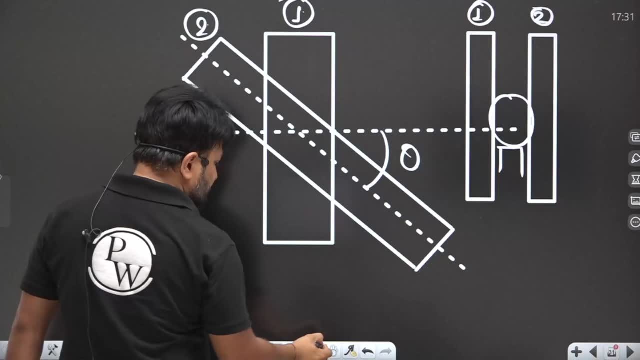 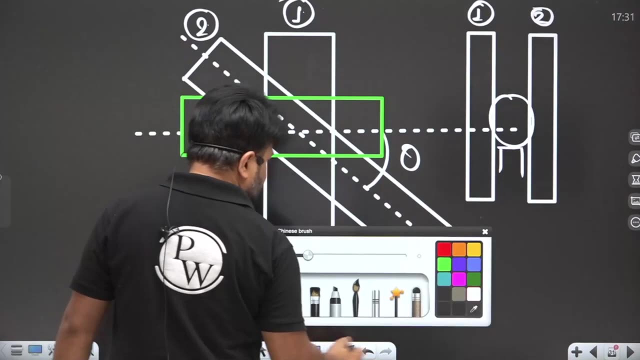 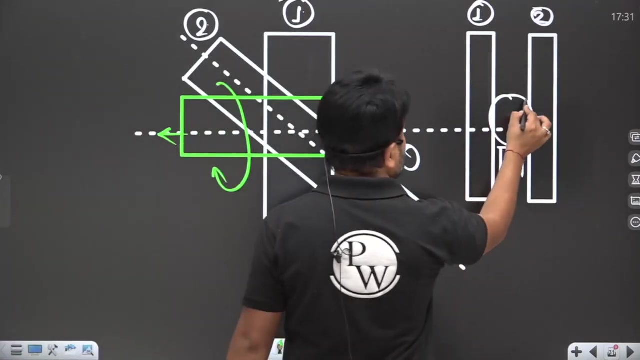 at the rest blade. now what is going to happen? this grinding wheel is going to be what rotate because of the inclination between the wheel. whatever with the workpiece might hear, whatever with the workpiece, this will rotate, this will watch rotate, this little rotate and move on. linear motion- right, this word. 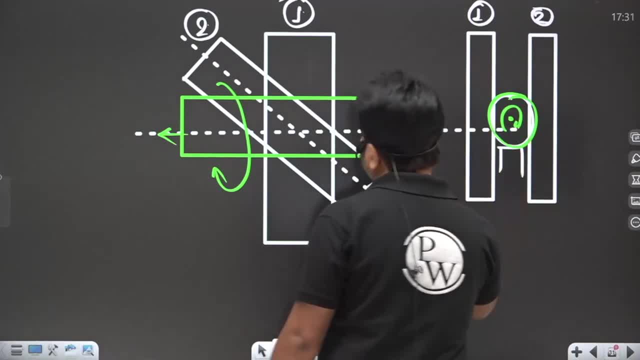 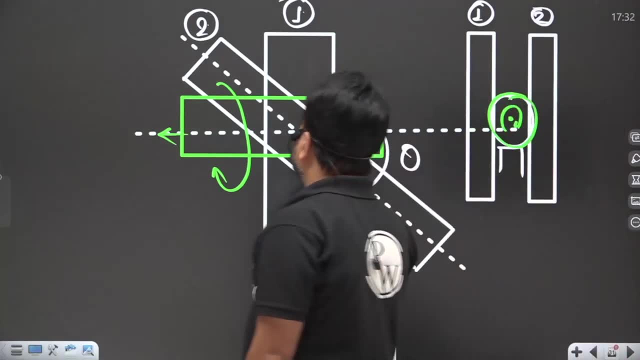 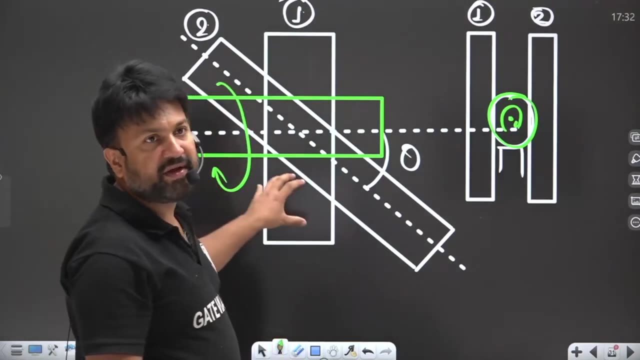 peace will rotate, ok, and muss paint linear motion, right, that is what you are as central as grinding, right, that is what your central as grinding. yet the work is not going to be a key here. the word is not going to be what here? the work piece is not going to be mount anywhere, ok, 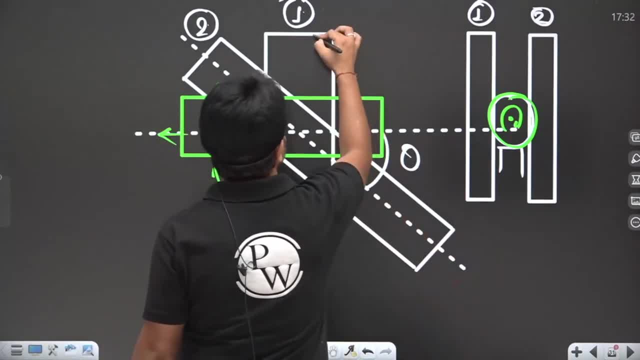 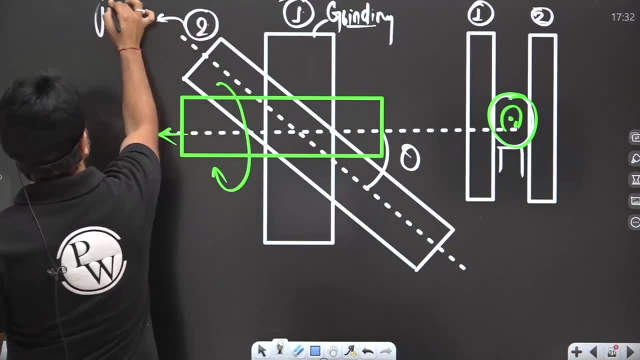 One of them here, wheel number 1, basically a grinding wheel. this is a grinding wheel, right, this is a grinding wheel. one of them is a grinding wheel and it is a regulating wheel. regulating wheel. regulating wheel- right regulating wheel.